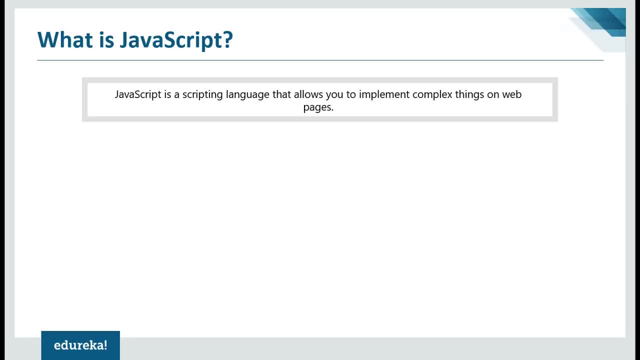 first of all, let me tell you that JavaScript is not related to Java at all. In fact, it has nothing to do with Java. Then why was it named JavaScript? Well, it was sort of a marketing strategy, And when JavaScript was first released, it was called Mocha. Then 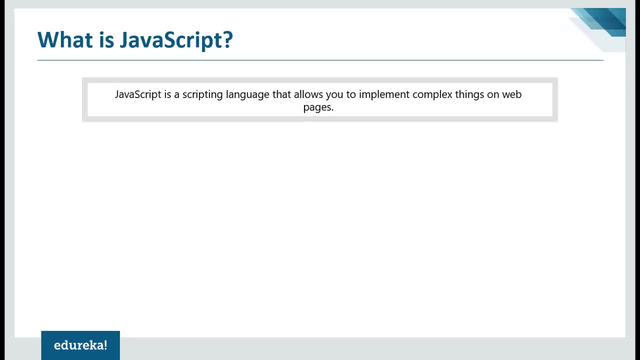 later on it was renamed to LiveScript and then to JavaScript. Now let's not get into the details of this Now. in simple words, JavaScript is a language of the web. So basically, every browser, every PC, every mobile understands JavaScript. It's like a universal language. 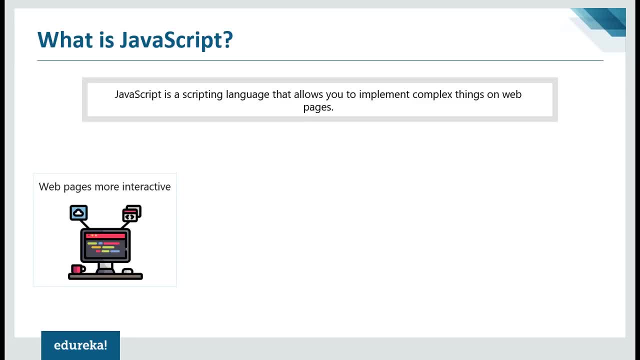 Now, what is JavaScript used for? JavaScript can be used to make web pages look more interactive, more attractive and more appealing. Apart from that, another key feature of JavaScript is that it is an interpreted language Now most of the popular programming languages. 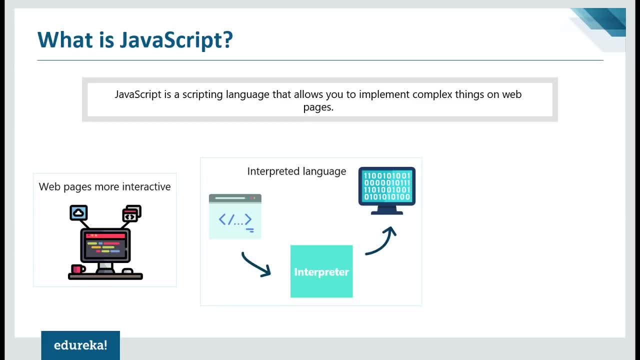 like C and C++, require a compiler, But when it comes to JavaScript, you do not require to compile the script. okay, So most of the browsers like there is Google Chrome, there's Internet Explorer- Most of these browsers have a JavaScript engine embedded into them. okay, So every. 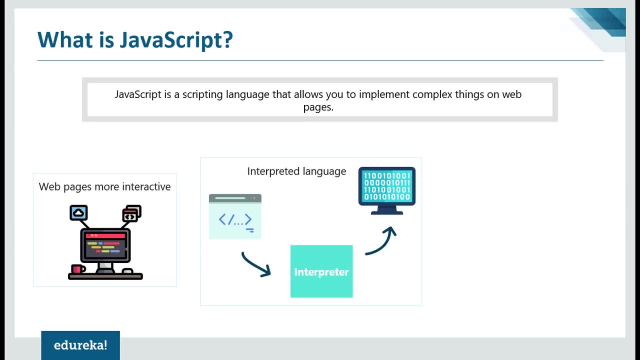 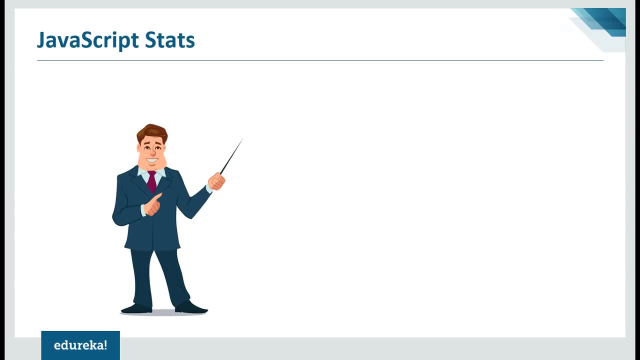 time you run a JavaScript code, it will automatically be converted into machine code by the web browser's engine itself. okay, Then another key feature is that it runs on the client's computer. okay, So it's a client-side scripting language. So, guys, I hope all of you are clear with what. 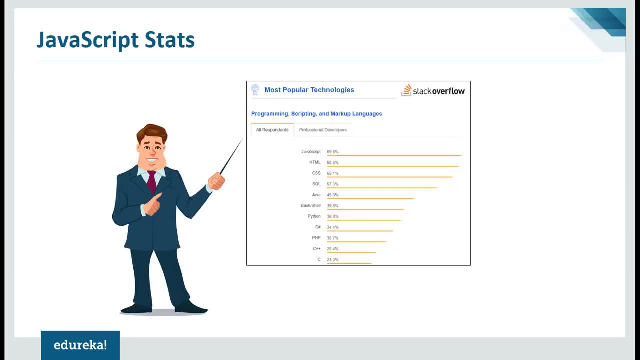 JavaScript is. Now we're moving on, So we all know that there are hundreds of programming languages, and new languages are being created every single day. Among these, there are very few powerful programming languages that bring about big changes in the market And JavaScript. 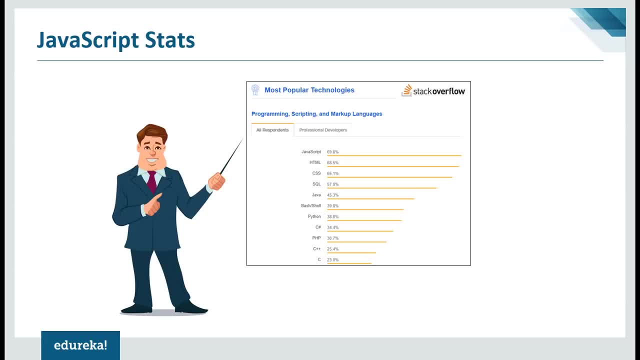 is definitely one of those languages Now. JavaScript has always been in the list of the most popular programming languages. Now, in this picture you can see that this was a recent survey from Stack Overflow, which showed that JavaScript is the most popular technology Now. it stayed in this number one position for six years in a row Now. 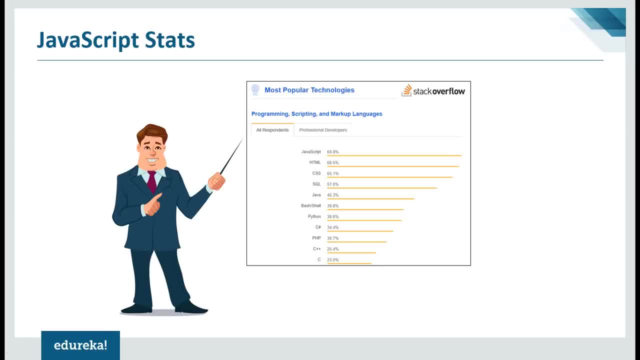 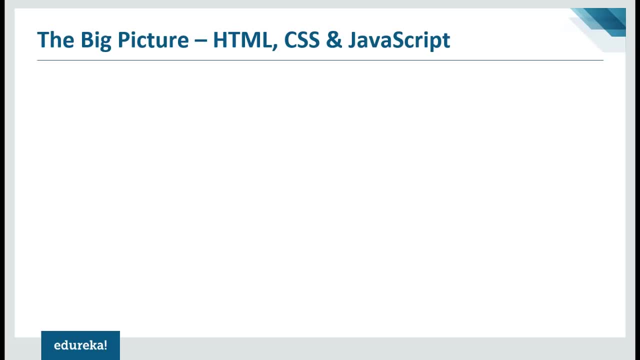 this means that it is a very effective language. A lot of developers are liking this language, okay. So, guys, I hope I'm audible. All right Now. anybody who's heard of JavaScript knows that JavaScript has something to do with HTML and CSS, So there is some sort of relationship. 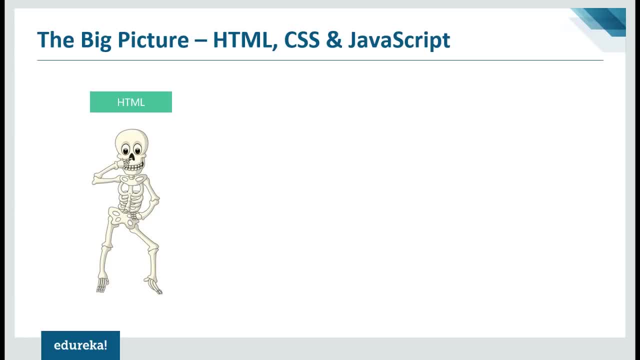 between these three. Now what is the relationship? Now, HTML is basically like the skeleton of the web page. It defines the structure of the web page. okay, HTML stands for hypertext markup language. Similarly, we have CSS, which stands for cascading style. 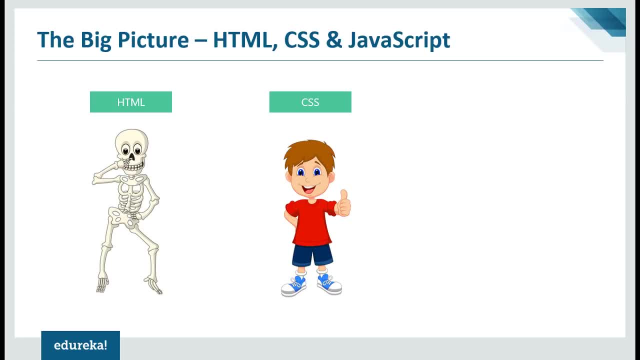 sheets. Now, CSS is like the clothes we put on to look more stylish and more appealing. Similarly, the web also looks more stylish by using CSS. okay, So any color or any pop that you see in a web page is because of CSS. Now, where does JavaScript fit in? So, basically, 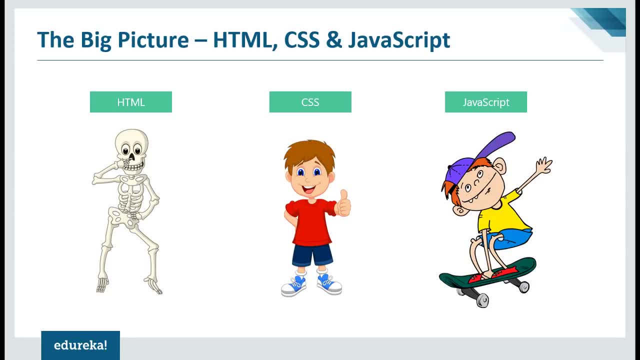 JavaScript is used whenever you see a page do something like this. So, basically, JavaScript is used whenever you see a page do something like this. So, basically, JavaScript is used when something is using something or something like this in a web page. So you can see that. 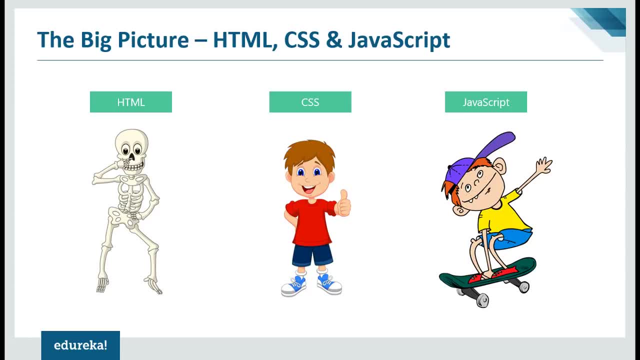 it's doing more than just sitting there and gawking at you. That's when JavaScript is used. So it is used whenever you want to implement some motion into the web page. So if you see anything moving on a web page or any sort of dynamic moment on a web page, it's because 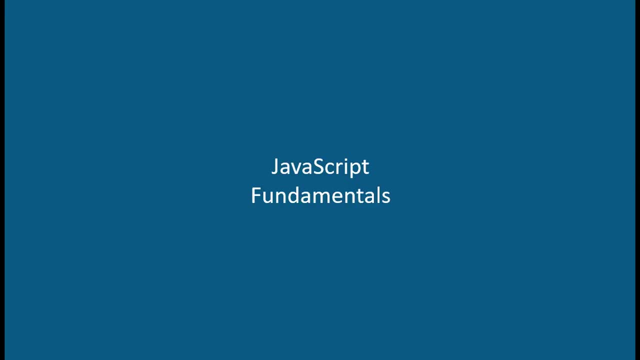 JavaScript is involved, okay. So, guys, now that you have a good idea about what JavaScript is and how it works, let's get on with the coding part. okay, So I'm going to cover a few basic programming concepts of JavaScript, And these concepts. 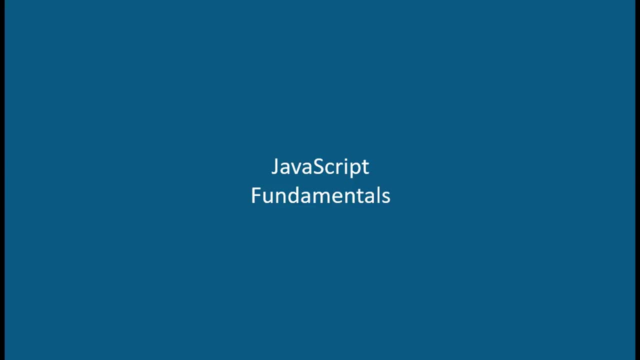 are quite similar to the ones we talked about, right? So we have the basic programming concepts, the c language and c++ language. okay, so anybody who's familiar with these c and c++ languages will easily be able to relate to this. okay, now, first we're going to see what are variables. 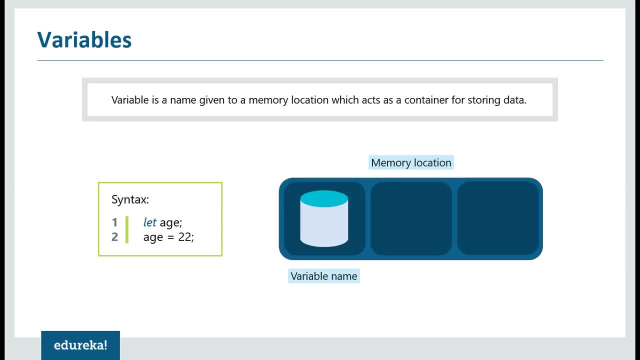 now, variable is basically a name that is given to a memory location and within this variable you can store a value. so let's say, i declare a variable called age and i'm going to store a value in it which is 22. okay, so this is what variables are, now what i'm going to do. 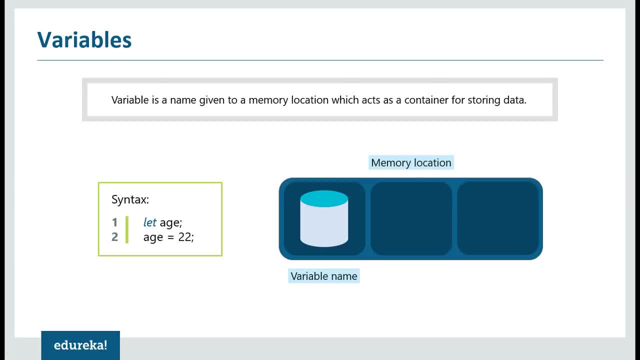 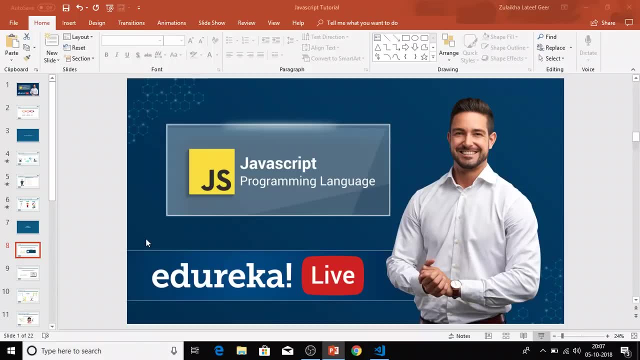 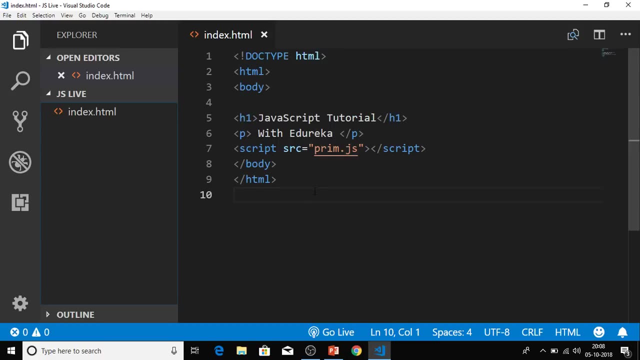 is, i'm going to open up a javascript editor and i'm going to show you how to declare variables and we'll see how to run codes using this editor. okay, so this is my visual studio code. um, so what i've done here is i have a simple html file and in this html file, 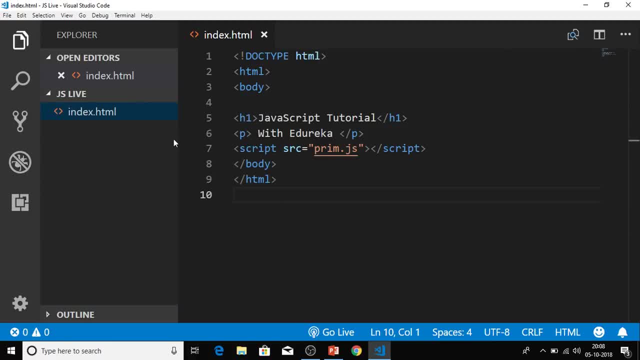 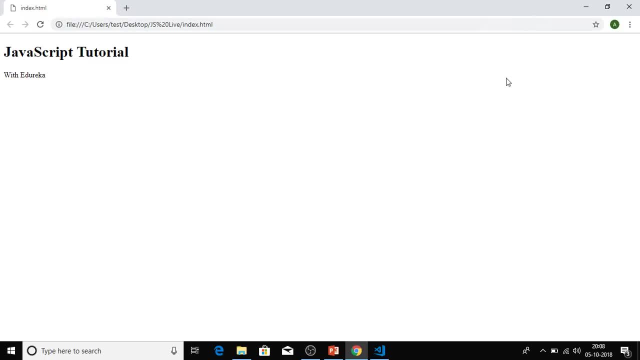 i've just defined a simple web page. let me show you how this web page looks. okay, it's simple. it's like this javascript tutorial with edureka. okay now, um, what we can do is if you right click on any web browser, like if you right click on google, chrome or even internet explorer- you can see this inspect here. 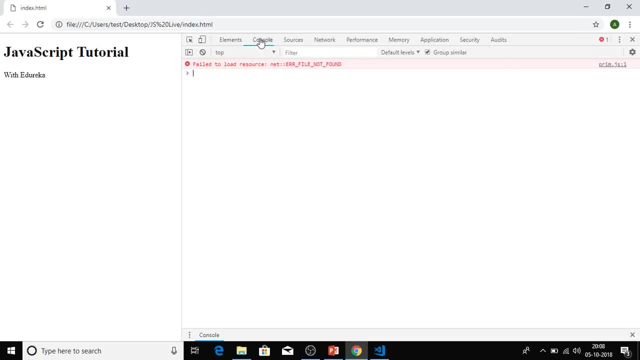 so what you do is click on inspect and you go to console. now, um, uh, if you try to log anything on this console, let's say you try to print hello world or something like that- let's try that. okay, when you do this it will print hello world onto the screen, okay. so basically, all these engines, all these browsers, have a. 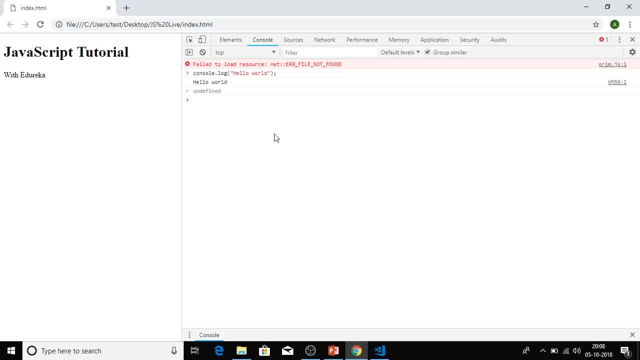 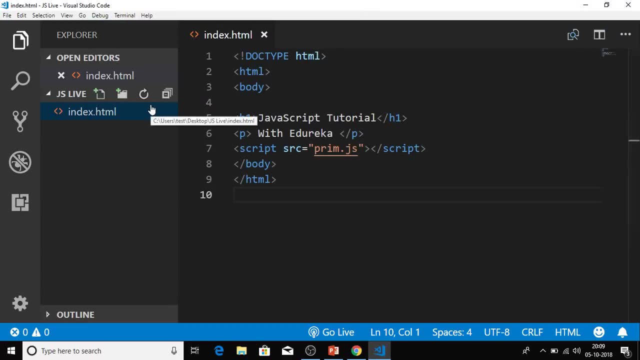 javascript engine embedded into them. okay, so you can run javascript code even in your browser. okay, now going back to our file over here. now there are two ways in which you can define your javascript code within this html file. now, every time a web page runs, the html file is basically: 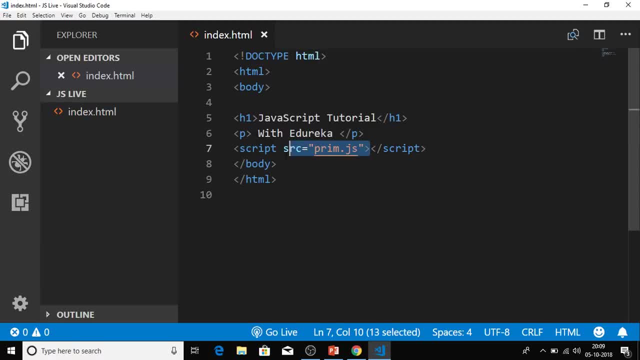 running. okay now there are two ways in which you can write your javascript code now. the first way is to define these script tags all right now. within these script tags, you can type your entire javascript code. so if i type console, log, and if i log, hello to the terminal. 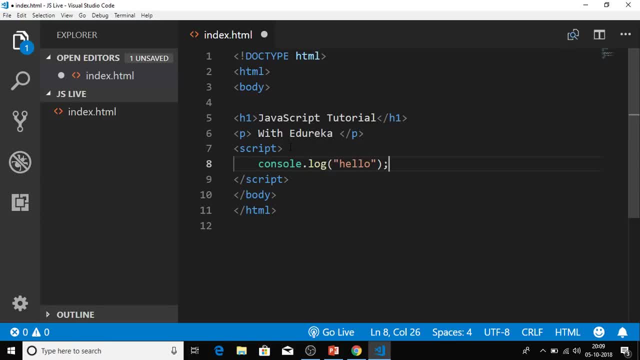 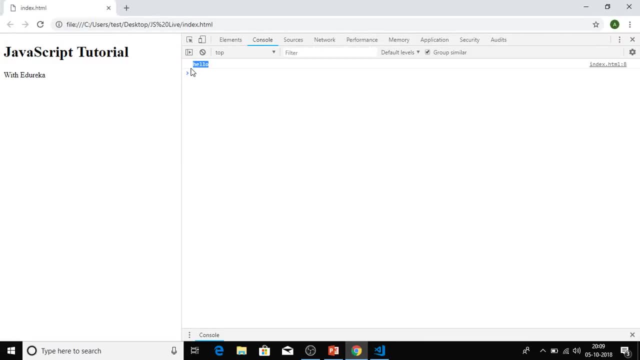 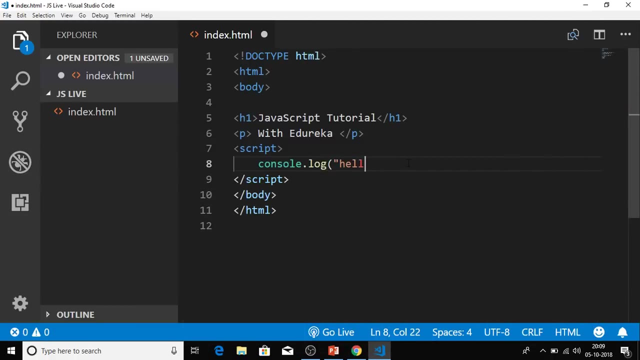 it should work okay. so i'm going to save the changes and let's refresh the browser. yeah, here you can see that it printed. hello, okay, now. this is the first way of writing your javascript. now, another way is what we are going to follow in this session today. now the reason why we don't go with typing your entire javascript. 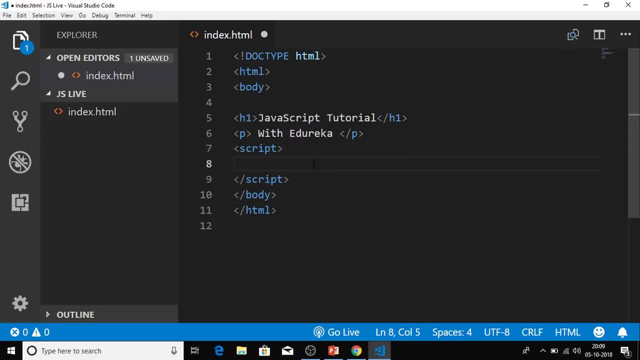 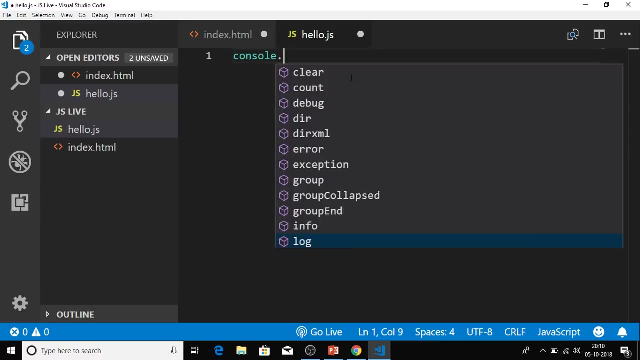 code here is because it's not practical. you can't type thousands of lines of code on your html file, so what we can do is we can type: let's create a new file first. we'll name it hellojs. okay, now in this file i'm going to log hello. 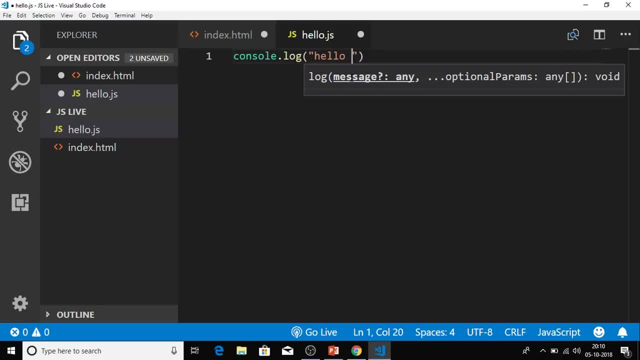 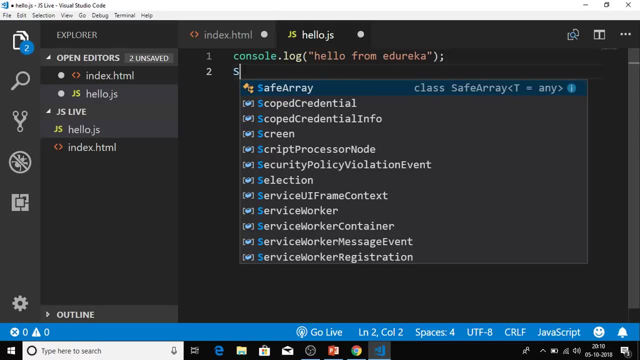 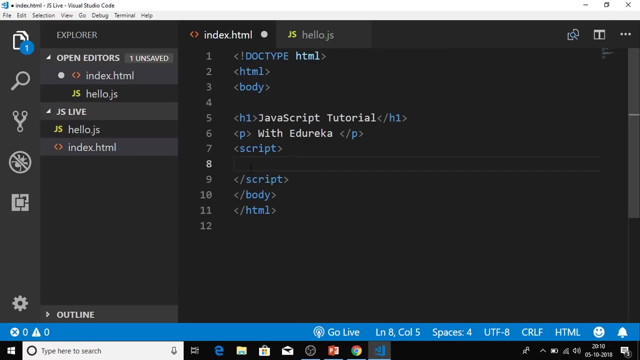 world. okay, i'll log hello world or hello from edureka. okay, i'm going to save this file and i'm just going to one second. yeah, so i'm saving the file and i'm just going to link this file in my html file. okay, so how you do that is you're going to define an attribute called src and you're going. 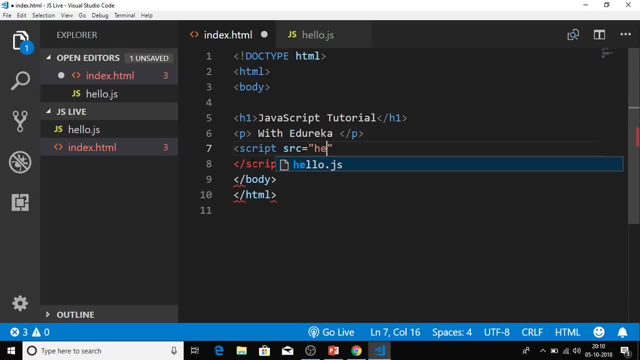 to set this attribute to hellojs. so what you're doing is: you're just referencing your hellojs, which is a javascript file, from your html file. okay, now close the tag and yeah, so this is the second way of defining a defining javascript. now what you can do is: 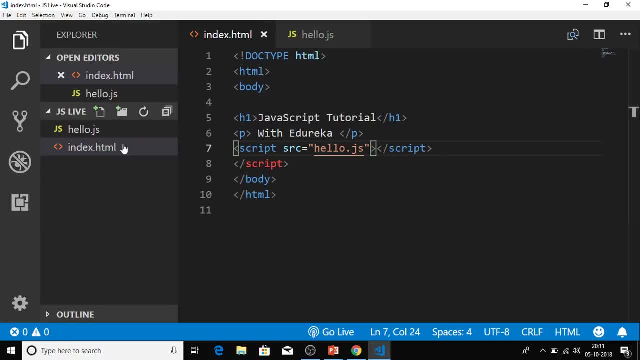 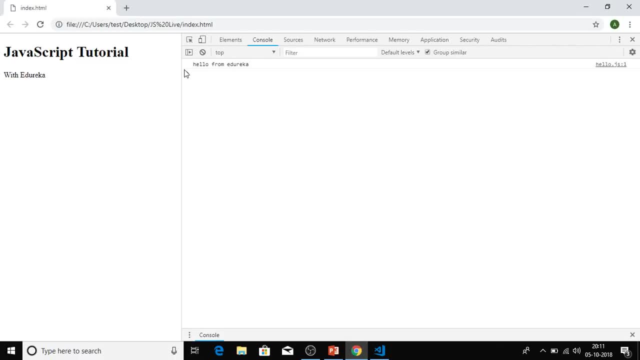 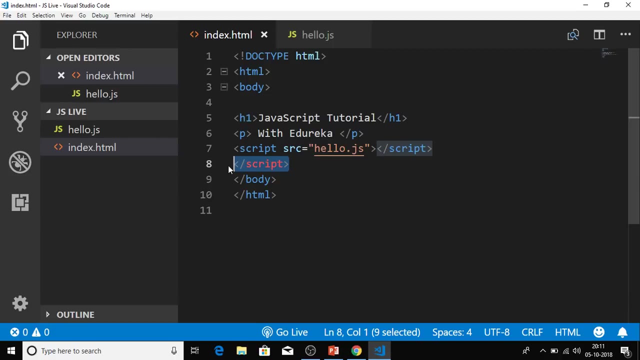 save this and open up your browser. it should print: hello world, hello from edureka. yeah, so you can see that it's printed: hello from edureka, all right. so these are the two ways of defining your javascript. now let's get started with variables. okay, now let's create a new file over here and i'm going to name it variables. 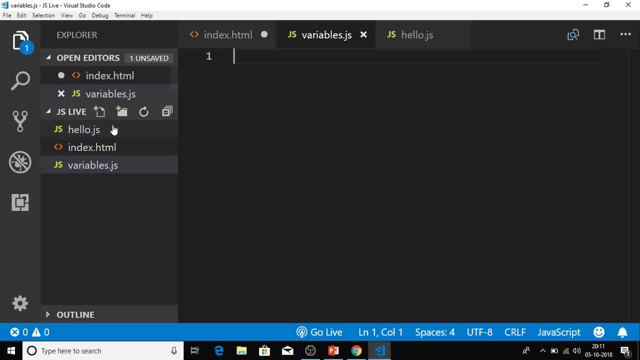 all, right, now i'm going to define a variable. in order to define a variable or declare a variable, you need to use the let keyword. okay, so let me define a variable called age and i'm going to set find a variable called age using the let keyword and i've set its value to 20.. okay, now let's try. 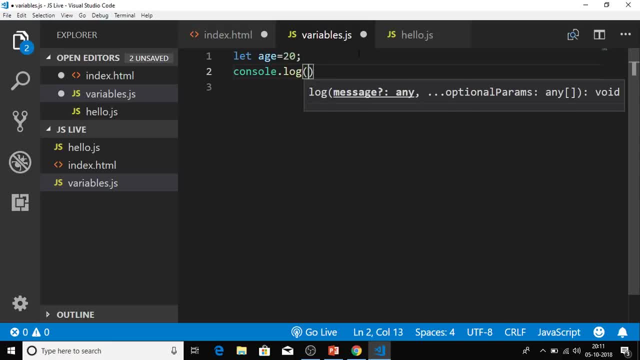 logging the value to the console. okay now, this function is as simple, is very simple. all you uh, what this function does is it's going to log whatever you type within these parentheses onto the console. okay, so let's just pass the value age. so we're just going to mention the. 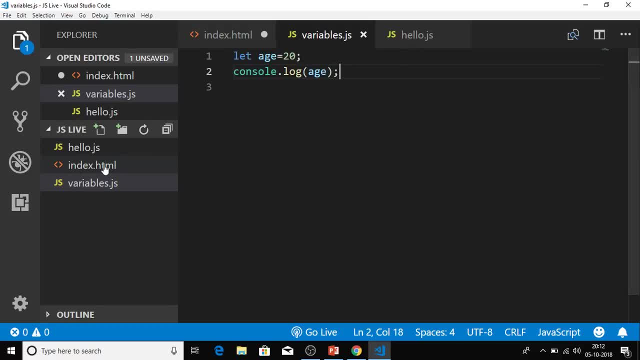 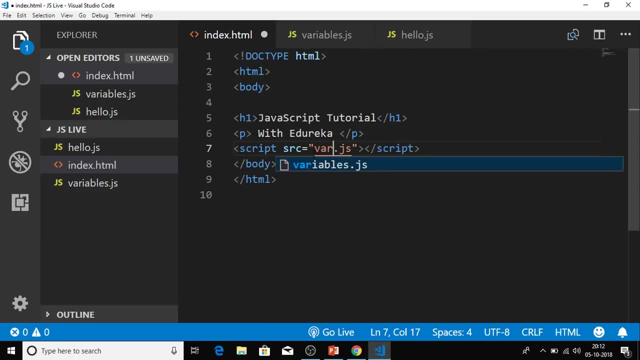 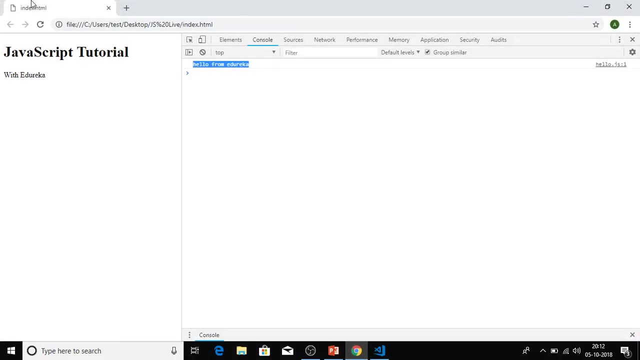 name of the variable. let's save this file. and we also have to link variablejs in our html file, okay, so i'm just going to change that over here, okay, and save your file. okay. now, when you refresh, you see the value of the variable, which is 20.. 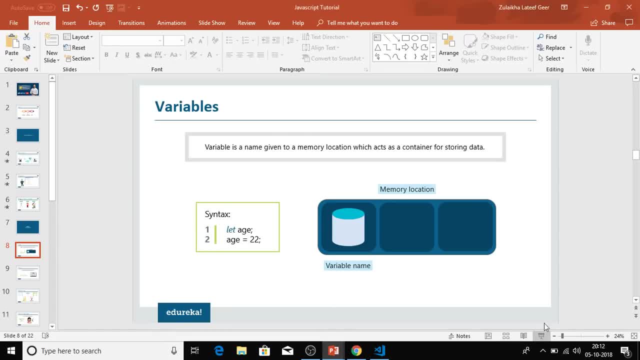 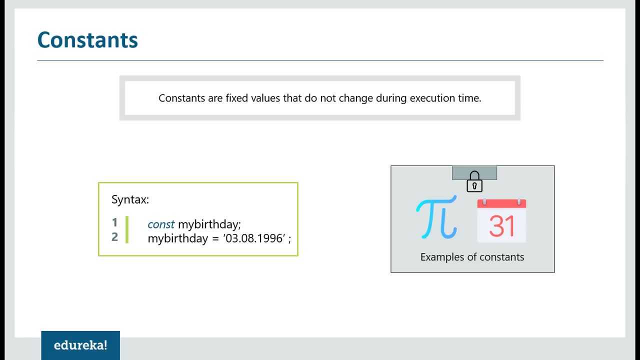 okay. so, guys, this was about variables. now let's look at constants now. uh, there are times when you don't want to use a variable in your javascript, but you can use the value of a variable to change because it might disrupt the whole workflow. now, in such situations, 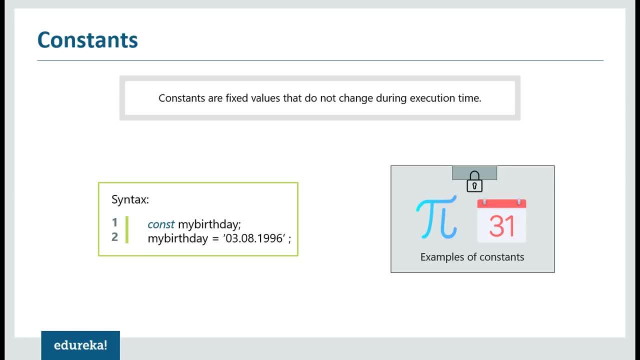 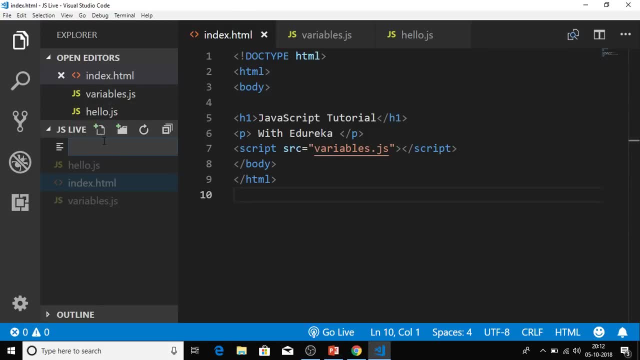 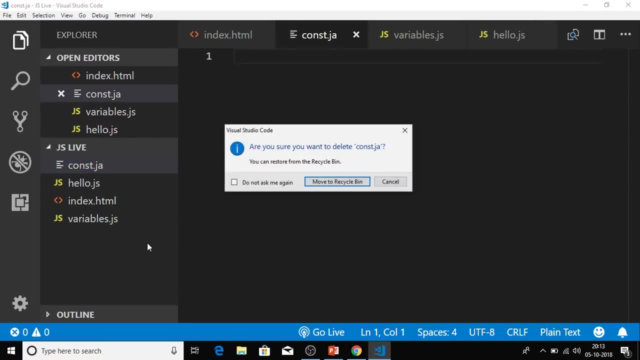 what you do is you make use of constants instead of variables. okay, now let's see how to do this, how to declare a constant on visual studio code. so i'm going to open a new file over here. i'll name it const dot js, and sorry, i named it wrong. okay, so i'm going to create a file. 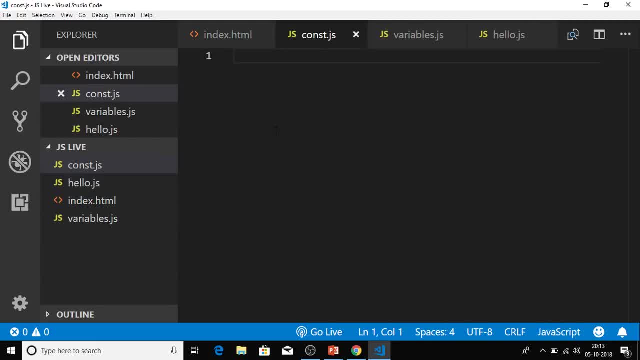 constjs. okay, now over here, let me show you how you declare a constant variable. so you use the keyword const. all right, const. and now let's declare a variable, say pi. now i'm going to set the value of pi to 3.14. okay, now let's log this to the console. 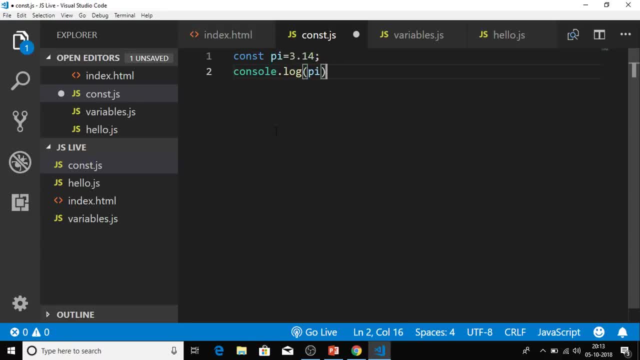 okay, now, before we do this, let's try to change the value of the constant variable. let's see what happens when you try to change the value of a constant variable. so i'm gonna set the value to 3.16. here i'd written 3.14 and now 3.16. okay, let's see what output we get. 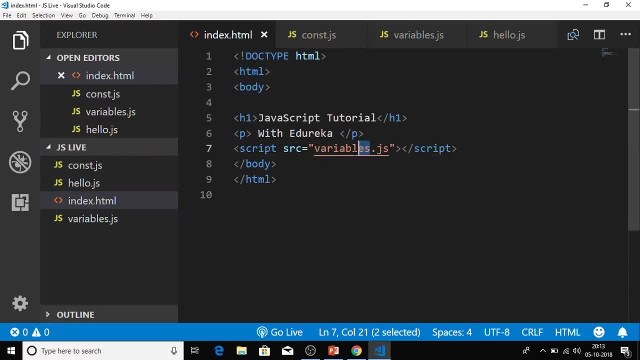 okay, guys. so also let's remember to change the link over here. yeah, now save this and open up your browser and refresh. yeah, here you can see that it's given an error. now this is because we tried to change the value of a constant variable. now you only define. 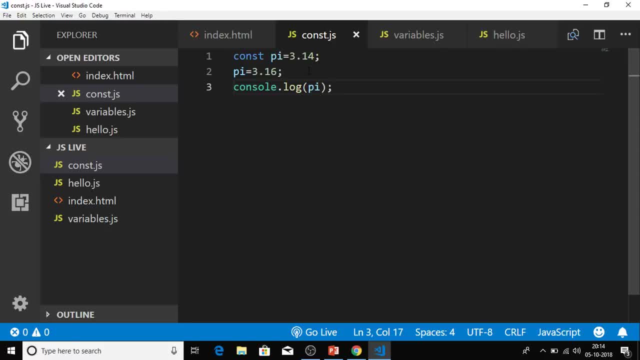 a constant variable. so you can see that it's given an error. now this is because we tried to change the value of a constant variable. now, you only define a constant variable when you want to have a fixed value throughout the program. okay, so this, this, uh, declaration that. 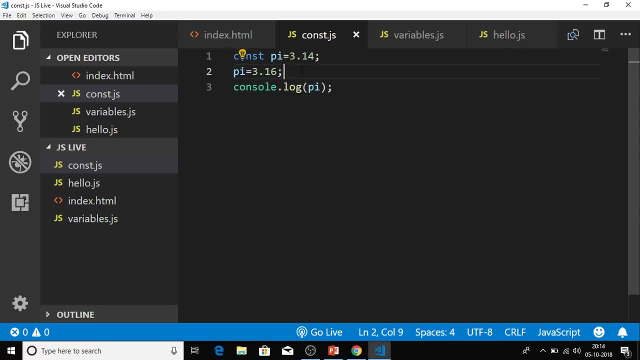 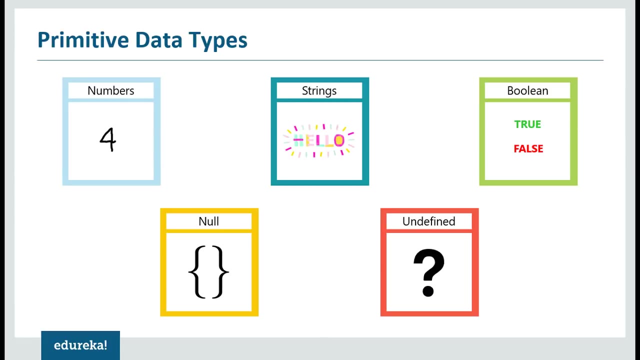 i did over here the value. i set it to 3.16 can't be done on a constant variable. okay. so, guys, that was about constants. let's move on to our next topic. okay now. the next topic is primitive data types. now, um, there are different types of values that. 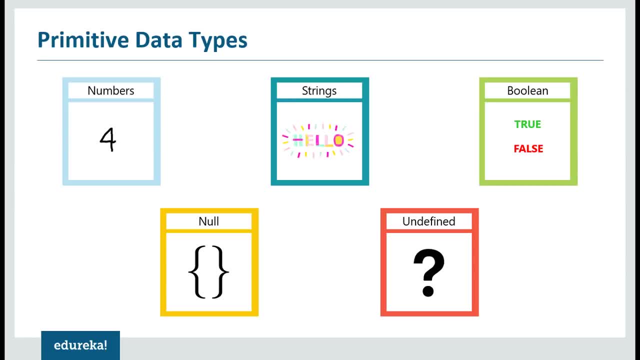 you can assign to a variable in javascript. we have two categories of data types. one is a primitive and the next is the reference data types. okay, now, under primitive, we have numbers, we have strings, boolean, null and undefined. now let's see how to declare each of these data types. 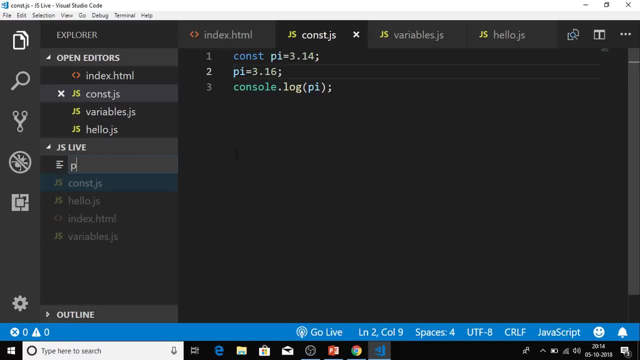 okay, now i'm going to create a new file over here. i'll name it primjs, okay. so first i'm going to declare a variable. let's call it name. all right, i'll pass the value edureka into it. now, what i did here is i created a variable called name and i created it using the let. 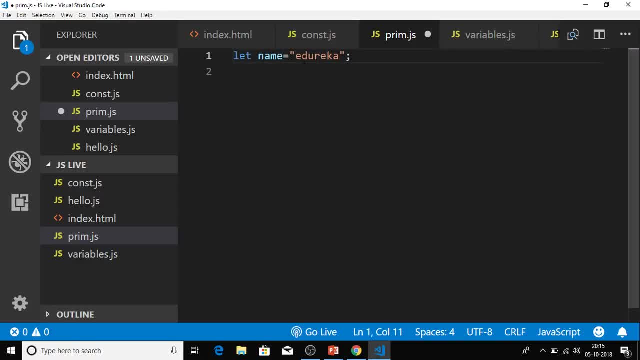 keyword. okay now, one important point to note here is: i declared the value of this variable within, uh, double quotations, or you can even declare it within single quotations. so what i did was, if i, uh, if i ever um enclose the value of a variable within quotation marks, then uh the computer. 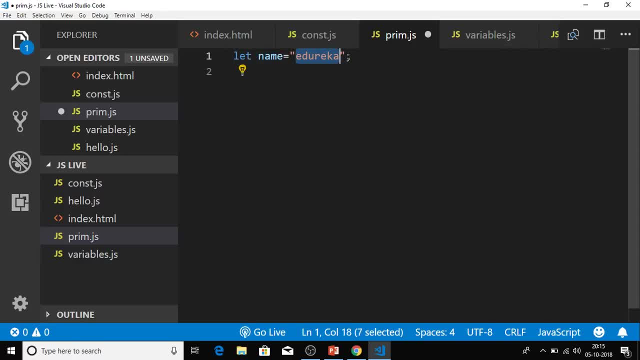 considers this to be a string. whatever is stored within these quotation marks is a string. okay, now, similarly, let's define a number. so let's define age equal to 30.. so this is basically a number. i've used the let keyword and i've set the value of h to 30, which is a number. all right. now let's see. 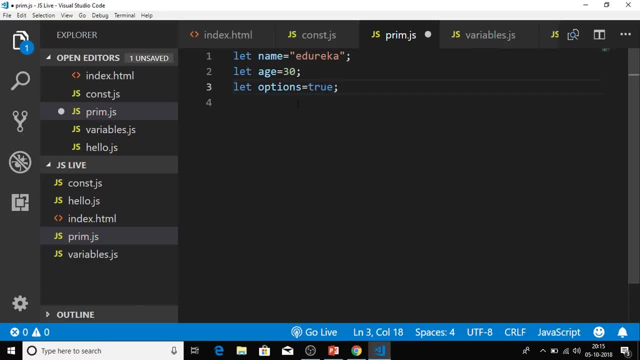 what this means. okay, so if i say: let options equals to true, now this is basically a boolean. okay, boolean can have two type, two values. it can either have true or it can have false. okay, you can use this in logical programs. your booleans are very useful in logical programs. okay, now let's. 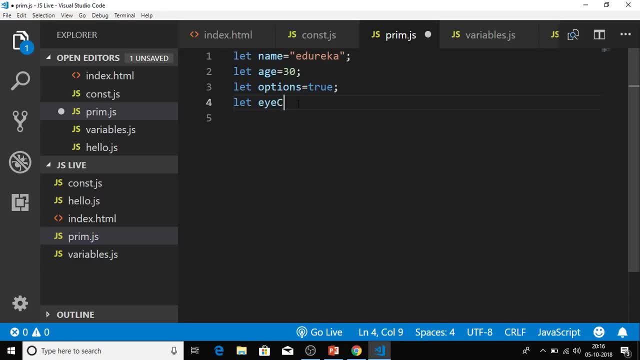 see another type: i color. okay, i'm defining a variable called i color and i'm setting it to null. now, these are null variables. now when, whenever you use a null variable, when you want to explicitly clear the value of a variable, okay, that's when you use a null variable, null variable. 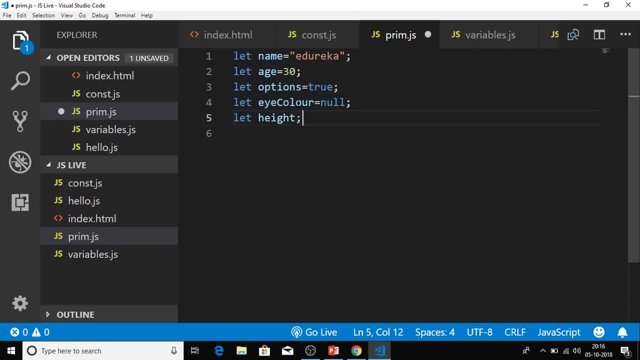 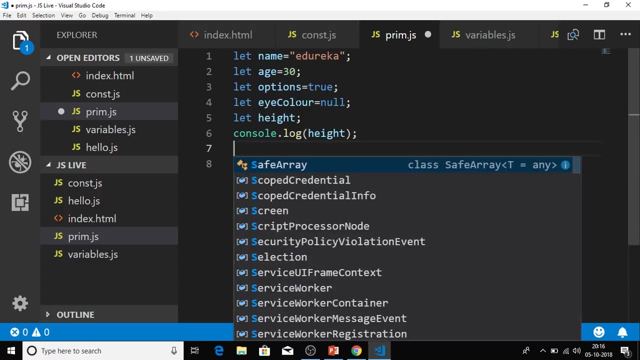 okay, now i'm defining another variable called height. i'm not set set the value of this variable. i haven't initialized it to anything. now let's see what happens when we try to log this height variable onto the console. all right, now save the changes and don't forget to change the name over here. 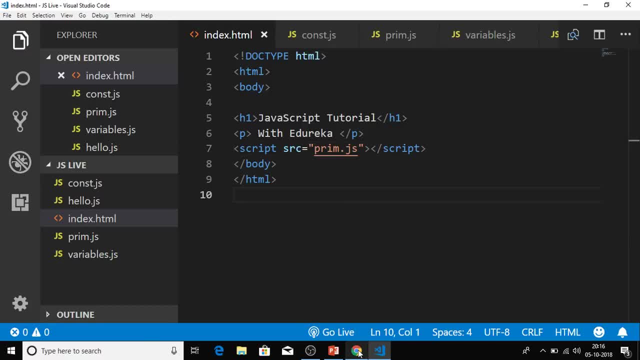 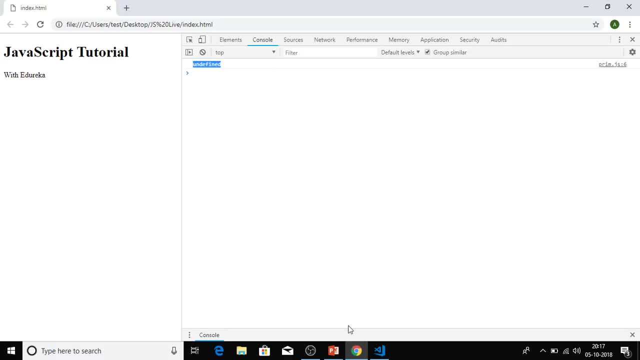 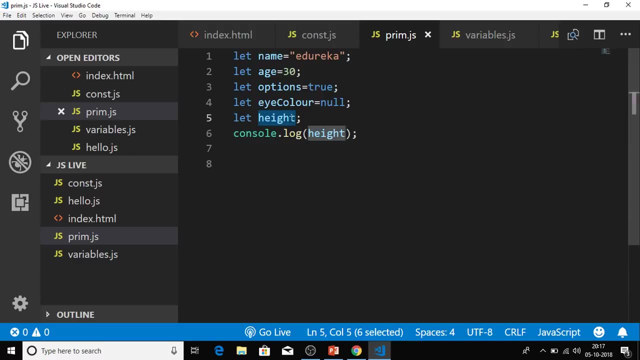 all, right now save this as well and open up your browser and refresh. okay, so here you can see that it's given undefined. now, uh, this means that, uh, look, when we declared a undefined variable, when we declared height as a variable, we didn't initialize its value to. 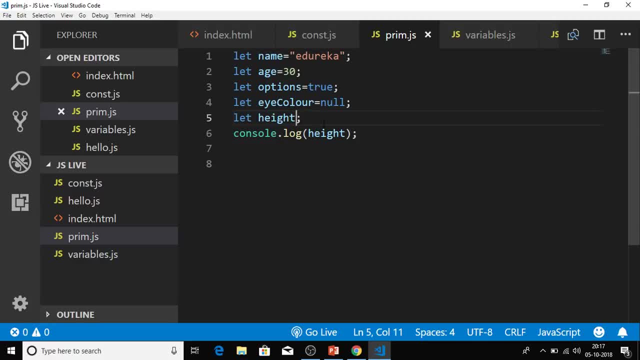 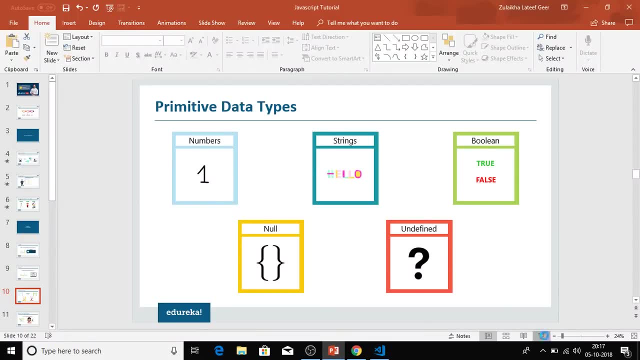 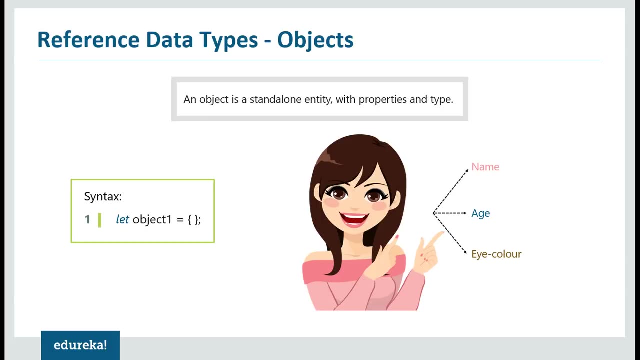 anything. so we didn't set the value to anything, so that's why it's an undefined variable. so this is also one data type in javascript. okay, guys, so with that we're done with primitive data types. now the next topic we're gonna look at is objects. so what are objects? objects? an object is basically. 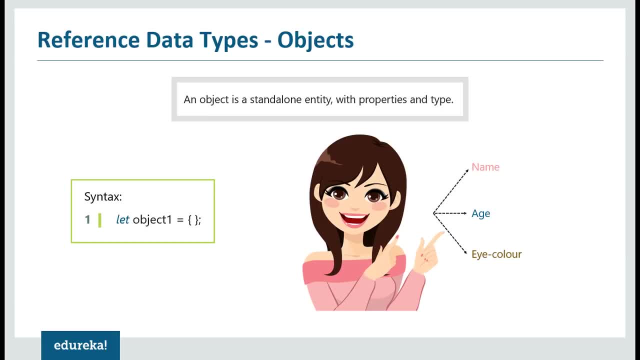 a standalone entity which has property and type. okay, so an object in javascript is a lot like an object in real life. so let's consider a girl. okay, now a girl has properties like her name, her age, her eye color- all of these are her properties. now, these properties obviously have some values. 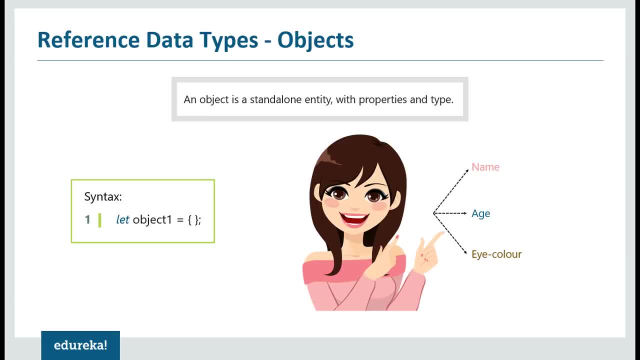 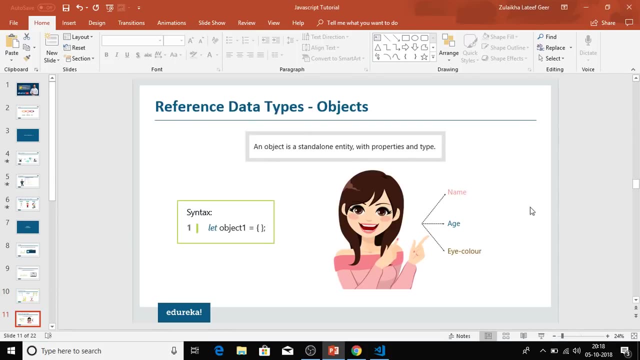 like her name may be emily, age is 22, eye color is brown, something like that. okay, so what i'm trying to say is: the girl is the object here and she has properties such as name, age and eye color, and she has values of those properties. okay, so this is how objects work. now, to understand it better, let's see. 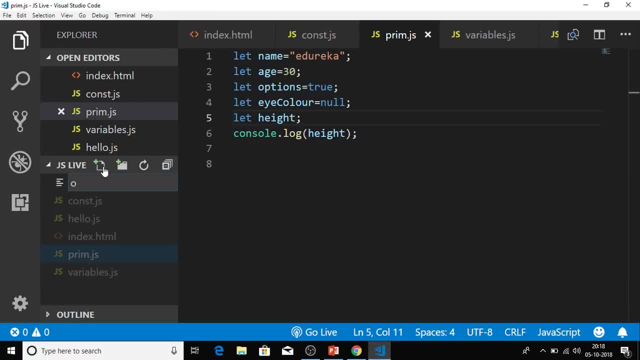 how to declare an object. okay now, let's add a file. i'll name it objectjs. okay now, over here i'm going to declare a object called pen. now, because an object is basically a variable, you use the let keyword itself to define an object. okay now, object is a variable which has properties and value pairs. 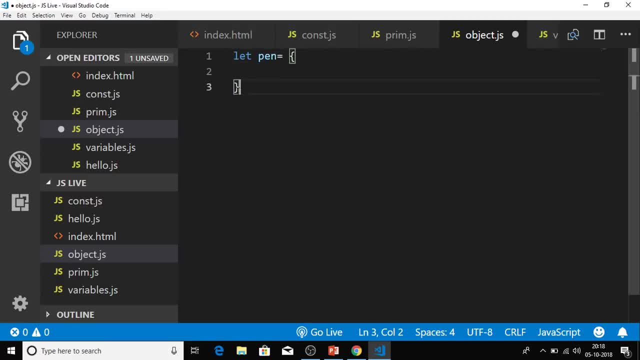 okay, so that's why you're going to have a set of pairs. so for that we are going to using these curly brackets. okay, now, within these brackets you're going to specify the type, the property and the value of the property. so let's say the first property is the type of pen, whether. 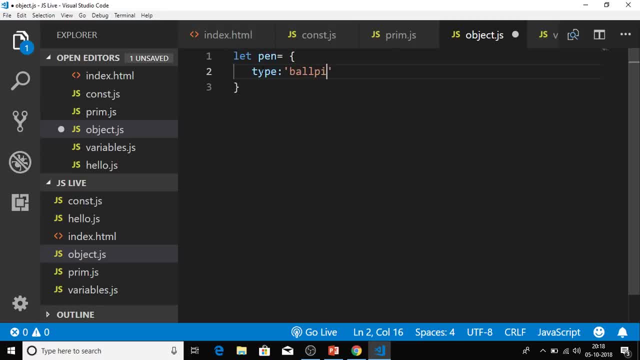 it's ballpoint or whether it is gel point pen. so i'm going to declare the first property, which is type: okay, the value of this is ballpoint. next, let's look at the color of the pen. so let's say it's black. similarly, we'll define another property cost and we'll set it to. 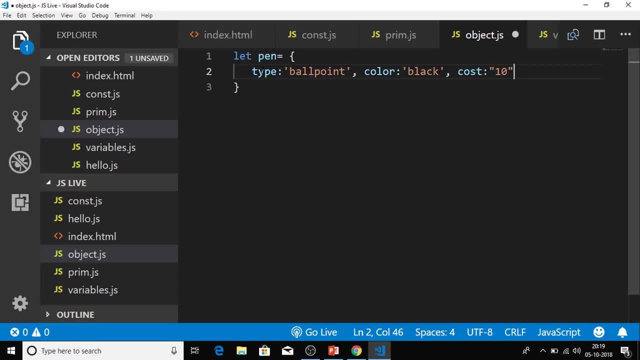 10. okay, so this is the cost. okay, now let's say that i just want to see the cost of the pen. so how am i going to get the cost of the pen? what i can do is, in order to access a property of an object, you use the following syntax. so the syntax is basically object name, dot, property name. when you 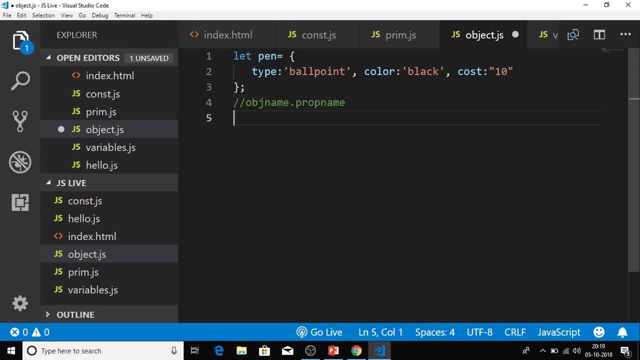 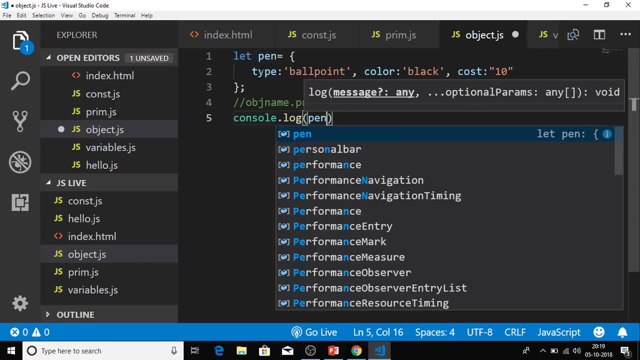 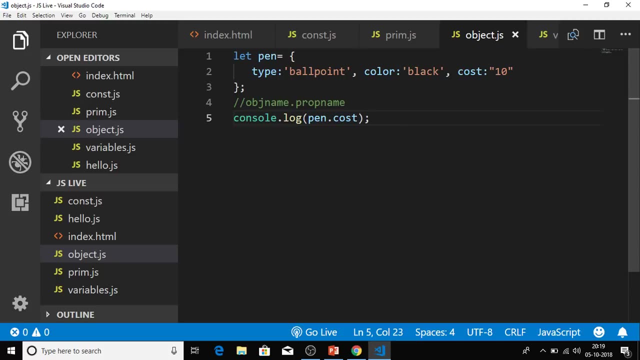 follow this, you'll be able to access the property. okay, so let's just print the cost of this pen. so you do that is, you write the object name first, which is pen, dot the cost, which is the property name. all right, now this will get logged to the console. let's save this file and let's 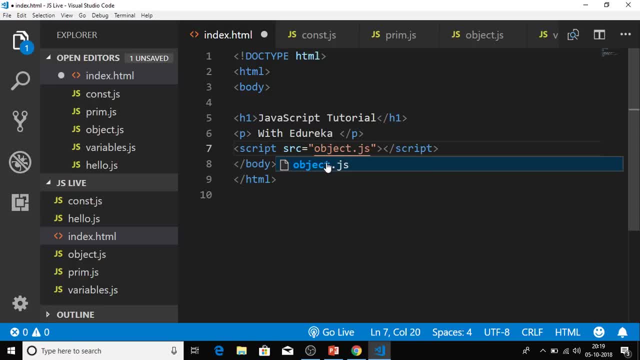 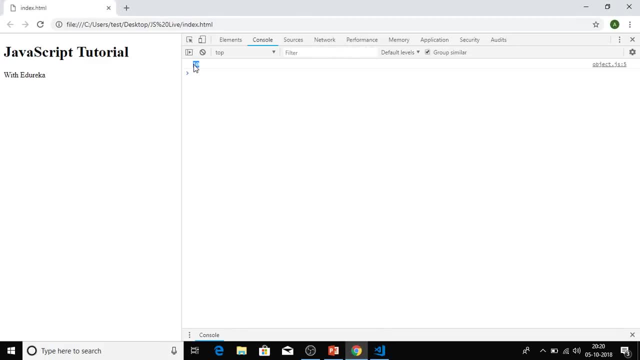 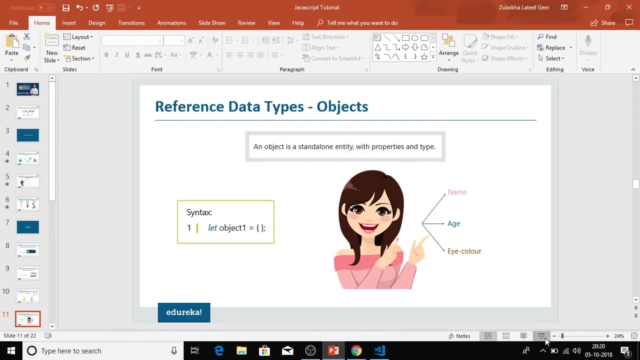 reference it from the html file. all right now, save this and let's run the code. okay, so the cost is displayed as 10. okay, so this is how objects work. now we're done with objects. let's look at our next reference data type, which is arrays. all right now. arrays are used to store. 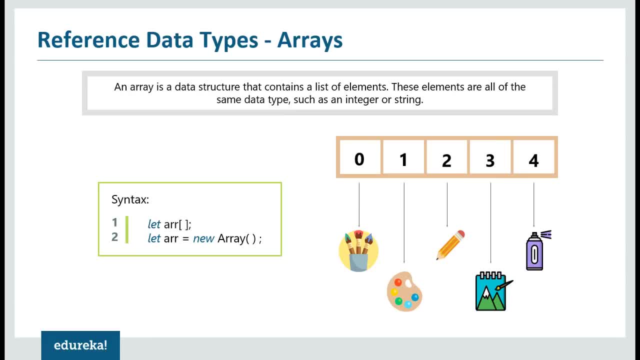 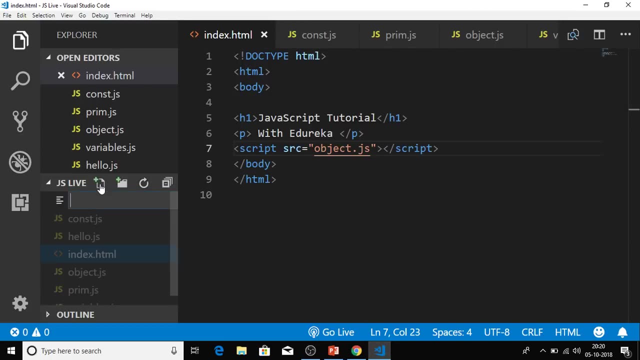 multiple values in a single variable. so if you have a list of items, let's say that you went shopping for some art supplies, okay, and you want to list down these art supplies in a array. so how you can, how you can do that is open up your visual studio code and i'm going to open a new file called 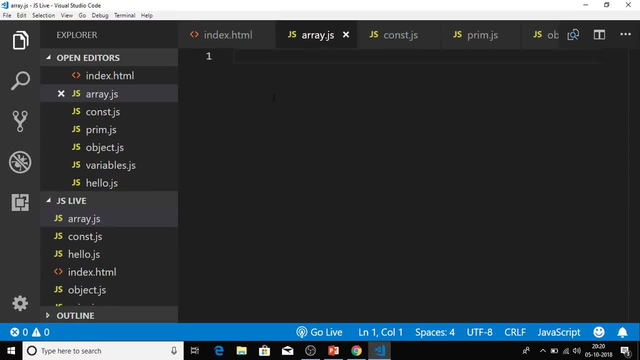 arrayjs. now here i'm going to declare a new file called array dot js. now here i'm going to declare an array. so to declare an array, the name of the array is shopping and you use the square brackets to declare an array. okay, because array is also a variable, so you're going to use the let keyword. 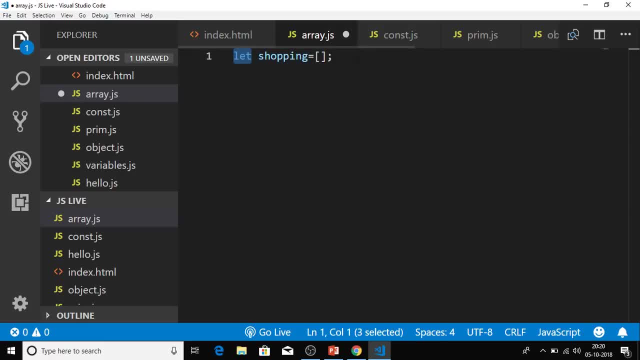 it's basically a variable which can store multiple values. okay, now let's add array elements. now, let's say i got a paint brush. okay, then another array element is spray paint and let's say canvas. okay now. um, so basically what i've done is i've listed down the array elements over here. now paint. 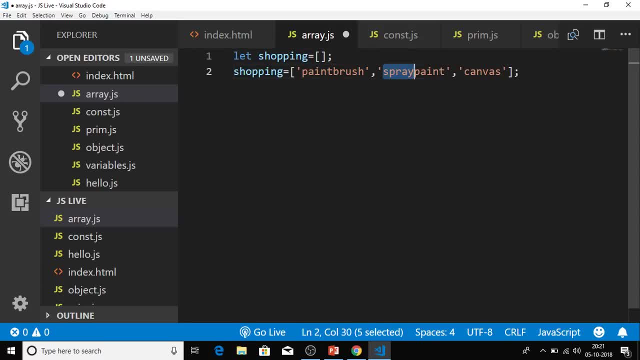 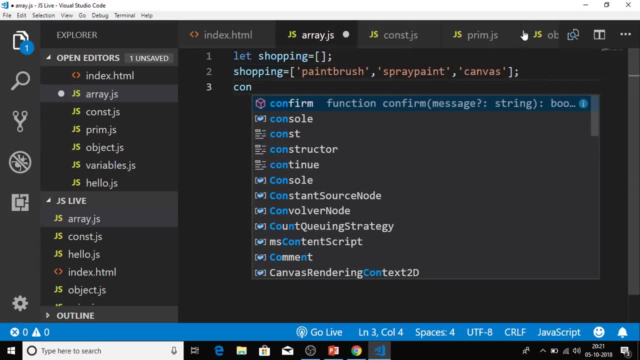 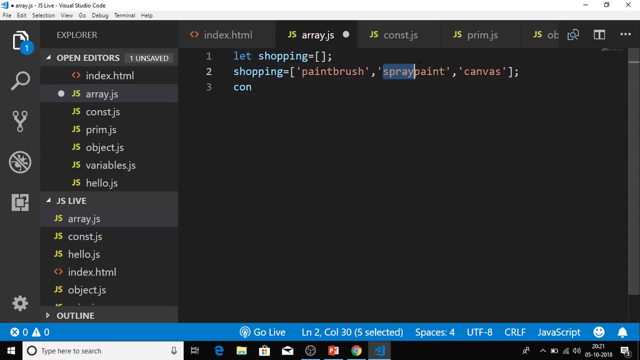 brush is one array element. i've separated it with a comma and defined another array element, and so on. now, in order to access an array element, what do you do? so let's try to print the array element which is at the second position. okay, so let's try to print spray paint. how are we going to do that? 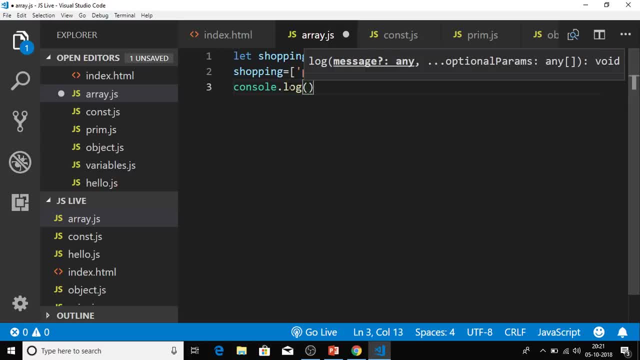 so let's use the log function. now, here i'm going to name, put the name of the array which is shopping, and within square brackets i'm going to put the index of spray paint. now, the index of spray paint is going to be one, because arrays start from zero. so at zero position we have paint brush. 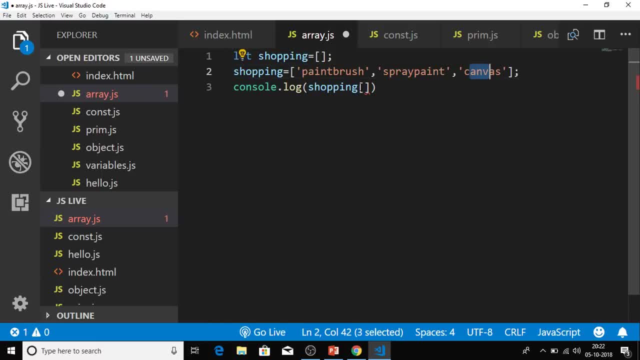 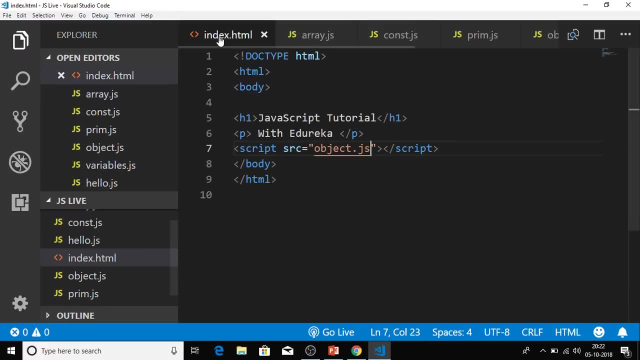 one, we have spray paint and two: we have canvas. okay, so i'm going to give one over here. let's save this, and let's also change the reference to array. all right now. uh, refresh your browser and here you can see spray paint. okay, so that's how arrays work. 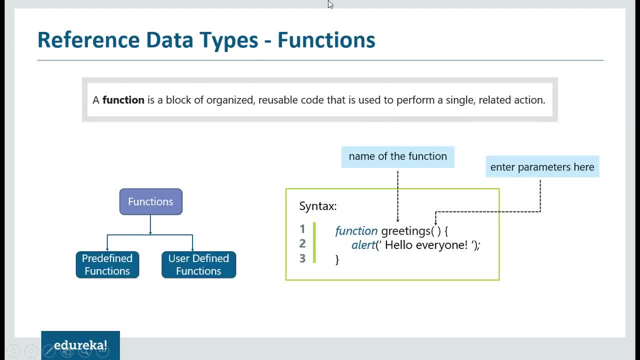 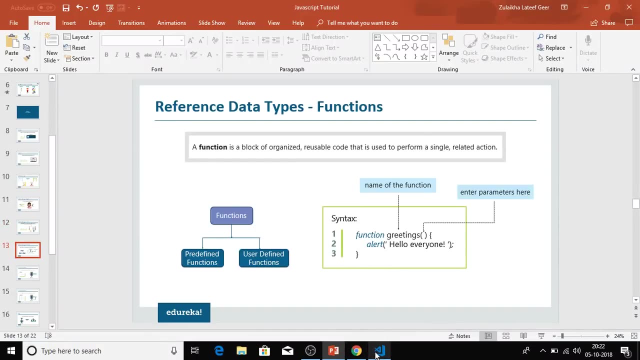 all right, now let's move on to functions. now, um, functions are basically our basic building blocks in javascript. now it's a set of statements that perform some tasks. okay, now, don't worry about what all is written here. i'll explain everything with the help of an example. so let's open up. 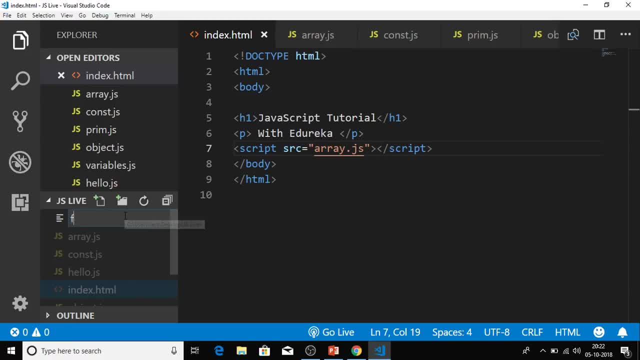 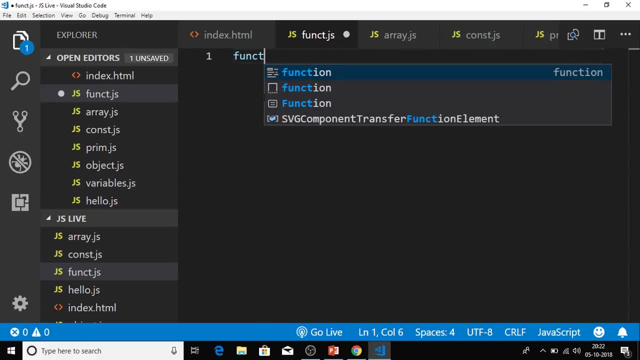 visual studio code. i'm going to open a new file. i'll call it functionjs. all right, now what i'm going to do is i'll declare a function using the function keyword. so function is the keyword you use for declaring a function. now the name of this function is prod and i'm going to pass two. 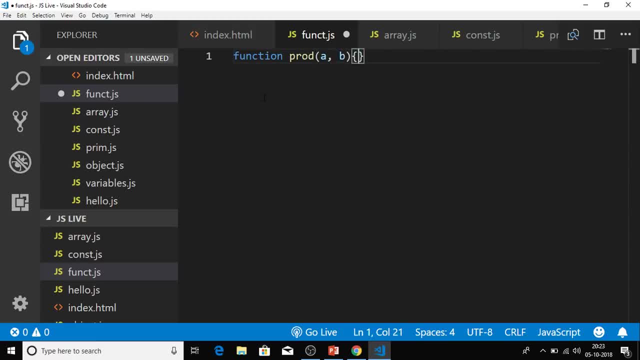 variables as parameters to this function. okay, and within the body of the function, i'm going to return the product of these two variables. so a star b, all right. now you have to end it with a semicolon. okay, now, what i did here is i created a function called prod, and i did this by using 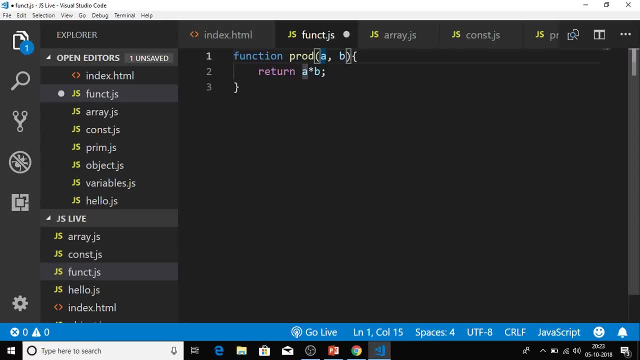 the function keyword. okay, and this function has two parameters to it, variable a and variable b. now, in order, right for a function to return some value, like, for example, if i want to actually calculate the value, the product of two variables, what i'm going to do is i'm going to call this function so how you call. 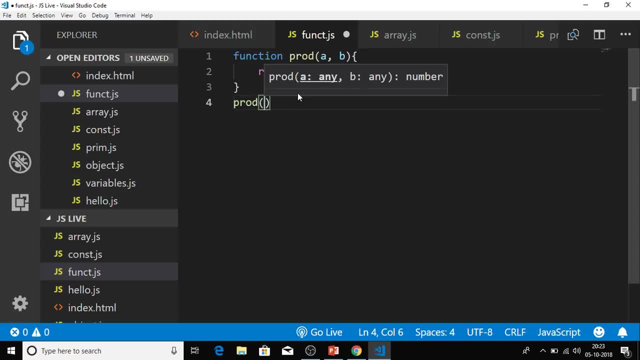 the function is the name of the function and you specify the values to these variables that you declared here. so a and b, you have to set the values over here. now these are known as arguments. okay, so here what i'm doing is i'm calling this function with these arguments. eight and two are 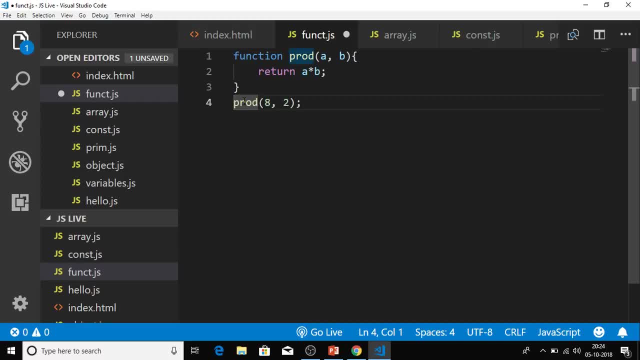 the arguments. okay, now what we'll do is we'll display the product of these two values. let's create a variable x. we'll store the value of the product in x and let's display it on the console. all right, save the changes and now open up html file. make sure you pass in. 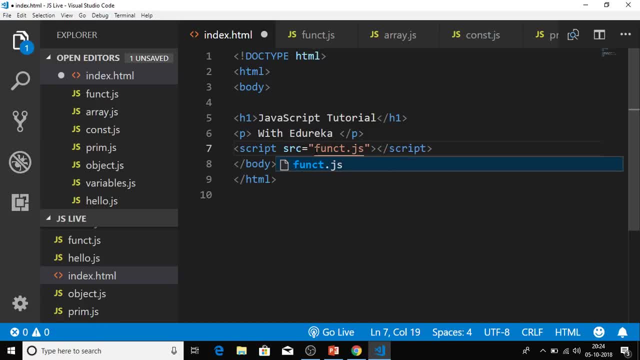 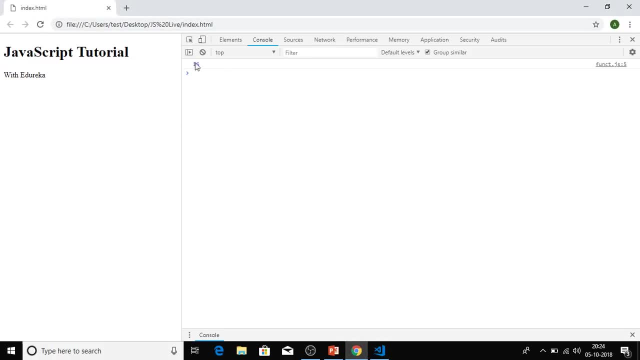 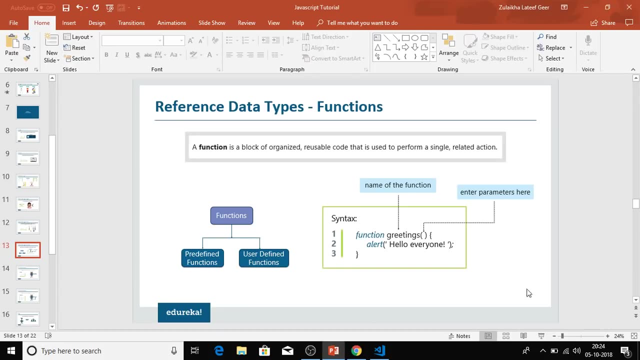 the name of the file. okay, save it and open up your browser. okay, so it's given us the product. 8 into 2 is 16. all right, so, guys, this is how functions are declared in javascript. so now that we're done with functions, the next thing we're going to look at is: 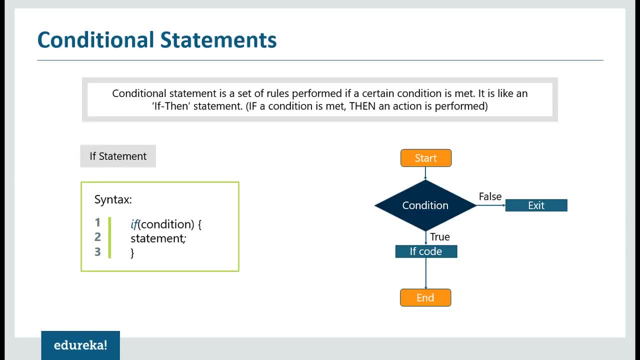 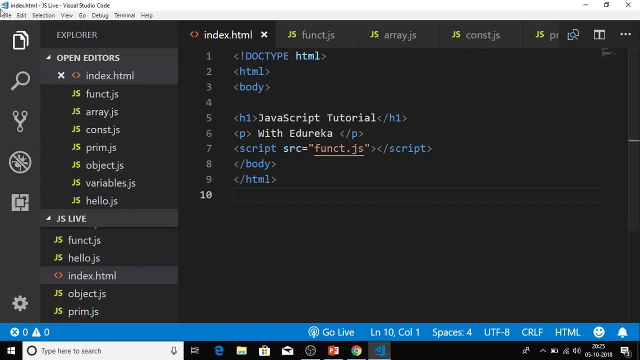 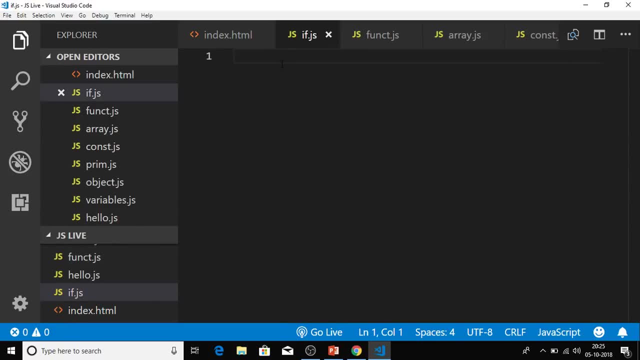 example, let's open up visual studio code. i'm going to open a new file. i'll call it ifjs. now, over here, let's type a code. so what i'm doing is first i'm declaring an array called numbers. okay, now i'm going to add some array elements into this. 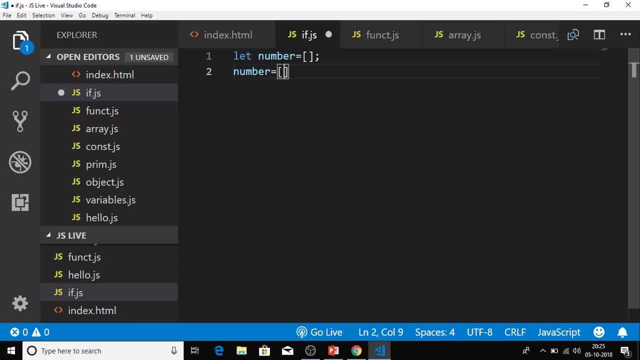 so this is how you add array elements. so let's just randomly add some numbers over here. okay, now i'm going to define a if loop. now let me just write the condition and then i'll tell you what it means. so i'm just going to put number at zero, equal to, equal to number at two. 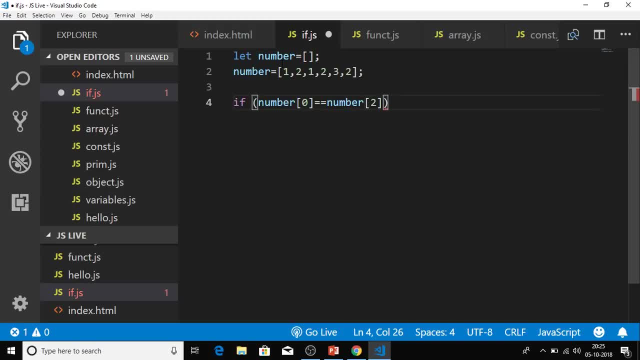 okay now, if this statement or if this condition holds true, then it's going to execute some code. so the code that is going to execute is this: we're going to print correct. okay, now let me tell you what i've done here. so first i've created an array called number. 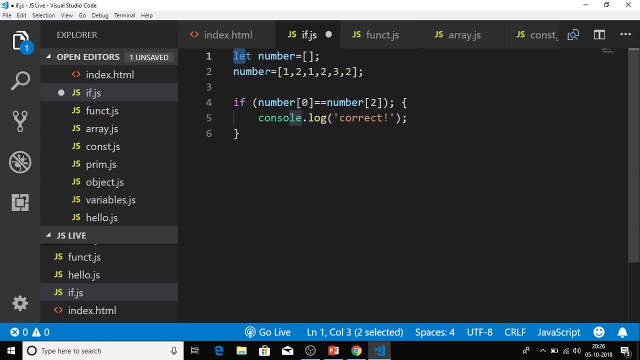 using this let keyword. okay, so this is how you create an array. then i've listed a few array elements over here. now what i'm doing is i'm checking. if this condition holds true, then this code will get executed. so the code within the loop will get executed, okay. 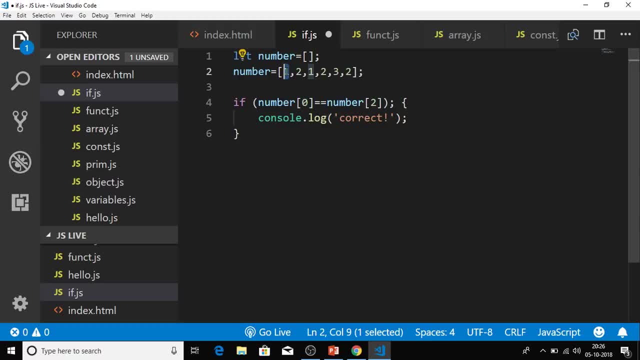 now number at zero position, which is one. i'm checking if this- the value at the value of number at zero- is equal to equal to the value of number at number two, number with index two. so basically i'm going to check if this and this is equal. okay, so one and one are equal, so this should definitely execute the block. 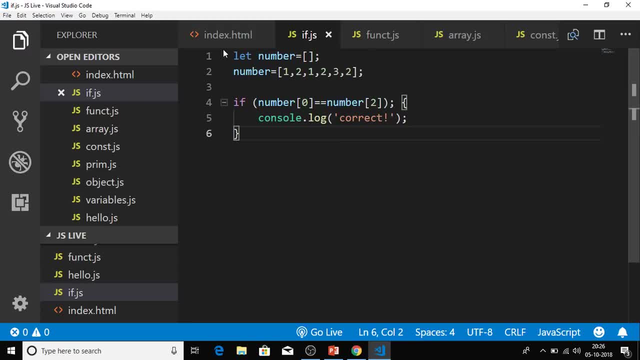 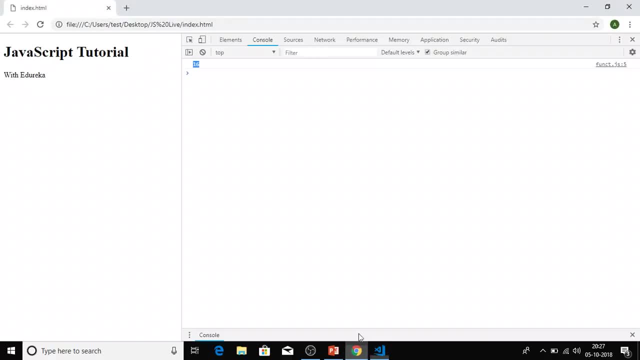 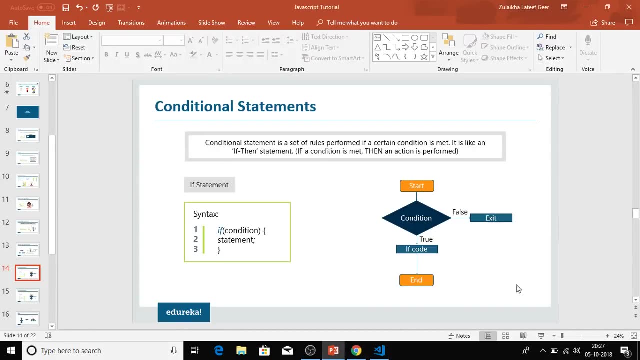 of code within the if loop. okay, now let's save this and let's reference it from our indexhtml file. all right, save the changes and open up your browser. yeah, see, it prints correct. okay, now this is how an if statement is used. now, the next thing i'll be talking about is the if else statement. 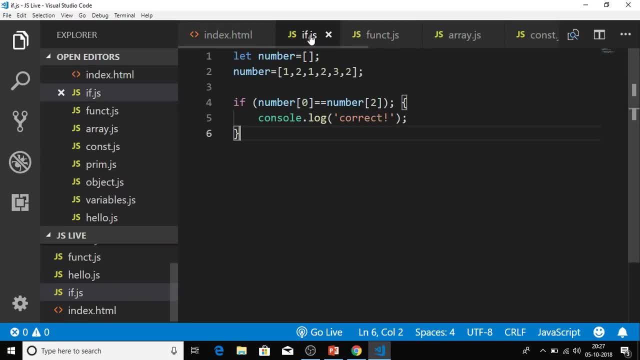 okay, let me just show you directly on visual studio code. so now an else is used whenever you want to execute a block of code if the condition is false. now let's say that this condition is false. all right, this condition holds false and you want to execute something else? then what do you do? is you define an else loop. okay, now. 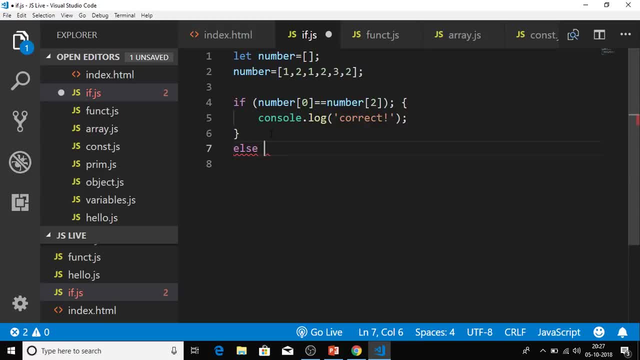 let's say that if that condition is not met, i'm going to log this to the console. wrong, okay, so all right, now let's save this and let's change this value. okay, let's make sure that this condition is false. let's set this to one and this to two, so it's going to compare this value and 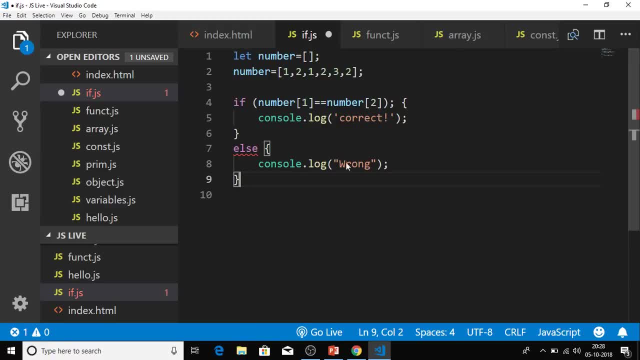 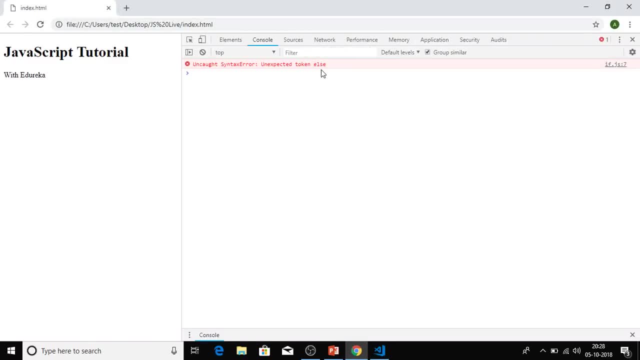 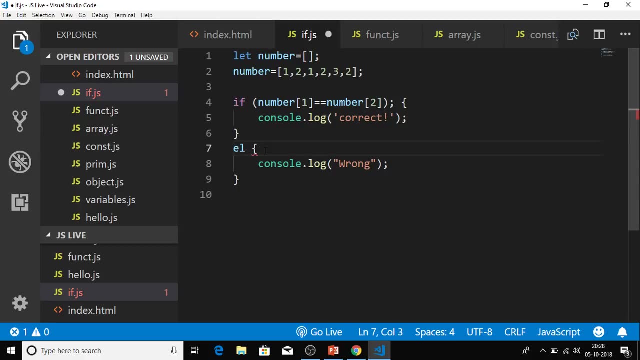 this value. now, these two values are not equal, so i should basically get wrong as the answer. okay, let's save this, let's open this up. okay, there is an arrow over here. okay, um, one second, guys. so i've declared the if all. right? uh, so i'm facing a small error here, so i'm going to go ahead and do that and i'm going to. 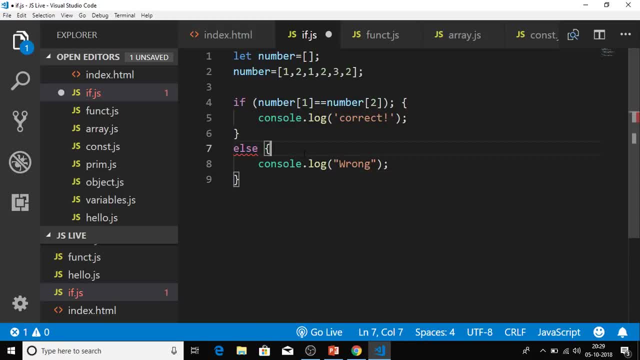 go ahead and do that and i'm going to go ahead and do that and i'm going to go ahead and do that problem over here. okay, i'll try to solve this before the end of the demo. so now, what would happen here technically is whenever this condition wouldn't hold true. this else block would get. 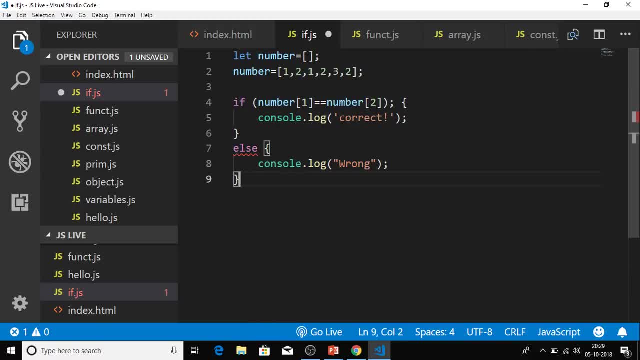 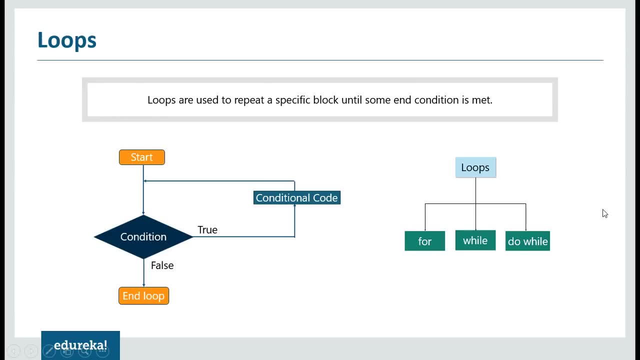 executed. okay, so this else block gets executed whenever this condition does not hold true. okay, now let's uh look at our next topic, which is loops. now, loops are basically used to- um, they are used throughout a block. uh, whenever you want to repeat it, basically do the same thing. so if you want to repeatedly do, uh like a run of specific code, 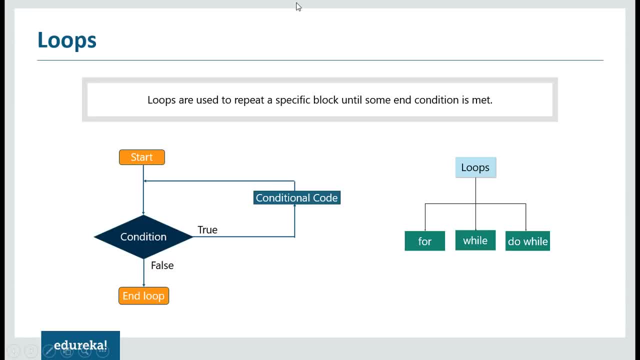 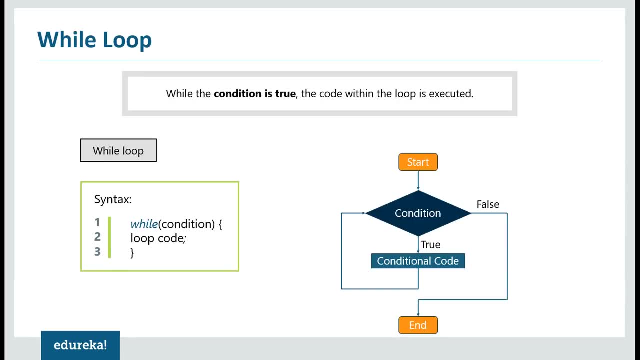 then you can use loops. okay now, um, there are three different loops in javascript: there's for loop, there's while and there's do while loop. so let's look at the while loop first. now while basically loops through a block of code as long as the specified condition holds true. so here, whenever, 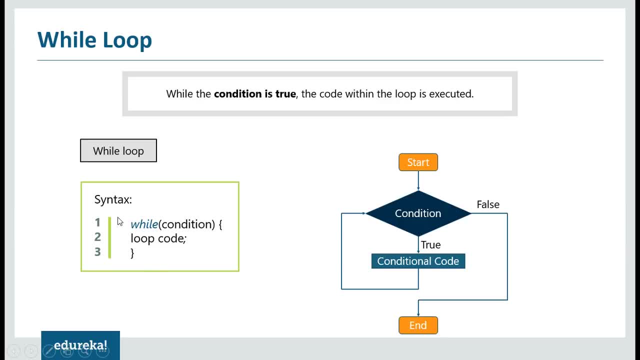 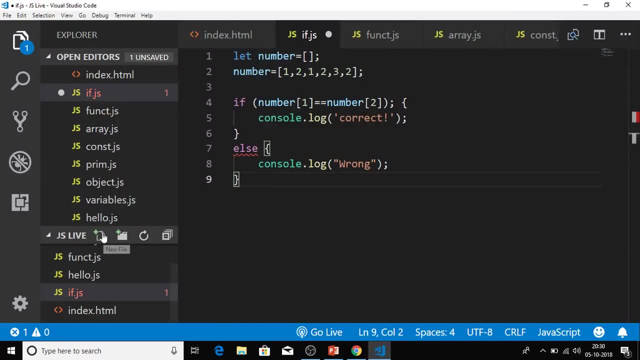 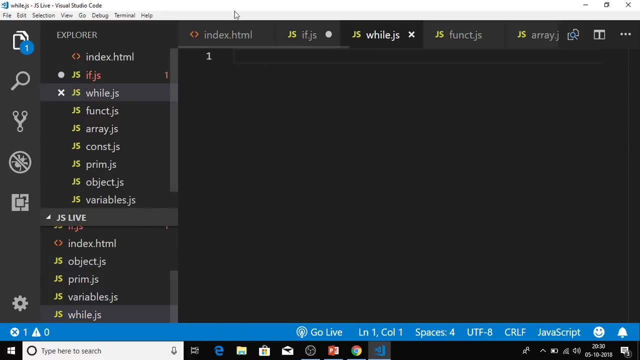 the condition is met, this while loop will get executed. okay, now, um, let's look at an example. let's try to run an example over here. so i'm going to create a new file. i'll name it while dot, js. all, right, now what i'm going to do is, first, i'm going to initialize the value of i. i'll set it to. 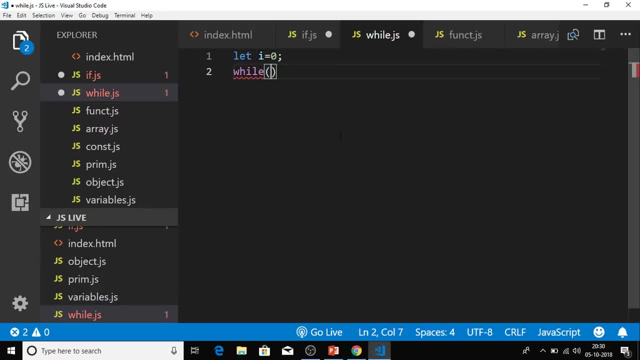 zero, and now i'll open a while loop. now, within this while loop, i'll set a condition, which is whenever i is less than five. okay, now, what i can do is, within this, whenever- uh, whenever- i is less than five, i'm going to set a condition, which is whenever i is less than five. 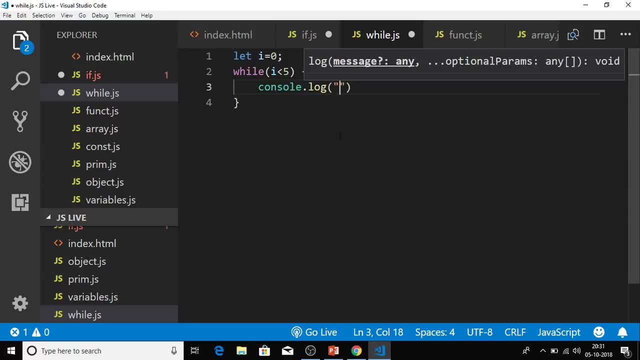 it's, it's going to execute this code. okay, so let's just display the number is and we'll display the number i, okay, and after executing this, it will just increment i, all right. so what i'm doing here is: first i'm setting the value of i to zero, then i'm defining a while loop within which i'm setting 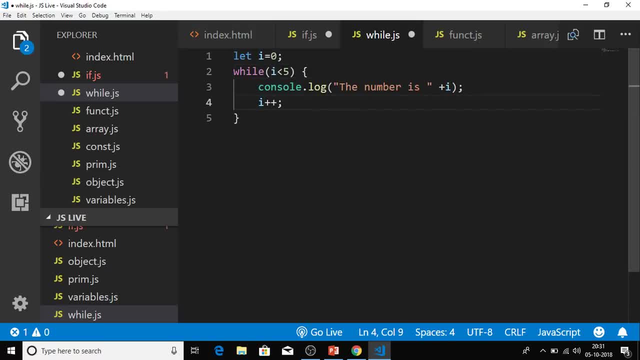 a condition: i is less than five. okay, now, whenever i is less than five, the consolelog- this uh function gets executed. that is, this will get printed on the screen. so whenever i is less than five, the consolelog- this uh function gets executed. that is, this will get printed on the. 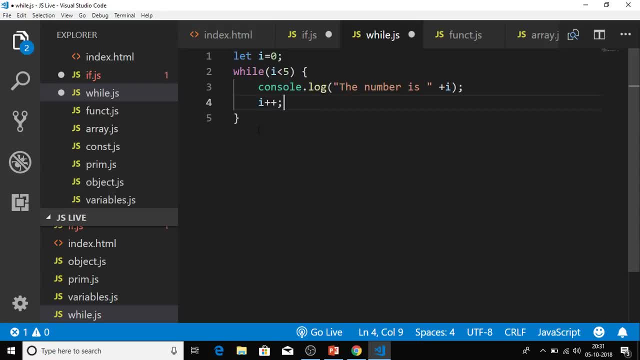 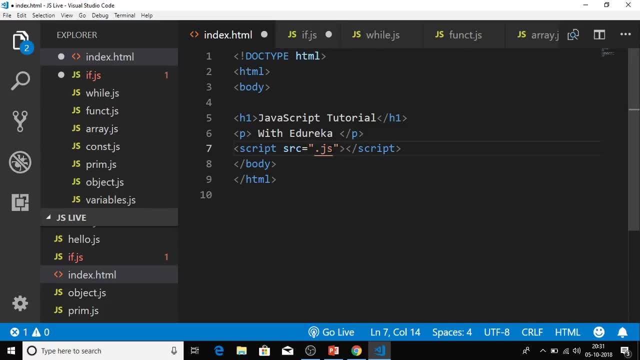 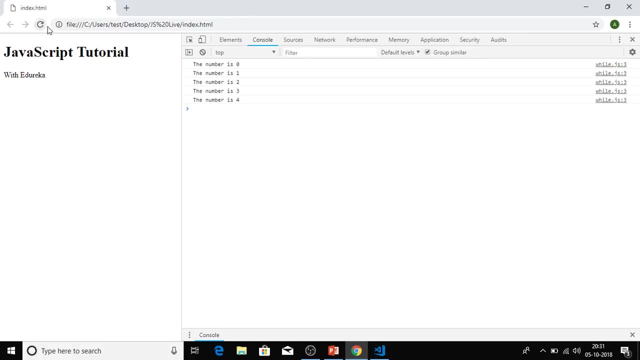 screen okay, and after that it will keep incrementing the value of i. okay, so now let's save the changes. over here, let's go to indexhtml and let's pass, while over here, let's save this and let's open this up. okay. so here you can see that the while loop has. 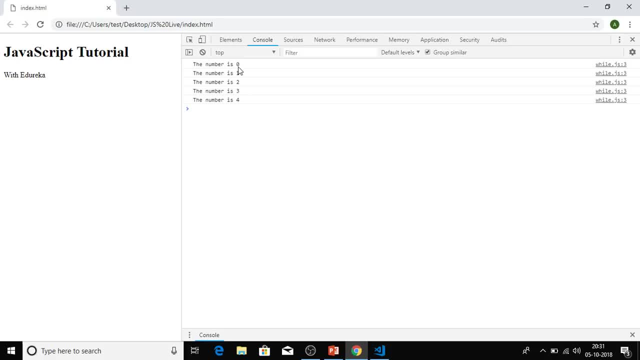 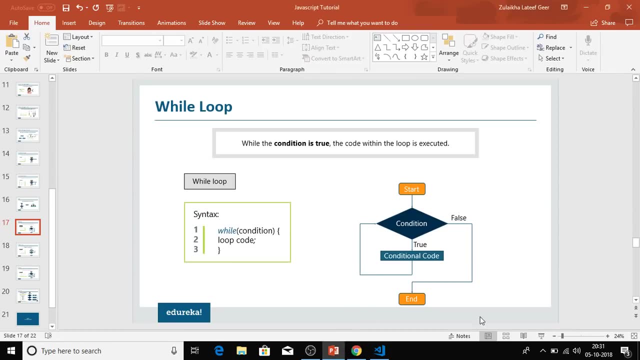 executed this, uh, four times. so totally five times actually, because it starts from zero. so as long as i is less than five, these um values get printed. okay, so that was while loop. now let's look at do while loop. now. do while is basically a variant of the. 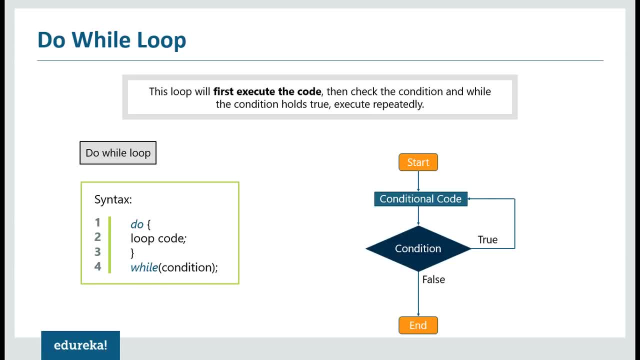 while loop. this loop executes the code block once before checking if the condition is true, then it will repeat the repeat this. repeat the loop as long as the condition is true. so basically, it will run this loop code once and only then it will check the condition. now, if the condition. 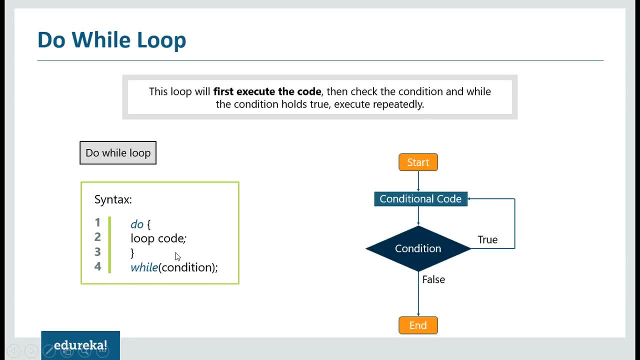 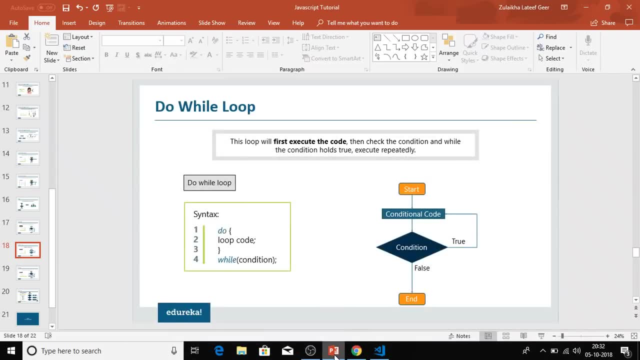 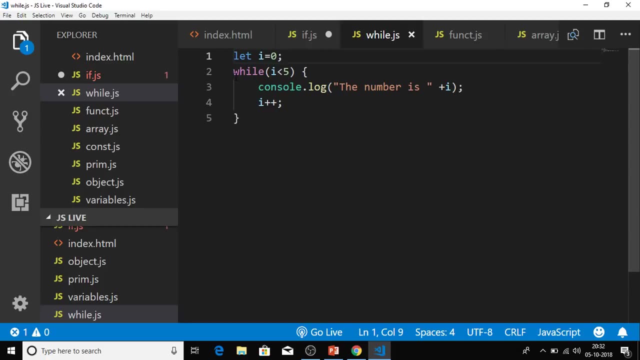 holds true, the second time it will repeat. it will execute the code. okay, so it first executes the code once and then checks the condition. now let's look at the same example. so what i'm going to do here is, let me just add: do over here. now, first you define, do block. 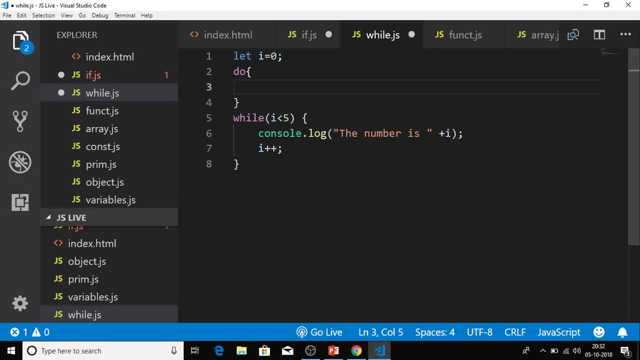 now, within this, you're going to have this entire code. okay, so what i did here was i opened a do loop and within the do loop i had a simple function which says console log and it basically logs this to a console and it increments i. so the first time, 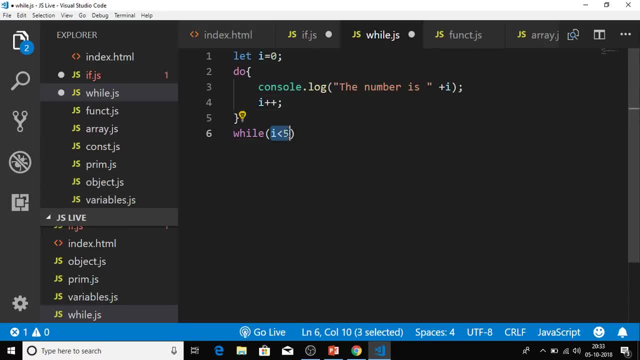 this, uh, this gets executed and after that this condition is checked. if i is less than five, let's actually make it i greater than five and let's see what happens. okay, now it'll check. if i is greater than five, then it'll go inside the do loop again. it'll run this condition, run this function and. 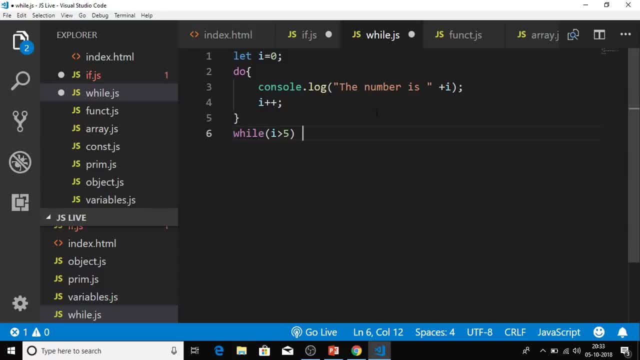 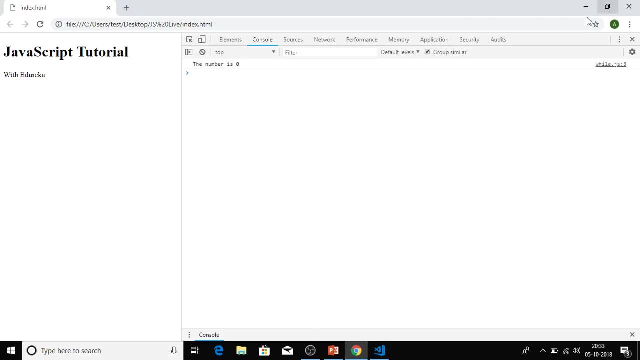 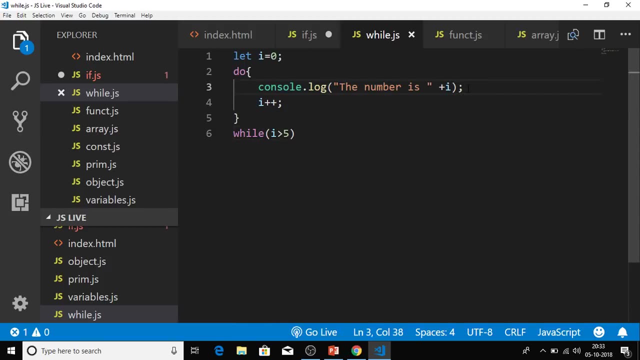 if this condition is not true, then it's not going to run the following code: okay, let's save this and let's open our browser. okay, now, this printed only once. now that happened because the condition does not hold true. it printed once because in a do loop, you have to execute the statement once. 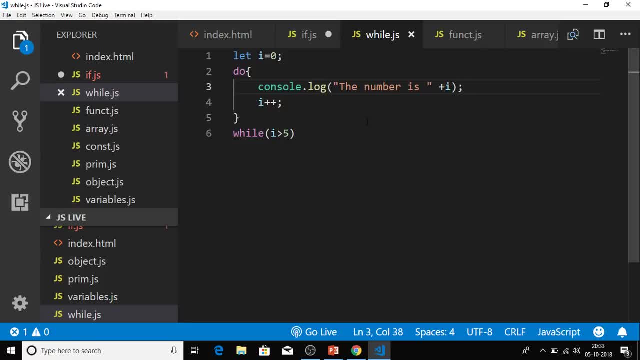 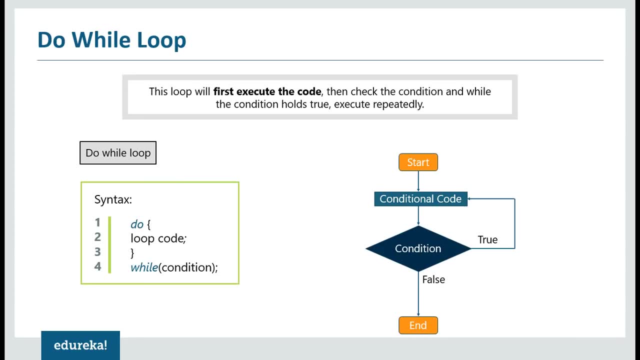 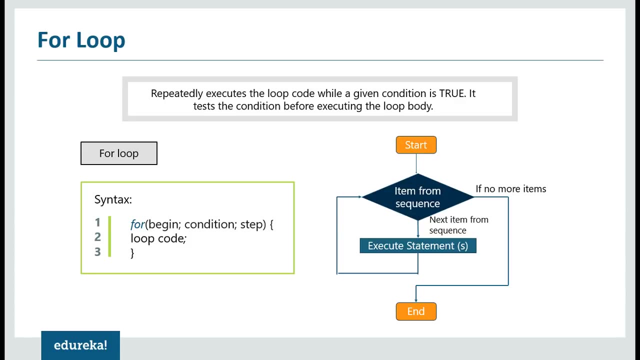 and then check the condition. the condition was false. that's why it didn't further execute this. all right now. that's the difference between while and do while loop. now let's look at the next topic, which is for loop. okay, now for loop has its own syntax. now, for has a begin statement, it has a condition, and then it. 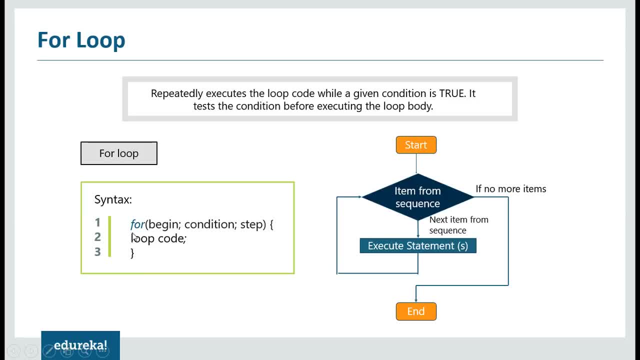 has a step. now. this begin is executed one time before the execution of this loop code. okay, now this condition will basically- it will define the condition for executing this code block. okay, whatever is there over here, it will define the condition for executing this and the last one. 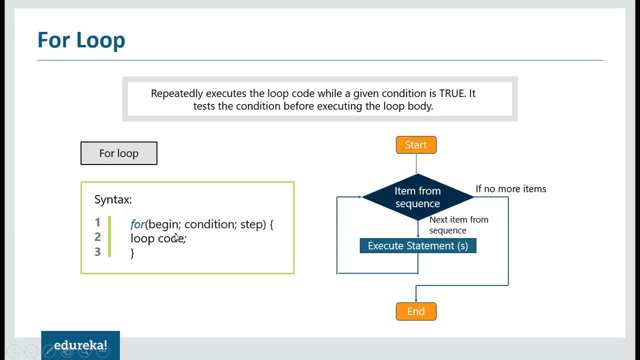 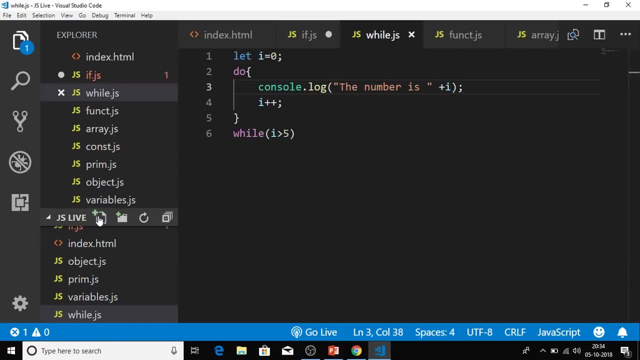 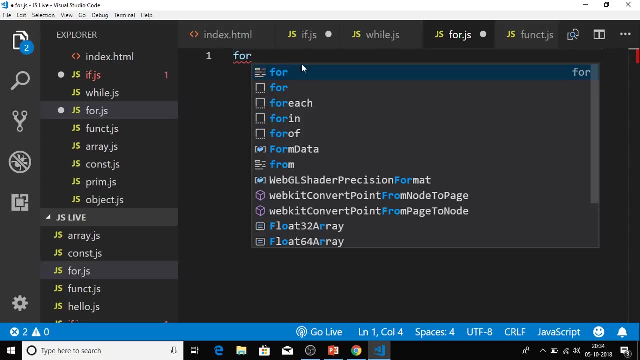 is step now. this is executed every time after this loop code is executed, so let's look at the condition for executing this. okay, so, guys, don't worry if you got confused, we'll practically do it now. so i'm adding a new file over here. i'll name it for dot js. okay, now let's create a for loop using: 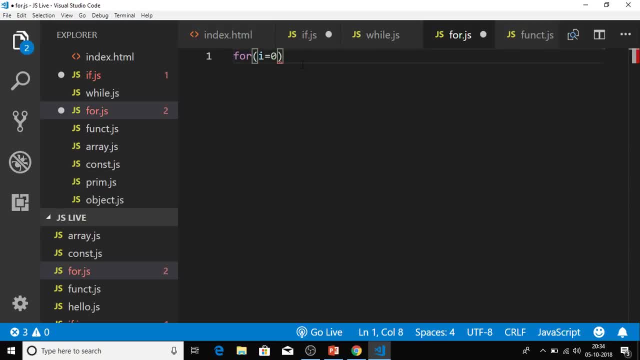 the for keyword. i'm setting i to zero first, and then i'm defining i less than five, which is the condition, and then i'm going to increment the value of i. okay, so this is basically my for loop. now, within the loop code, i'm going to create a for loop and then i'm going to increment the value of i. 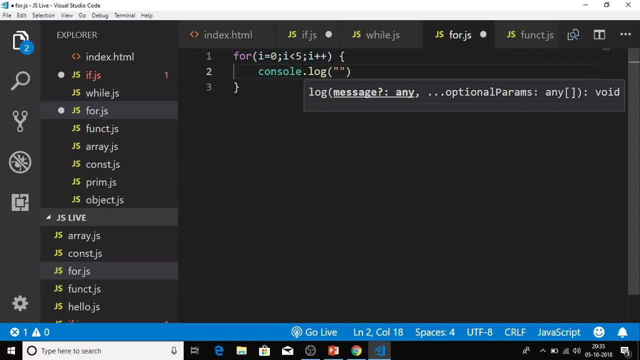 to log the same thing that we did for the while loop. okay, so i'm going to run the same message. the number is and. okay, so this i'm going to do. and then, um, yeah, so basically that's all, because here you automatically can increment it. now what happens in this for loop is: first you define the. 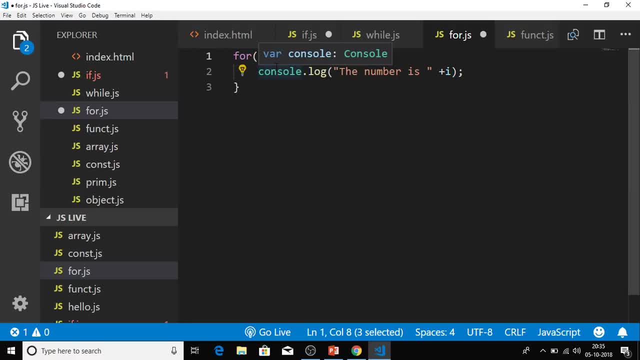 i equals to zero condition. now this is executed, uh, one time before the execution of the code block. so execute i is equal to zero and get, get into this loop and execute uh, this uh function okay. after that it's going to check the condition. if i is less than five, then it'll keep executing the loop. 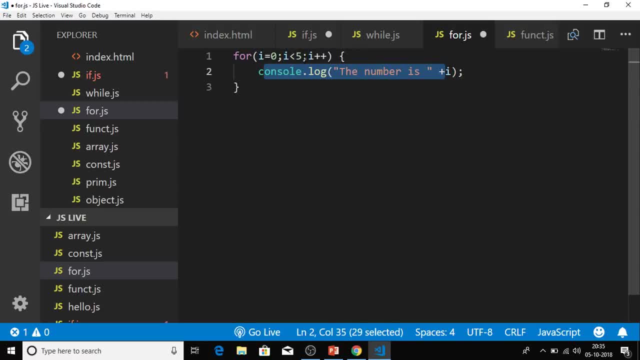 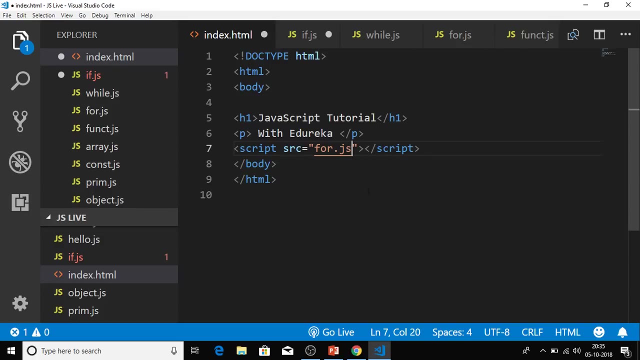 and after it's executed, the loop code it's going to increment the value of i. okay, so i plus plus is performed after this block code is executed. okay, now let's save the file and let's reference it from here. all right, let's save it and. 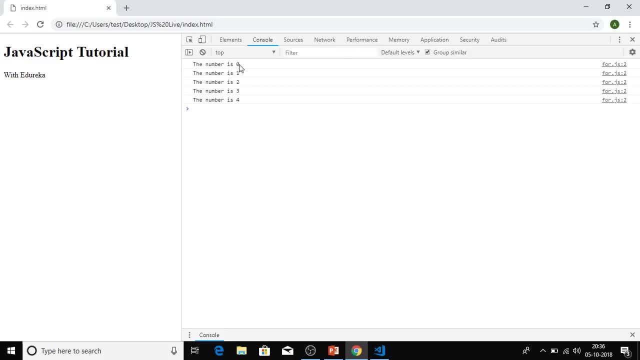 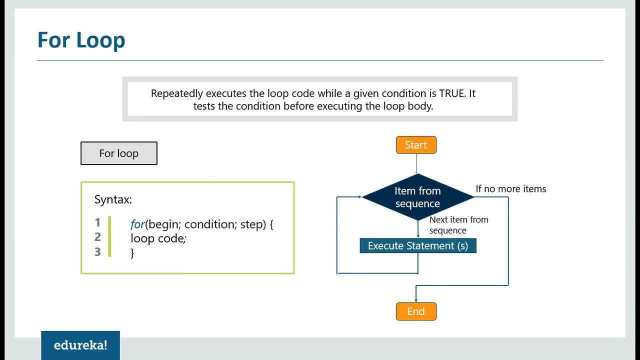 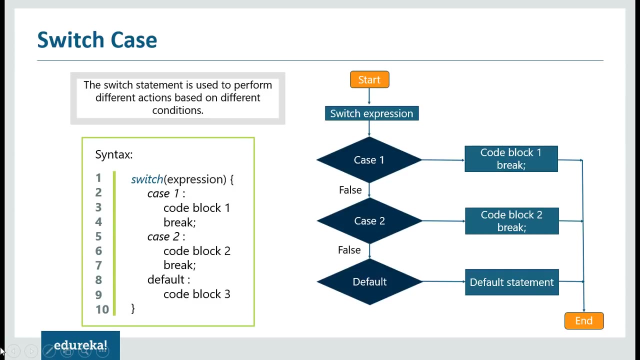 open up your browser. yeah, you can see that it's printing numbers from zero to four, so it's executed this loop five times. okay, so, guys, that's how the for loop works now. uh, at last, we're going to see switch statements now. switch statements are used to perform different actions based on different 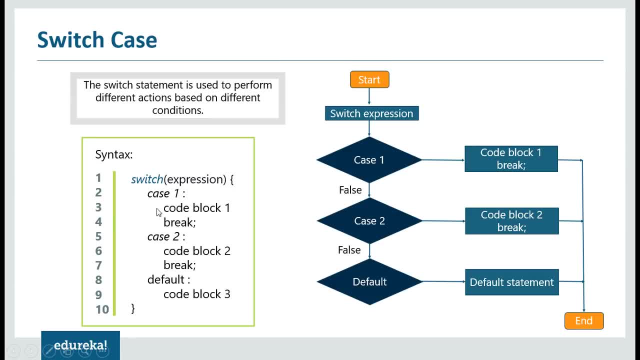 conditions. now, how does the switch, uh, switch- statement work? so, basically, switch expressions. these are switched expressions, whatever, whatever is defined within these switch brackets over here. we're going to call them switch expressions. now these get evaluated once. okay, so what happens is the value of this expression is compared to the value of each case. so the value of each case and 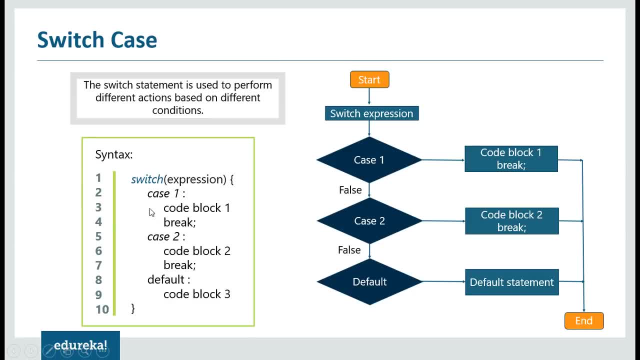 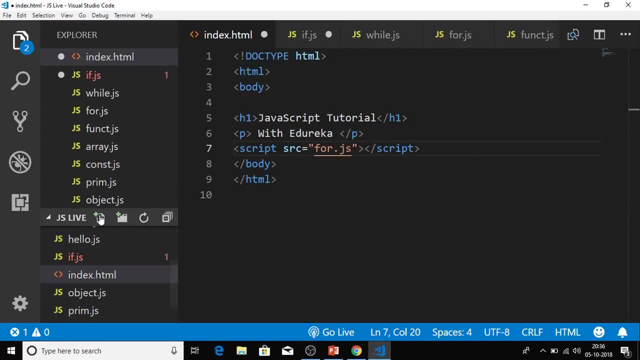 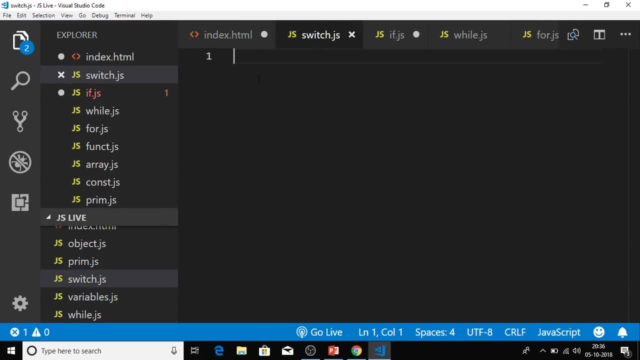 this expression is compared now, if the expression and the value of the case match, then that respective code block will be executed. okay, now don't get confused. we'll just run a simple code over here. we'll see how it's done. so i'm creating a file called switch. now let's create a 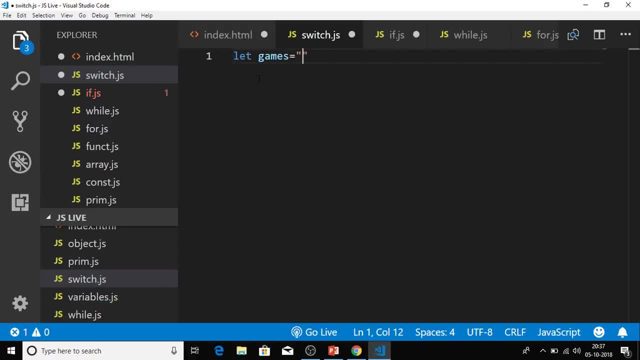 variable now. first, i'm just creating a variable called games and i'm setting its value to football. okay, now let's create the switch statement. now, within the switch statement, um, i'm going to pass the games variable and let's define the different cases now. so the first case: 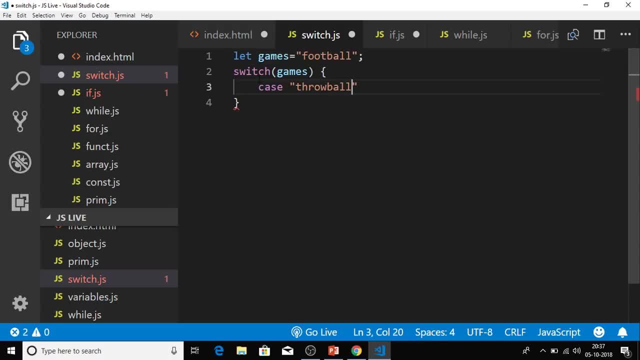 i'm going to set the value of the first case to throw ball. okay, now, after this, i'm going to have the code block that's going to get executed if this expression matches the um, if this case matches the expression. okay, so let's just say i. 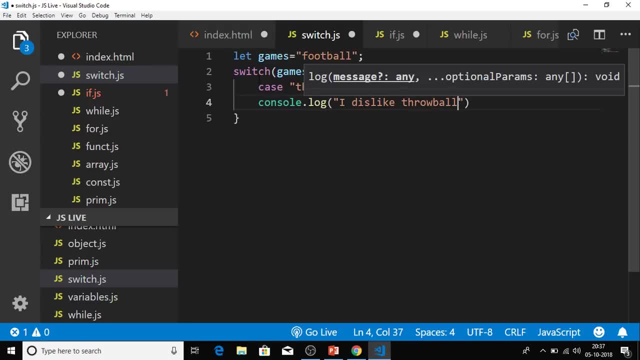 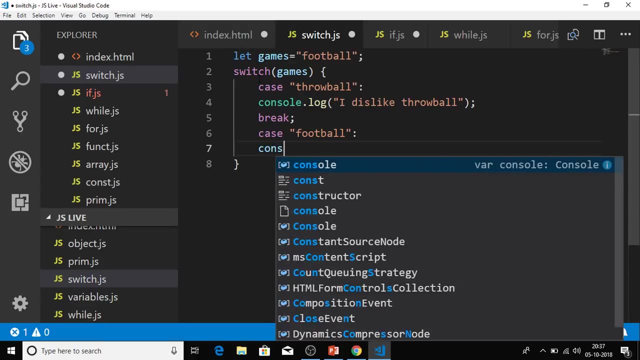 dislike: uh, throw ball, okay. and also, after every case, you're supposed to give a break. so this is how you define a break. now let's define another case, we'll name it football. and now let's define some code block that will get executed if this matches. so let's say: 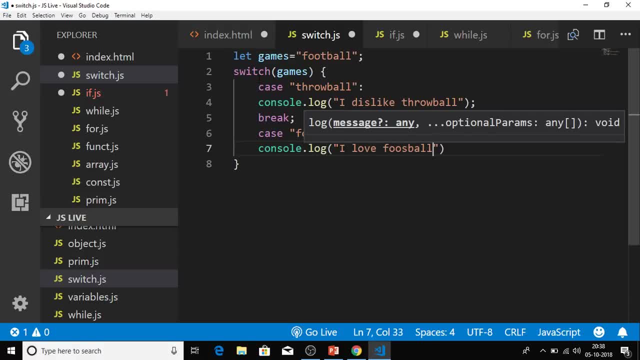 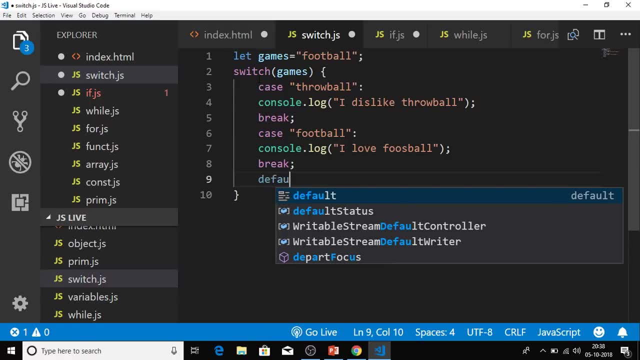 i love foosball- okay. now let's give a break after this. and another important thing you need to define is the default statement. now, in this default statement also, i'm going to have a code block. i'll say: i like other games- okay, and we're going to end this with a break. 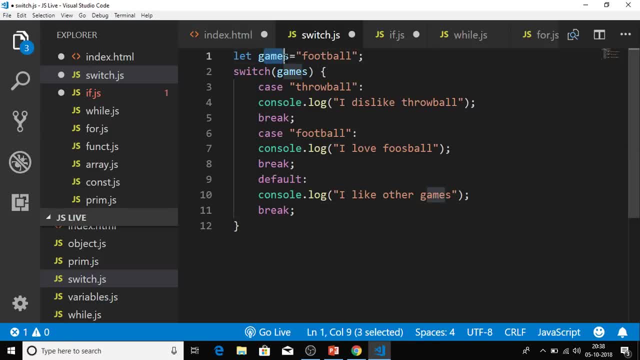 so what i did here was i basically um, declared a variable called games, i set its value to football. then i pass this games variable to the switch statement. okay, so i pass games as an expression to the switch statement. then we have two cases here and one default statement. the first 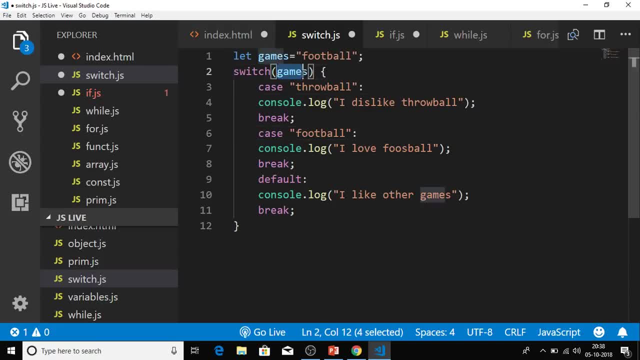 case is throw ball. second is football. now, if the value of games matches with any of these values- football and throw ball- then that respective code block will get executed. okay. and in case the value of games does not match with any of these two cases, then the third default. 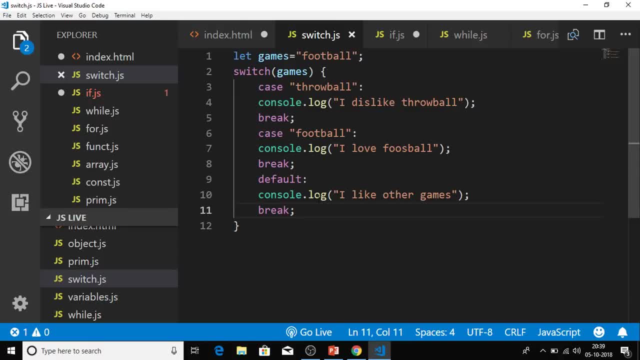 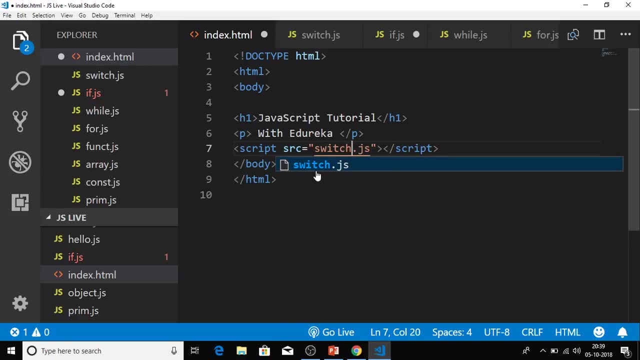 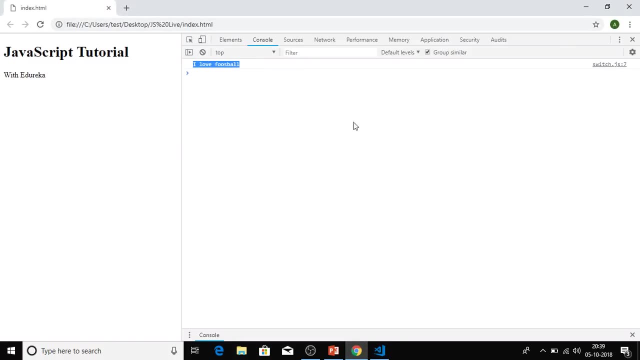 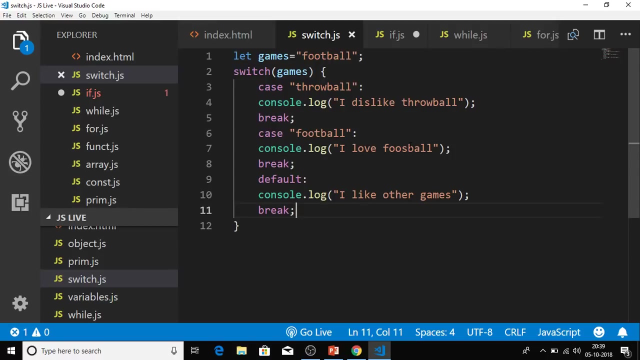 statement will get executed. okay, now let's save this and let's pass the reference of this file so it is switchjs. save this and open up your term. your browser refresh, so you get: i love foosball. so you get. i love foosball because, um sorry, football. oh, here i've written foosball. sorry, i meant to. 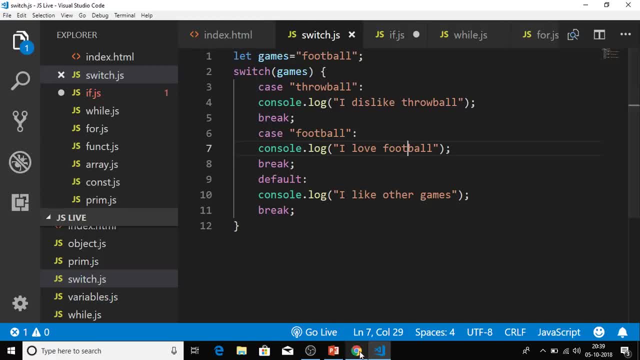 write football. okay, so let's just try that again. okay, so i love football. now, the reason this got displayed was because the value of games is football and the value of this case is also football, so the respective code within this case gets executed, all right. so, guys, that's how switch cases work, okay, um. 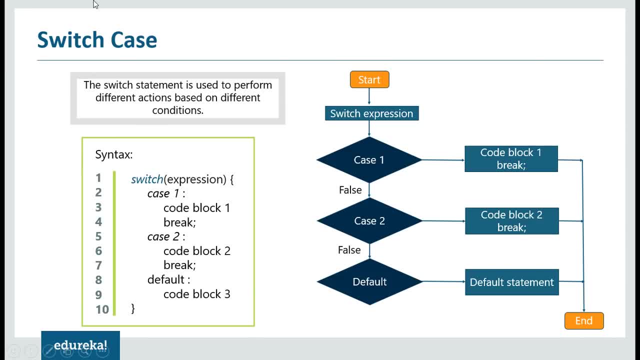 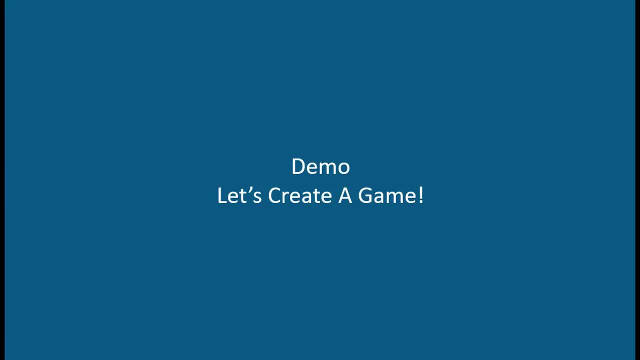 okay, uh, now going back to our session now. uh, now let's build a guessing game. okay, so we're going to build a guessing game using javascript. so now that you have a basic idea of all these fundamentals like variables, constraints, you can build a guessing game now. so, along with a javascript, we'll be using html and css to build. 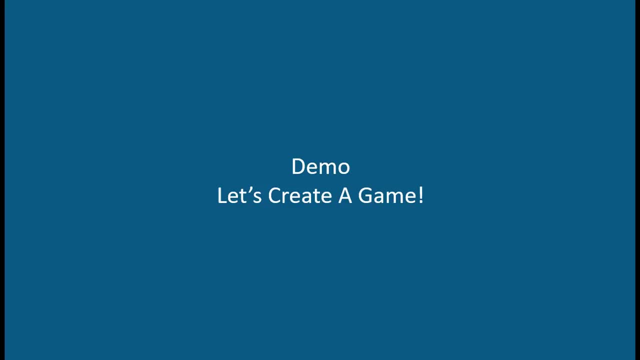 this game. okay, now, discussing html and css is sort of out of scope for today's live session, but i'll leave a copy of this code for all of you that you, all of you who want to run it. okay, so we're going to create a color guessing game. 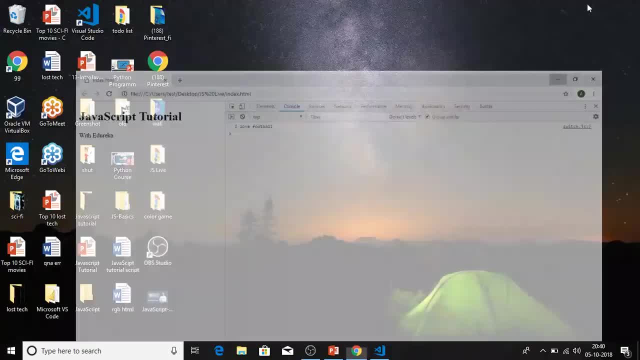 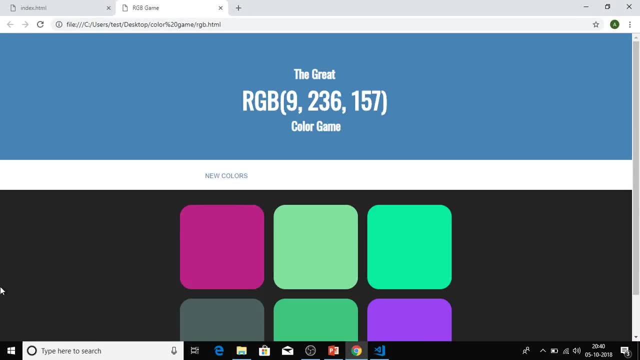 let me show you how it looks. so okay, so this is how the game looks. um, now all you have to do is guess the color based on this rgb value. okay, so you have to guess the color of these squares based on this rgb value. so, for example, over here, you can see that the value of blue, which is 157, is quite high. so you can guess. 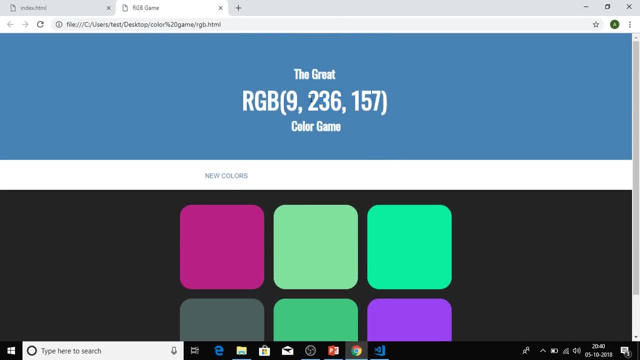 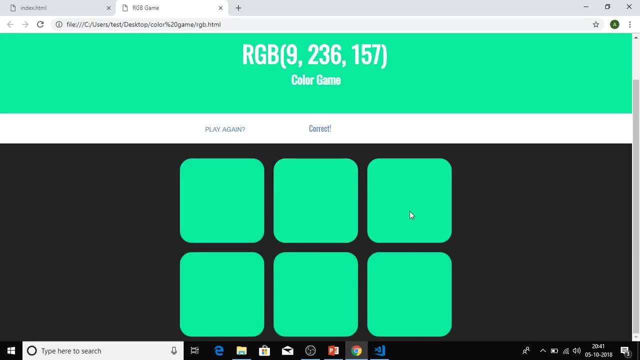 no, sorry, here it's 157, so you can guess. no, sorry, here it's 157, so you can guess. no, sorry, here it's green. yeah, so the value of green here is very high compared to red and blue, so you can guess that the color here will have more of green. so let's try. yeah, so i get, i guess, the correct block. 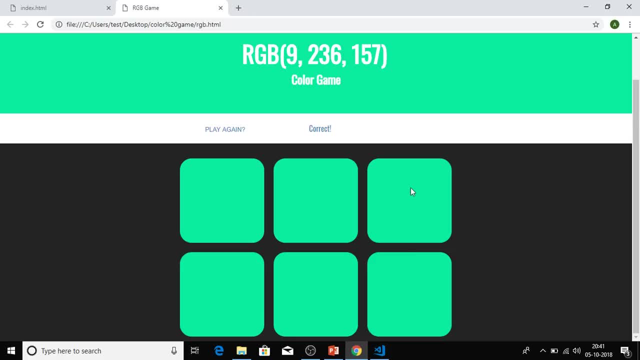 so all of these six squares turn to the winning color. winning color: okay. similarly, the header also turned to the winning color. okay, you can again. we can play again and you know, you can choose and you can even change colors over here. so this is the game. now let's look at how. 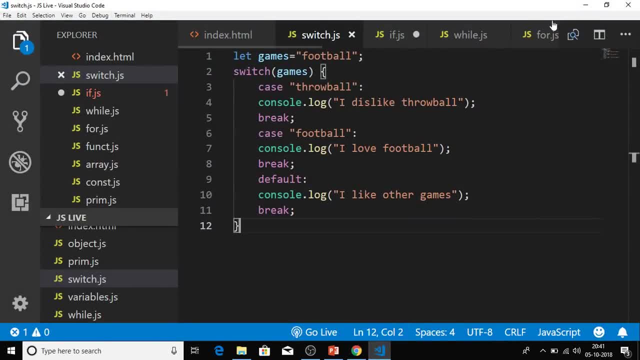 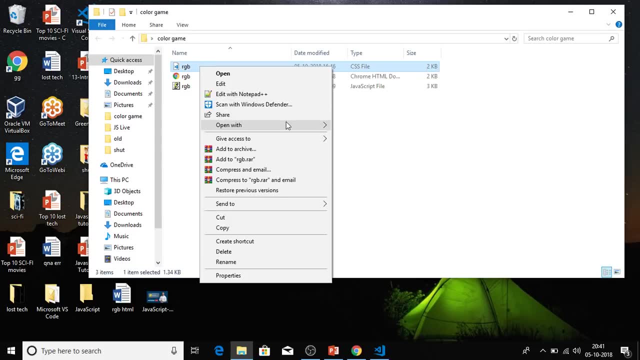 this is how we created this game, okay, so i'm going to open up the code. so, guys, i've already typed out the code over here, because it'll take a lot of time for me to type this code on the on this session, so i'm just going. 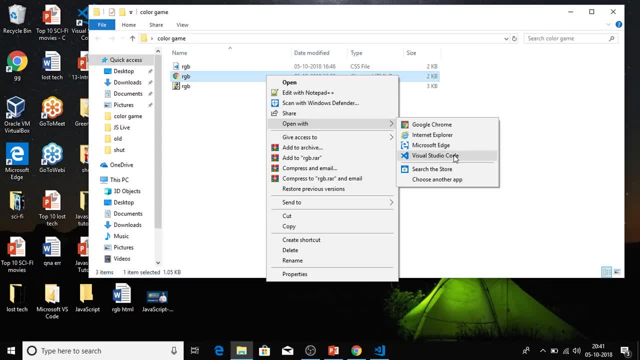 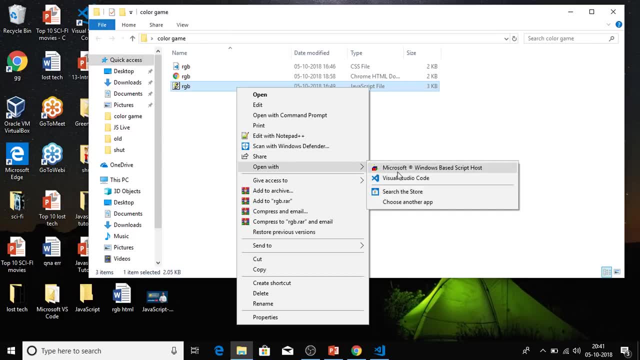 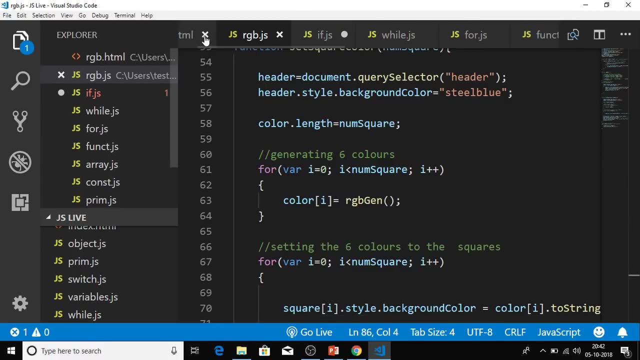 to open up the javascript code. i'm going to open up the html code as well as the css code, okay, so i'll just close the other one second. guys, just bear with me, let me shut everything, otherwise you guys might get confused, okay. okay, i forgot to open the css file, okay. 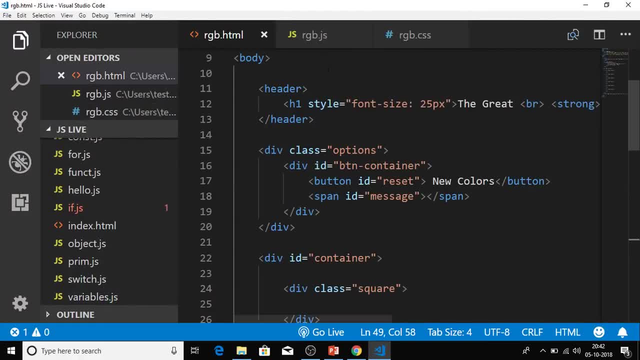 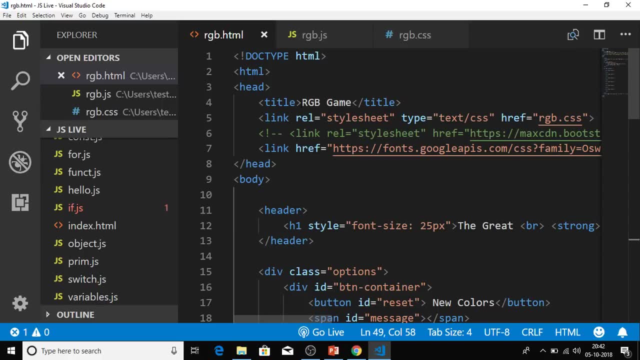 okay, okay, okay. so now we're ready to load the css file in our code. we're going to load it into. so now i have the html file for this game. i have the javascript and the css file. now i am not going to go in depth about html and css, but let me briefly tell you what i will. 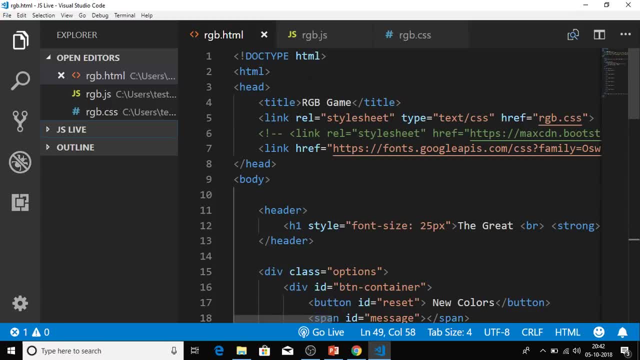 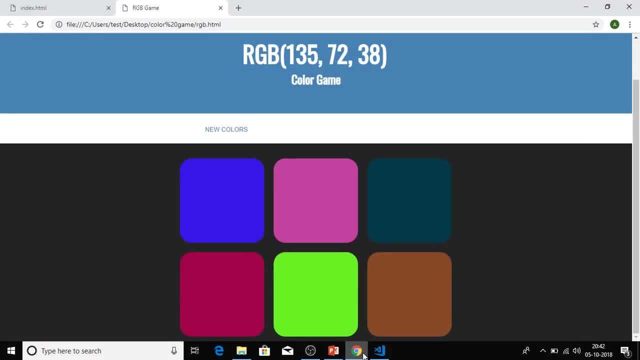 give you a brief idea about what's happening over here. ok, so basically, first we have a html file. now, within the header, we have a title for our game, which is rgb game. now, this is basically the title. here you can see: rgb game. ok, then we have a reference, we have a 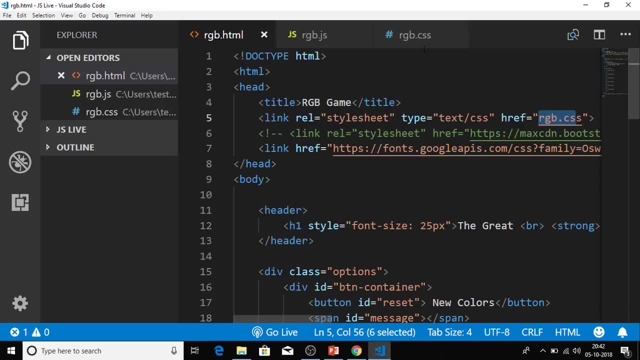 link to the css file. rgbcss is the file, so we have a reference to this file from our html file. then we also have a reference to a font- ok, so you can down load different kind of fonts from google. so this is basically a link to the font. so i have designed my webpage. 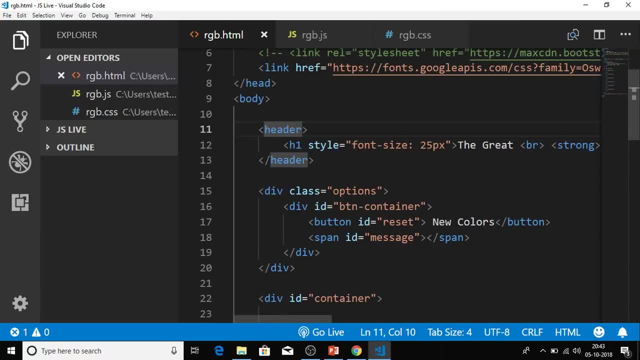 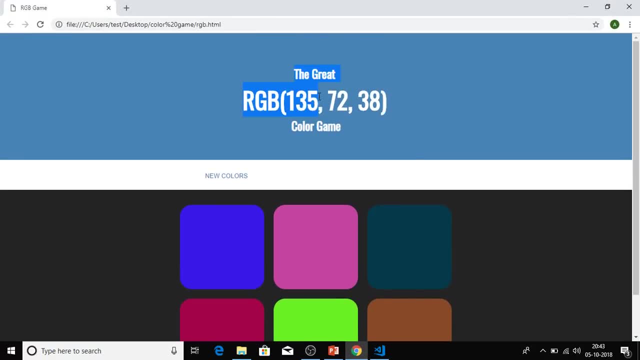 with these fonts. then within the body, we have a header. now let me show you how the header looks now. this is the header basically. now in that line of code we are basically printing this: the great rgb game 2. we have a header and here you can see, we have a link to the 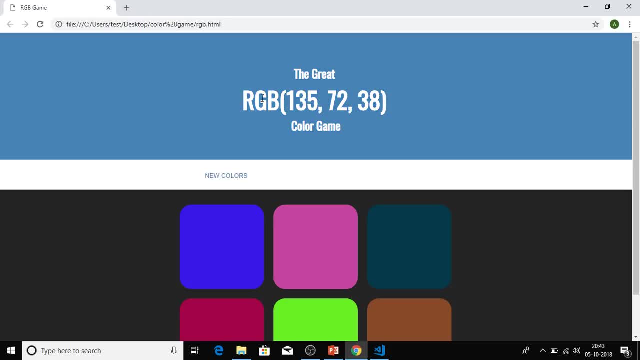 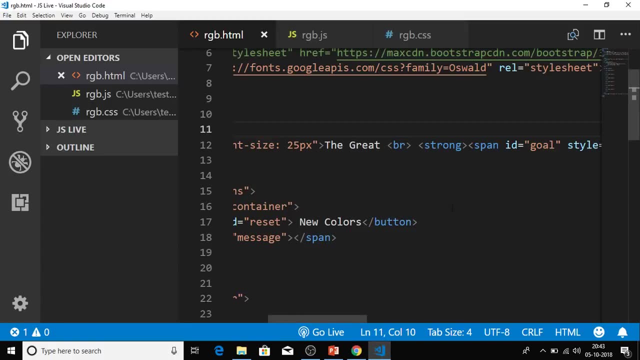 code inside the code. here we have a handle again- and we have a reference here for this- with the values and color game. now this is basically a rgb value is basically randomly generated values. okay, so because it's randomly generated values, we have passed this in a span. 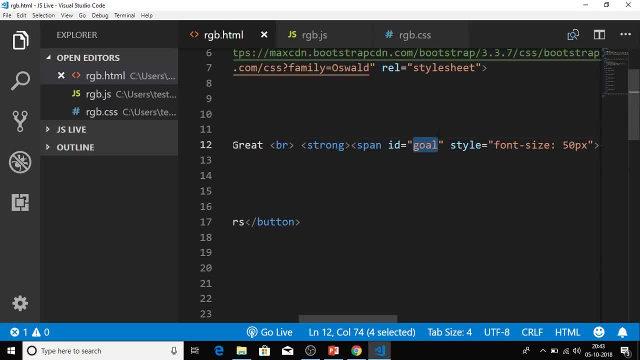 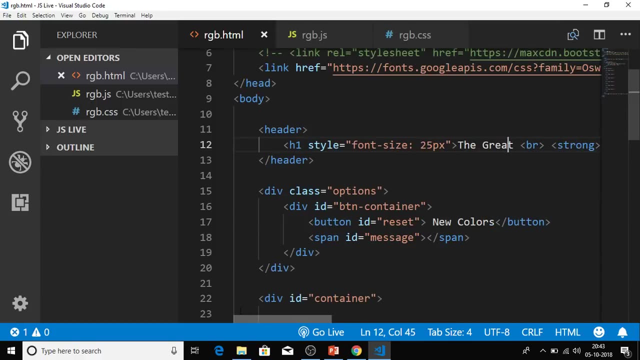 okay, we've the. basically, the rgb value is stored in this variable called goal. okay, now we have defined a span for this, because this rgb value keeps changing. okay, apart from that, it's going to print the great um color game. okay, so that's what this line does. then we have different. 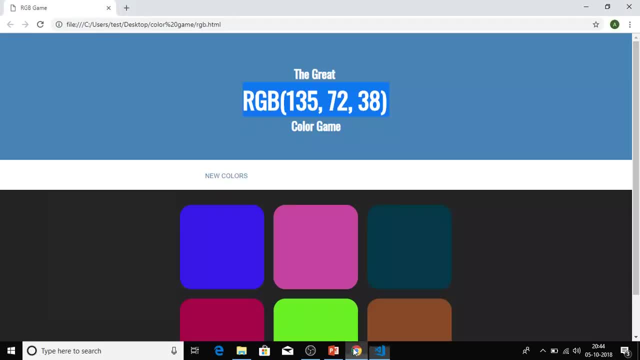 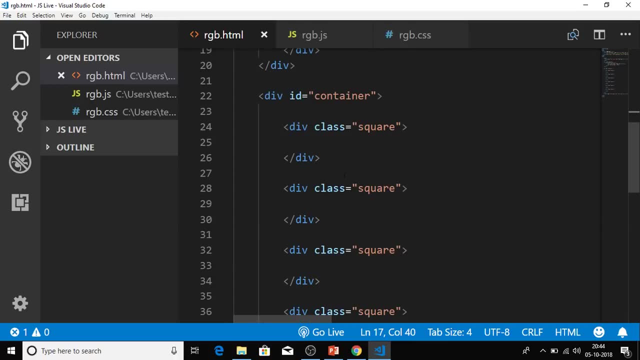 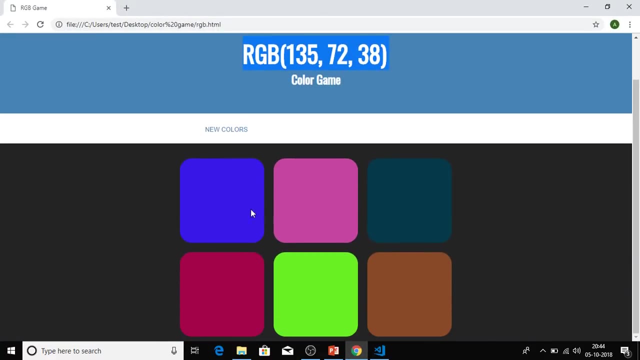 divisions. so we have button. we have a button called new color. you guys can see it over here: new colors and then, um, now moving on to divisions. so we have six different, six different divisions here and each division has a class called square. okay, so, because we have six different, uh, boxes. 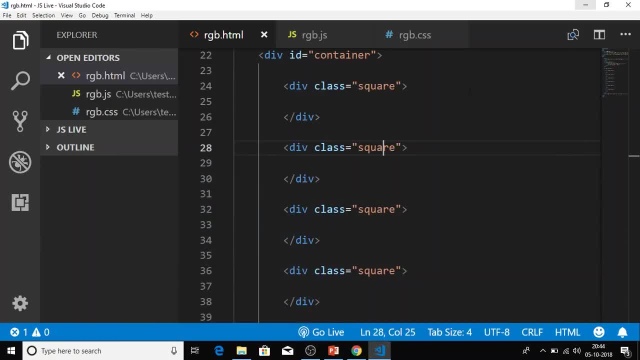 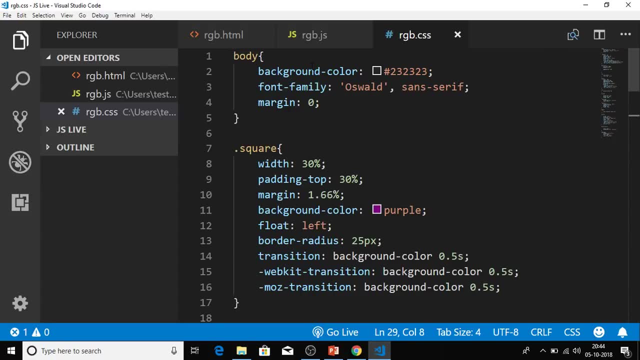 here six different squares. i've defined six functions called square. okay, now, moving on to the css file. now, basically, i have designed the body, and for the body i've used this background color, it has a particular font, and so on. okay, and each of these squares have: 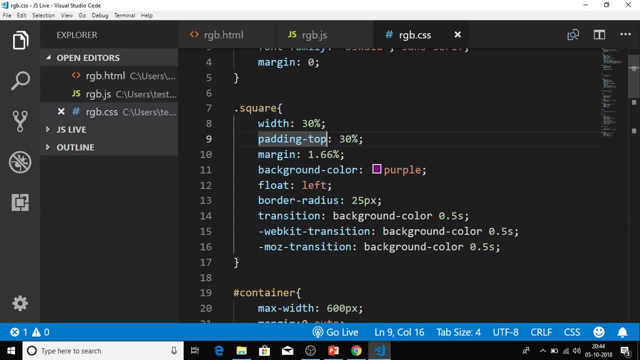 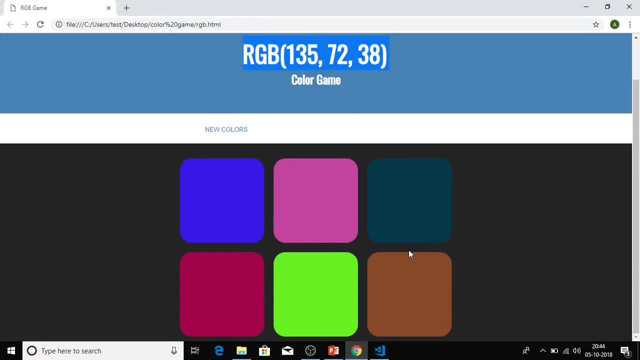 set of properties like the width of the square, the padding, the border, the background color. all of this is set over here. okay, so you can see that the, the width, the shape of these squares, all of this is defined in the css file. okay, so basically, the color, the design is done in the css file, that is. 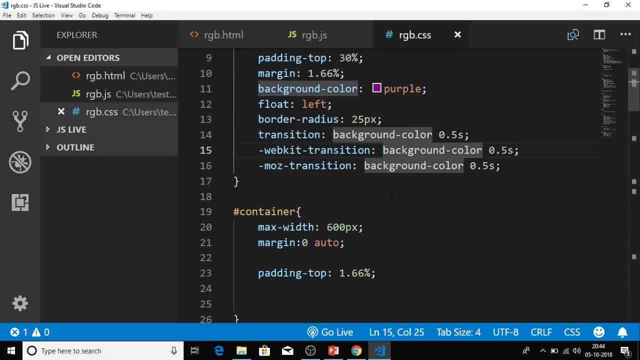 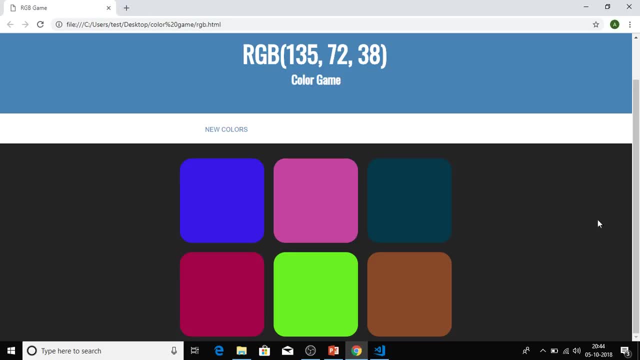 the css file, and then we have the css file, and then we have the css file, and then we have the purpose of css. it is for styling purpose, okay. similarly, this container i've defined, this is basically the container. you can see the black border over here. this is the container, okay. 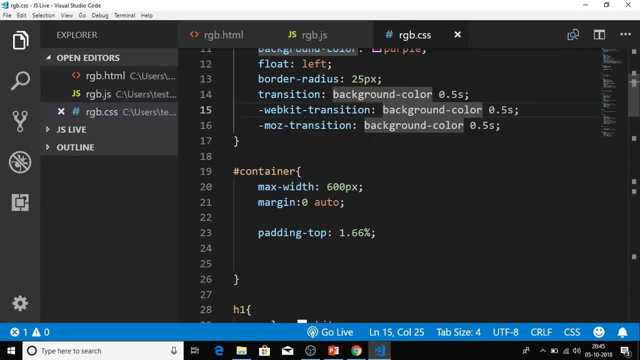 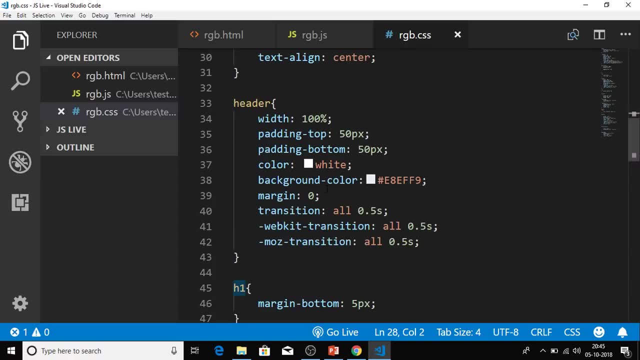 this container has all of these six um um squares. okay, uh, then we have a header for the for printing the rgb game, and similarly, headers i've given a lot of. uh, what do you call? i've given a few properties for the header, like it should be, of this color. 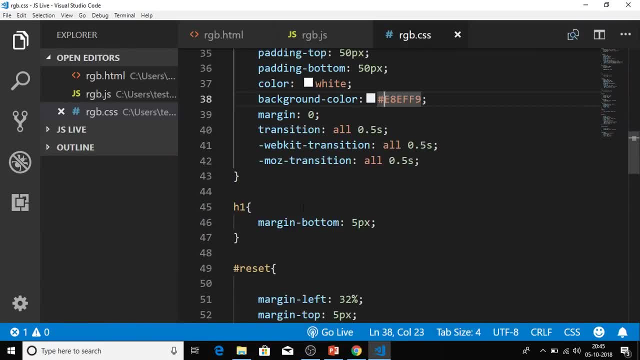 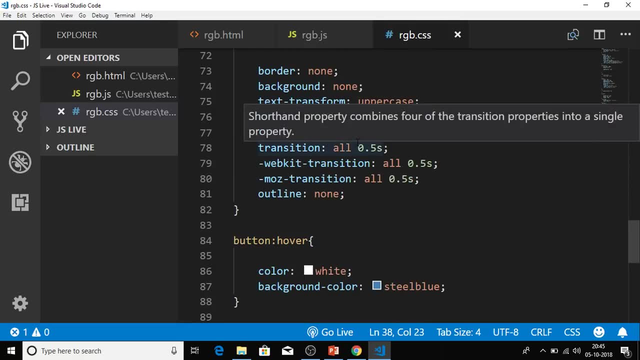 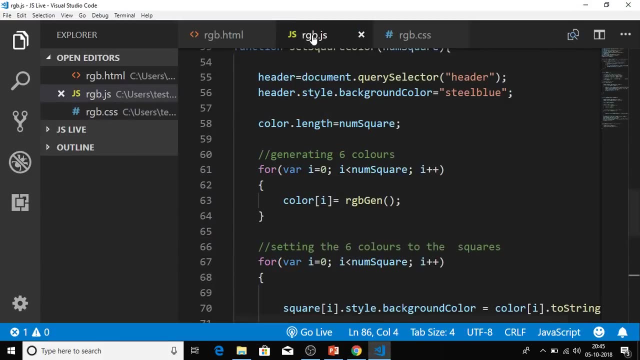 so this is basically the header, okay, and similarly there are other. every other thing is styled using the RGB CSS file. okay, so within the CSS, I'm going to style everything. anything that you can see here, any color pop or any sort of styling, is because of the CSS file. now let's focus on the JavaScript file. now. 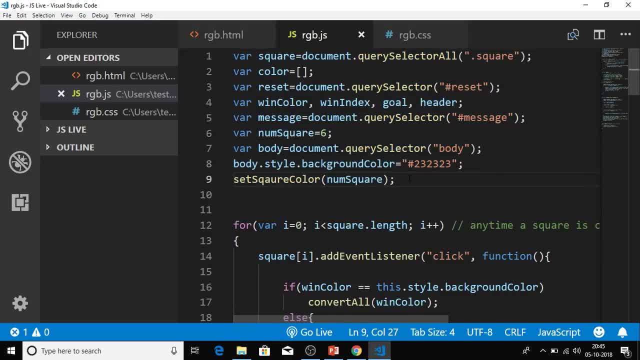 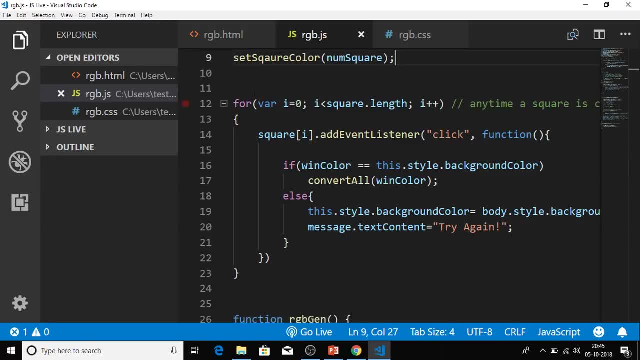 these are variable declarations, so I'll get back to this at the end. now let's look at the functions and the for loops that are used in this JavaScript file. okay, now, the first for loop is used any time a square is clicked. this: what happened? this is what happens, so let me show you what we're doing here. so now, 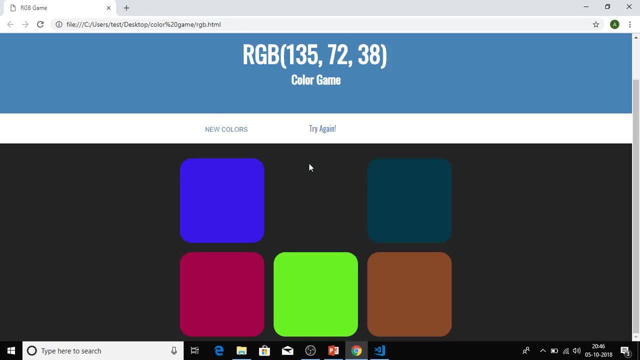 every time I click a square. so if I lose, then this the color of the square is turns into the background color, turns into black. basically, now, if I, for example, if I win the game, let's say: okay, it has more of red, yeah, so if I win the game on clicking the square, all the other squares are also. 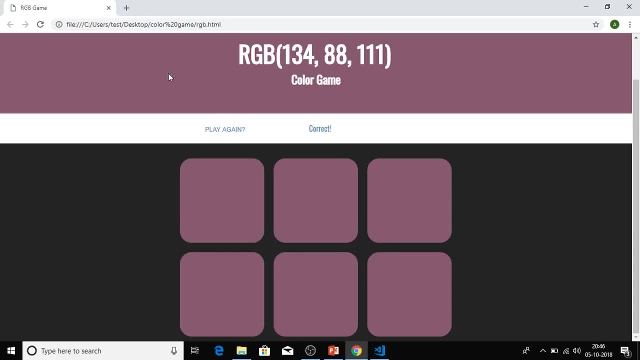 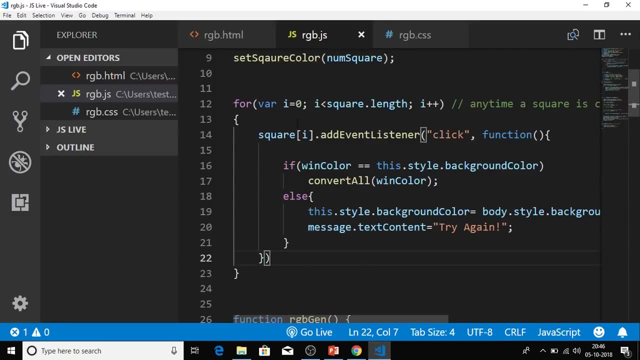 going to turn into the winning color, okay. similarly, even this header is going to turn into the winning color and a message called correct is going to be displayed. now, how do you do this through code? so this is what is explained over here. okay, so I'm going to define a for loop within this. I'm starting it with: I. 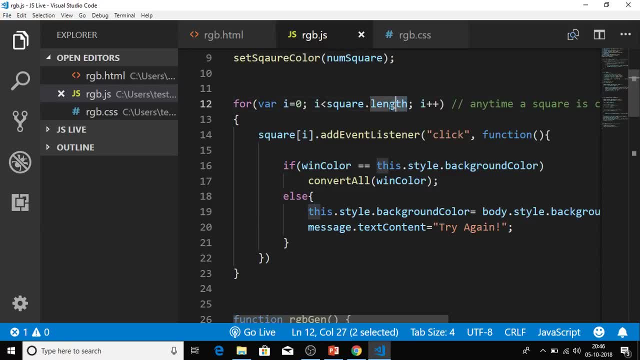 equal to zero. I is less than square dot length. now this function, this will basically calculate the number of squares. okay, so square is stored like an array. it's sort of stored like an array and you're just going to calculate the length of this array. okay, it's something like this. so the length of 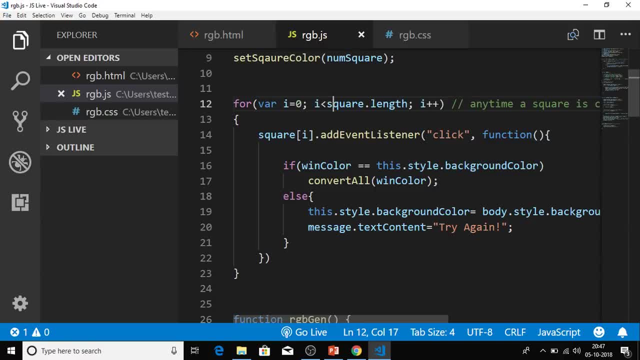 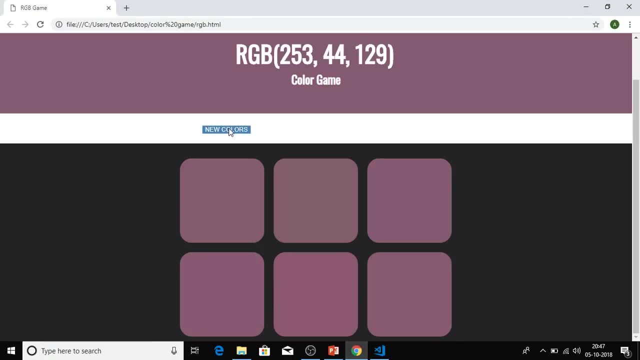 this is six. so this is basically: I is less than six, and then I'm going to increment the value of I. now what happens is, every time you click on a particular button or you click on a particular square, some event occurs. okay, now you need to add event less listeners, which listen to all of these events. so 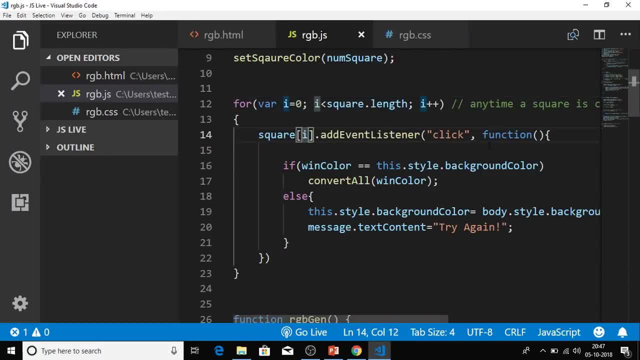 for that. I've added event listeners here. now, every time a square is added to the square is clicked. you can see click. every time a square is clicked, this function is carried out. okay, this function is run now. this function has an effects loop. now, within the if loop, I've defined a condition. this is the. 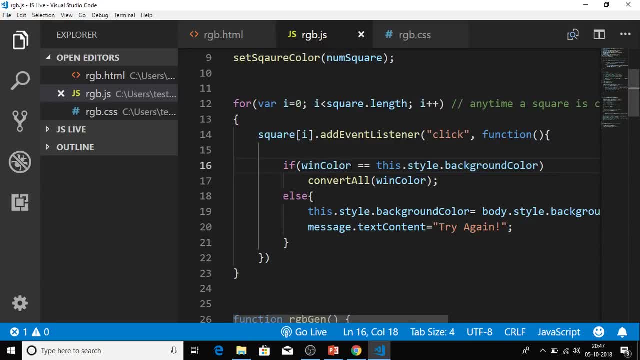 condition now, when color is basically stores the value of the, the RGB value of the winning color, okay. so, whichever color is, correct that that colors value is stored in this wind color variable. okay, now, if this value of this variable is equal to this, now what is this? dot style, dot background. 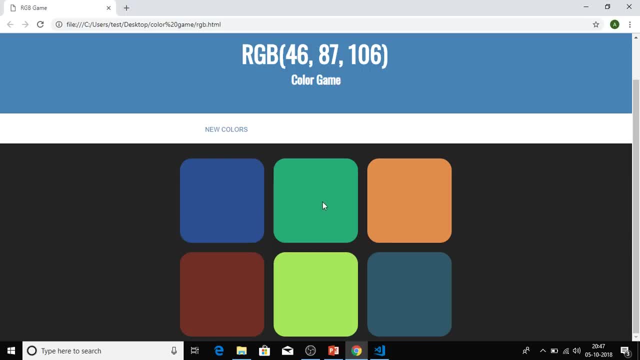 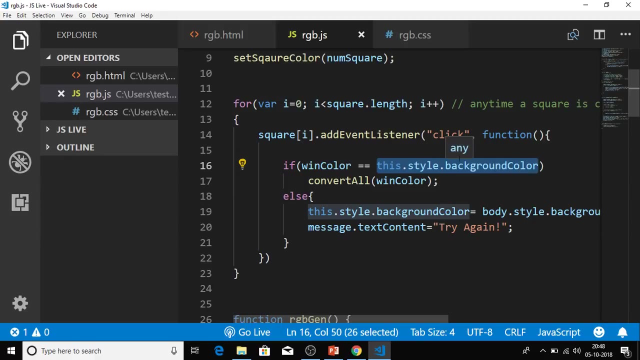 stand for. let me show you what it stands for. so now, every time I click the square, so if I'm clicking this square, basically the RGB value of that square is stored in this, alright, so basically the color of the square that I clicked on is stored in this. so you're going to compare that color to the winning color. 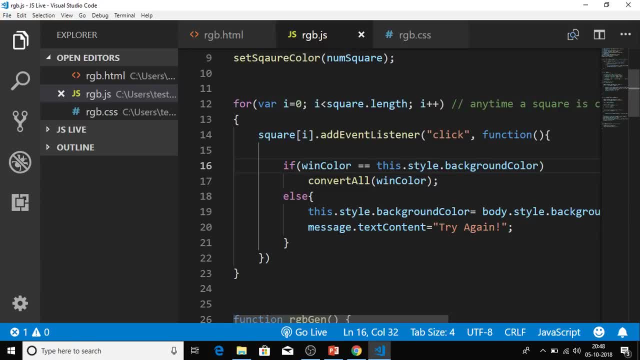 now, if this is equal, I mean, if it's not true, then you're going to run this function. so you're calling a function called convert all with this parameter. okay, now let's look at where this function is: convert all, yeah, so what happens over here is: first, you're. 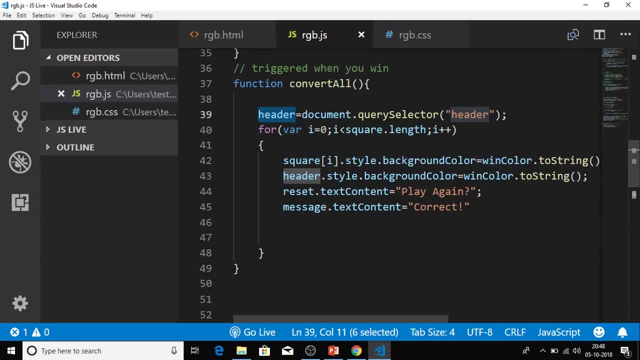 selecting the header, and then there is a for loop. I'll get back to this now. what happens in this for loop? we have the same condition: I is equal to 0, I is less than 6, I plus plus. so what I'm doing is I'm selecting all the squares and I'm 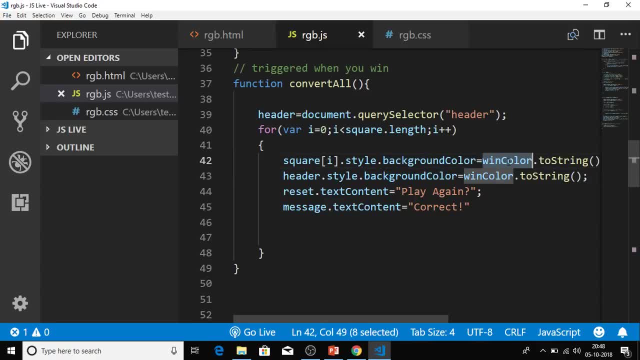 basically changing the background color to the winning color. okay, so I selected all the squares, I changed their color into the winning color. similarly, the headers background color is also changed to the winning color, because here you can see that if I win this game, okay, so in this I'm 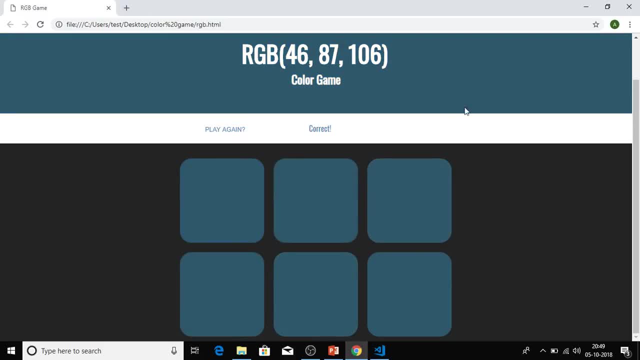 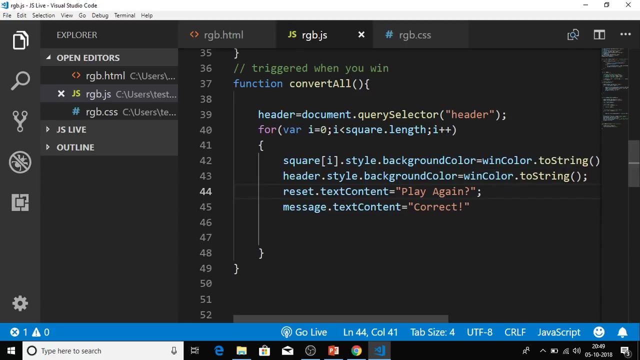 expecting more of blue. so, yeah, as soon as I won the game, the headers color, as well as these six boxes, also change and this message got printed: okay, correct, and also play again. new colors got changed to play again. okay, these few things happen, so that's what I'm doing here and then. 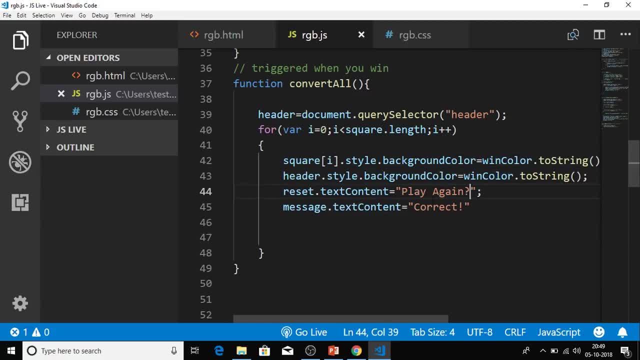 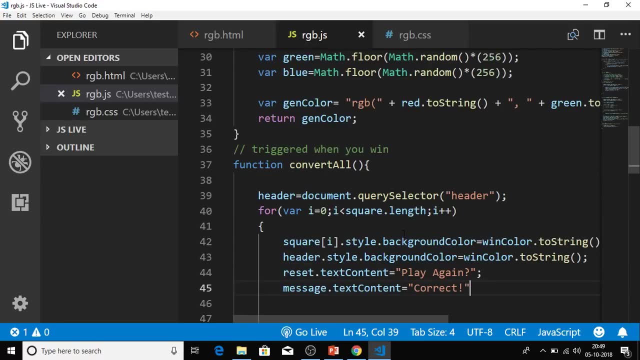 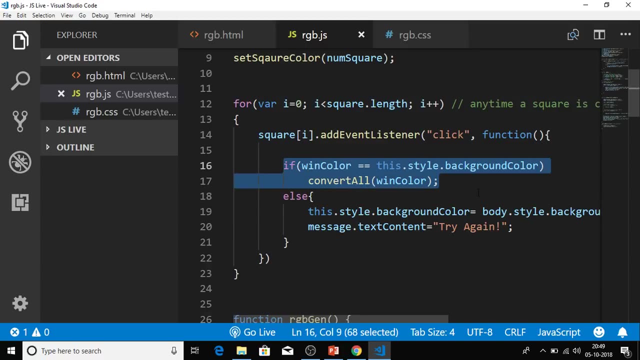 see exactly what I said. I'm going to reset this to play again. the button is reset to play again, and then a message called correct is printed on the screen. okay, so I hope you all are clear with this function now. after after this is executed. so basically, this: if condition will get executed. if, though, if you've 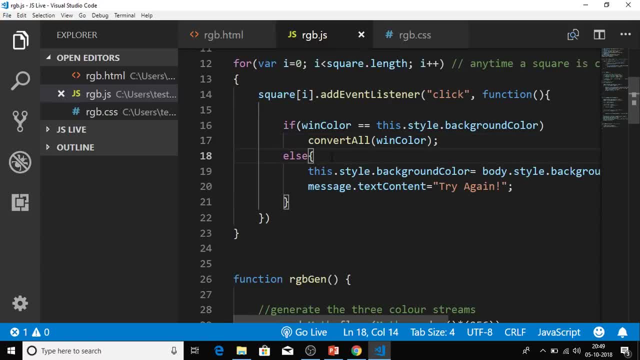 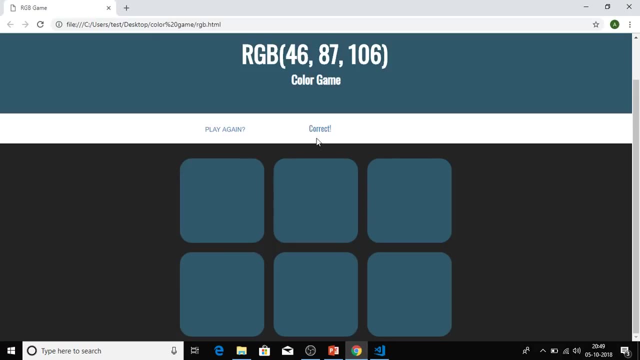 won. now, if you weren't able to guess the value of, if you weren't able to guess the color of the square, this condition will get executed. so, basically, the box that you clicked on, the background color of that box is set to the color of the body. okay, so basically, let's let me tell you what's happening over here, okay. 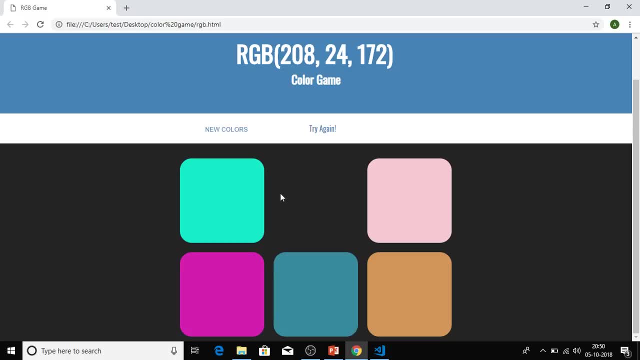 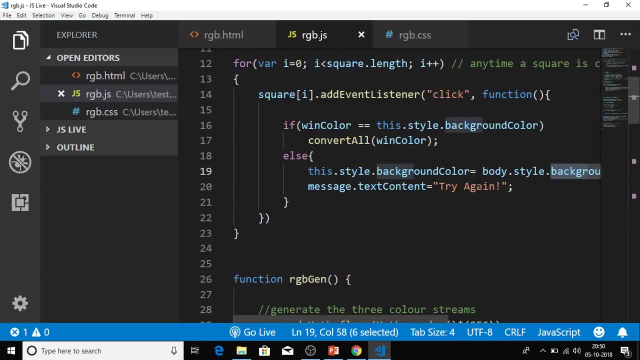 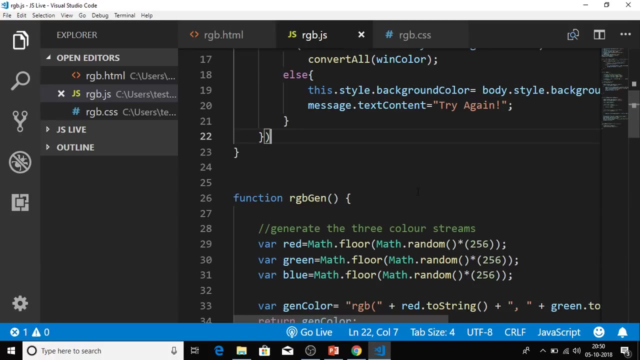 so this was a wrong answer. so what happened is, the color of this box was set to the background color of this page, so that is black. okay, that's exactly what's happening in this line of code, okay, and also this message is getting printed, which is: try again. so that was about this function. next, we 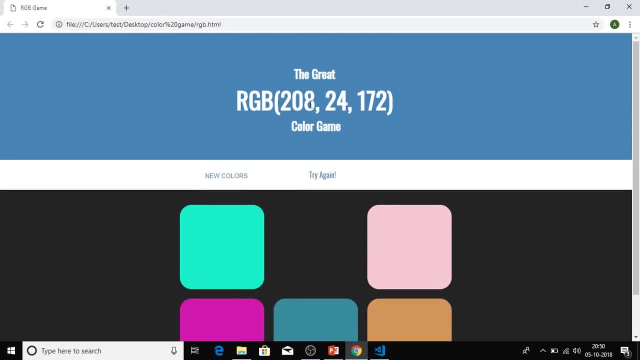 have the RGB generators now. here you can see a few RGB values. all right, you can see values 208- 24. this stands for the red value, green value and the blue value. now, every time we click on new colors, new string is generated, new stream of RGB values is generated now in order to generate these. 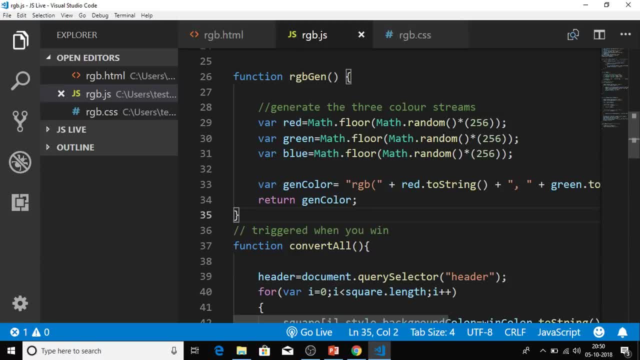 colors. you use this function. okay, this function. now, what happens is there are three variables here. there's red, green and blue. now, how we generate these values is we use a function called math dot- random. okay, now what this function will do is it will, basically, it will return. 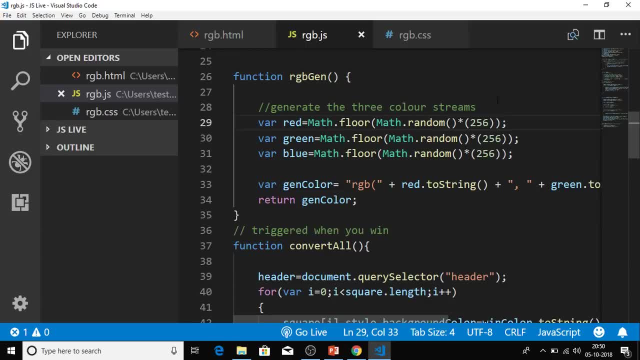 decimal points between 0 and 1. okay, so it might return something such as 0.25, 0.13, 0.23, something like that. okay, it will just return values between decimal values between 0 and 1. okay, now these values are multiplied with 256. now we are multiplying it with 256 because there are 255. 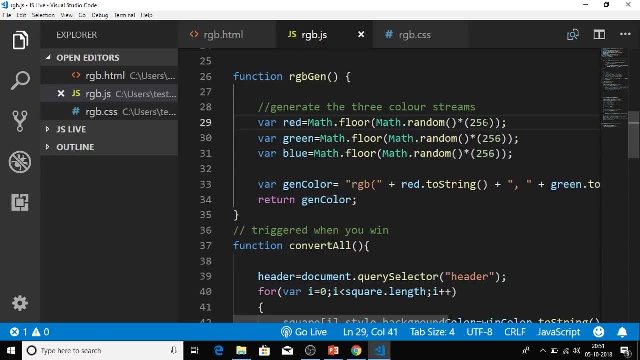 256 values of colors, so from 0 to 255. okay, so these are. this is basically the range of colors. so you're going to multiply this randomly generated decimal point with this integer. when you do that, you'll get a decimal. now, the computer will not be able to understand a decimal. that's why you use math. 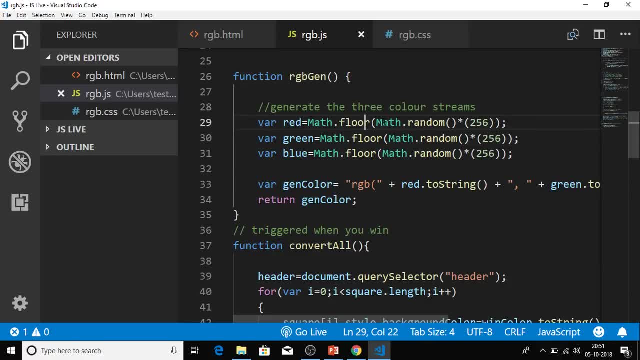 dot floor. okay, now, this math dot floor will basically round off this decimal point. okay, so that's how the value of red, green and blue is generated. okay, now this: you're just going to add these values into strings and then you're going to return the generated colors. okay, 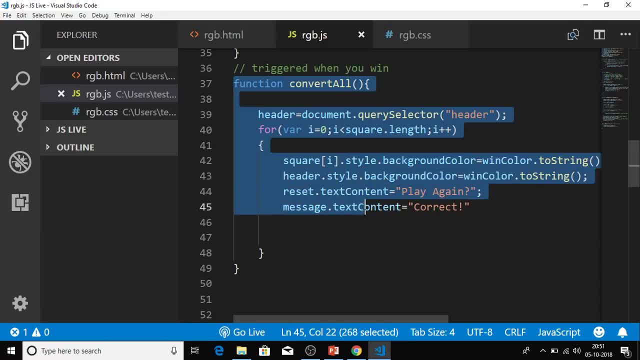 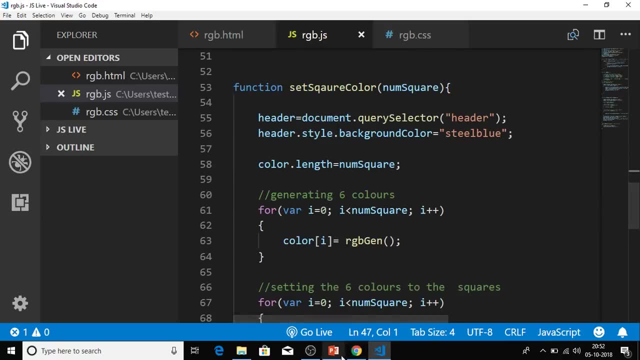 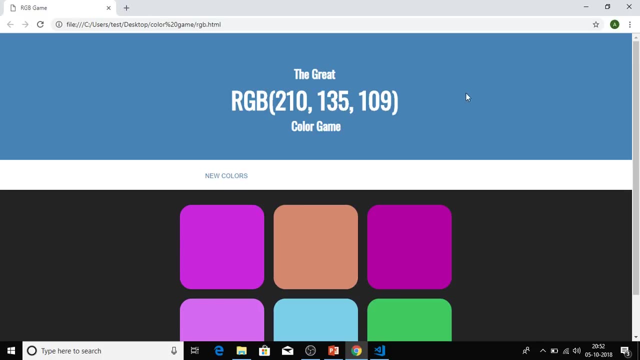 now this next function. i spoke about convert all. i already explained this function to y'all. now, moving further, we have set square function. now one thing i forgot to tell y'all is so whenever you open the game, the header is always set to blue, is always set to a color called. 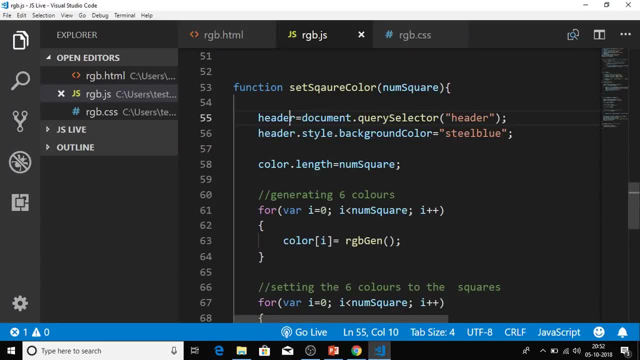 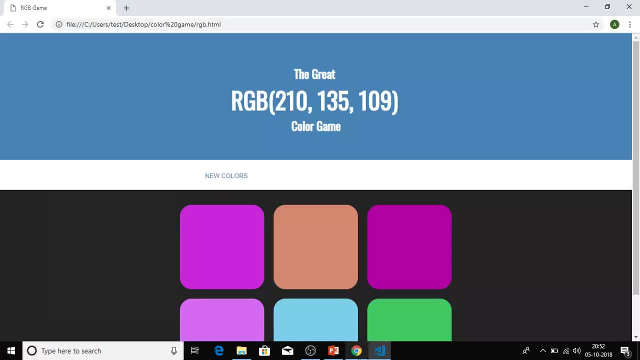 steel blue. okay, so that's what i'm doing here: i'm selecting the header and then i'm setting the background color of this header to steel blue. okay now, um, when you open the page, you see that these six squares have six different colors. now, how do you generate these colors? now, this for loop. 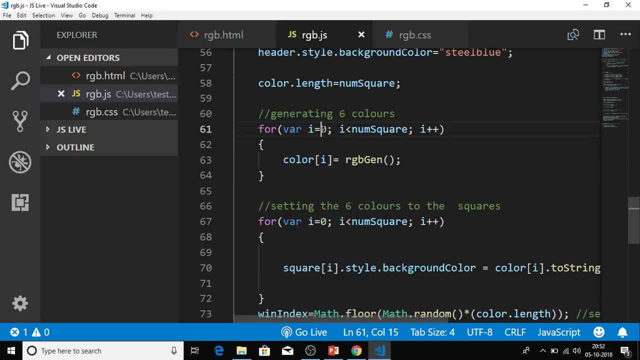 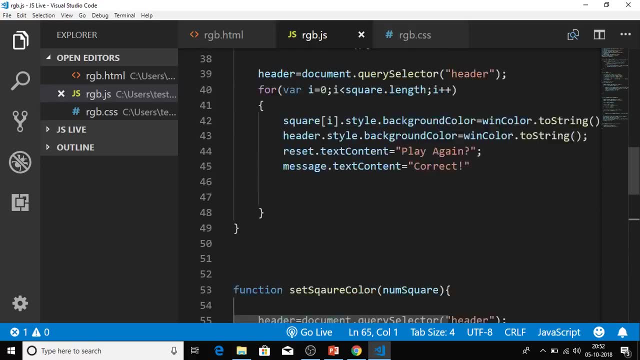 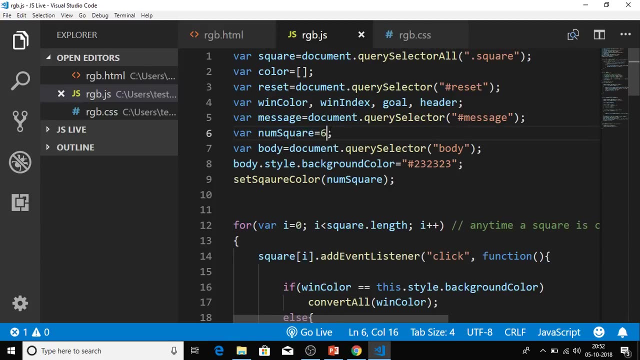 is used to generate these colors. okay, now this for loop starts from: i equal to zero, i less than num square, and you're incrementing the value of i now the value of i. i had declared it in the beginning of the program. okay, so i've set the value of i- uh sorry, the value of num square to six. 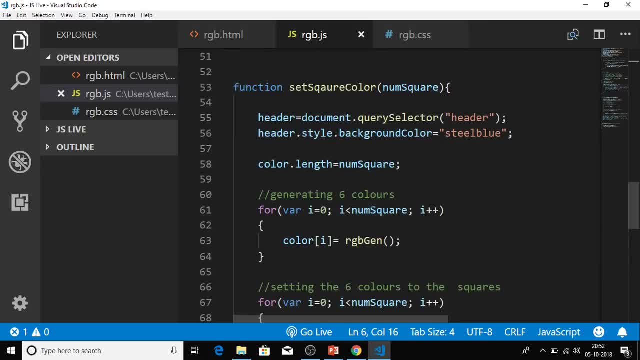 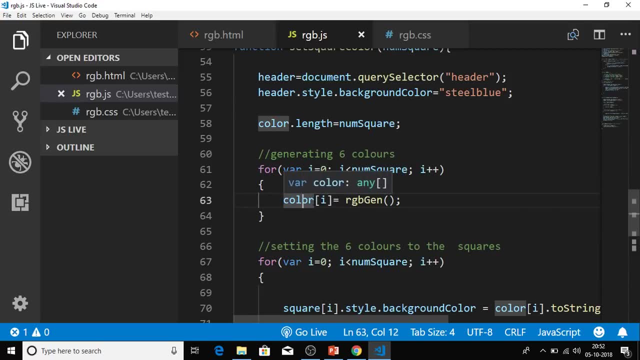 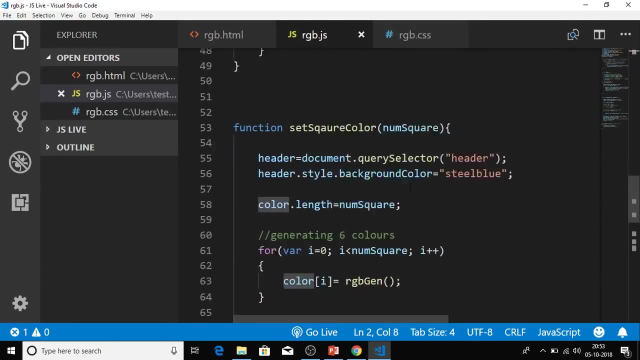 so basically, over here, um, yeah, so this is basically. i is less than six. okay, so what you're going to do is, within this color array, which also is declared, uh, in the beginning, yeah, here's the color array. um, within this color array, i'm going to generate six different colors. how i'm going to. 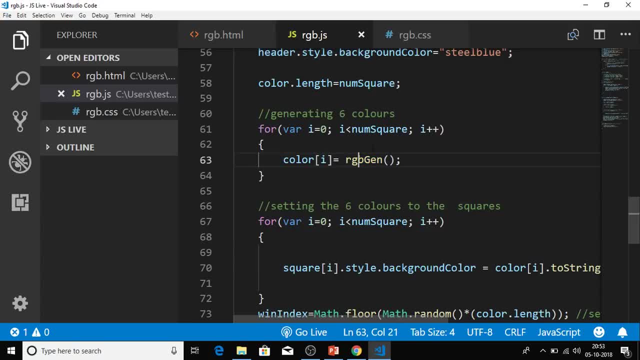 do that is by passing this to the um rgb generator function. now, i told you that this rgb generator function randomly generates- uh, different rgb values. okay, so basically, i'm going to get at the end of this for loop. i'm going to get six colors generated by this rgb generator function. 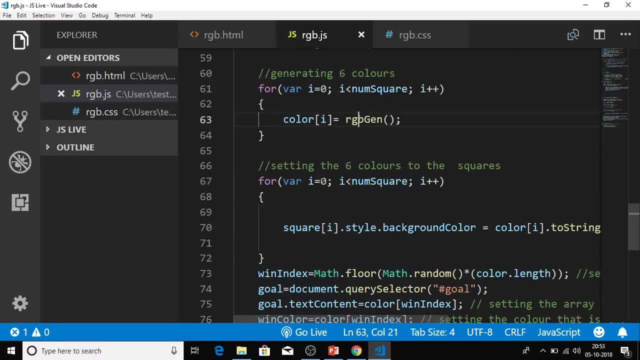 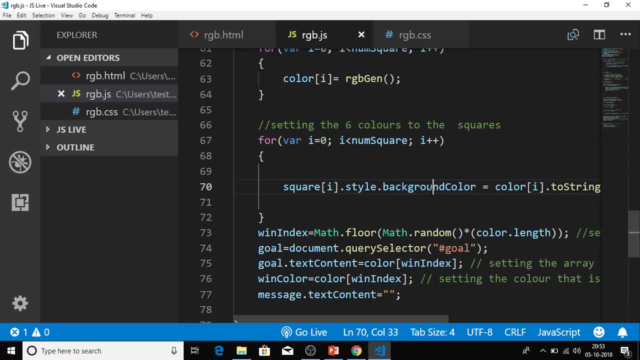 now you need to set these six colors to the squares. for that you're going to run this for loop. okay, now, in this for loop, basically, i'm selecting every square and i'm setting the background color to the array of colors that i just generated. okay, this is as simple as that, guys. this code is very. 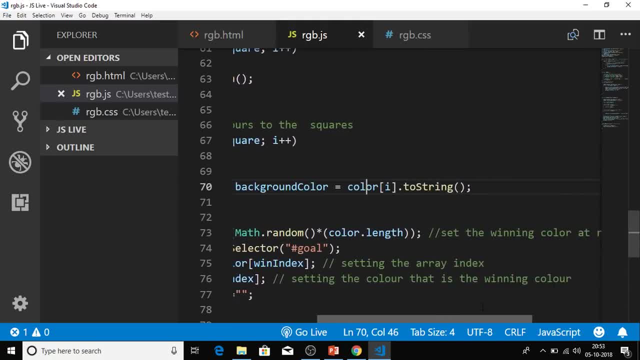 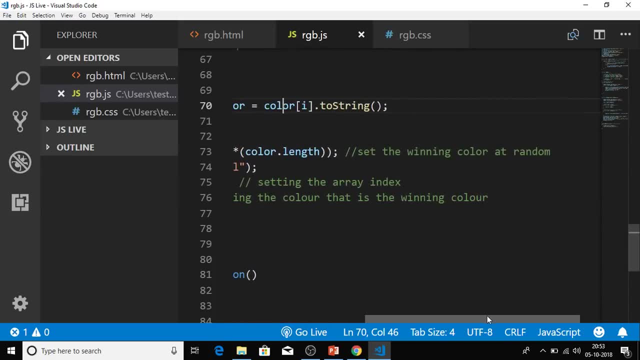 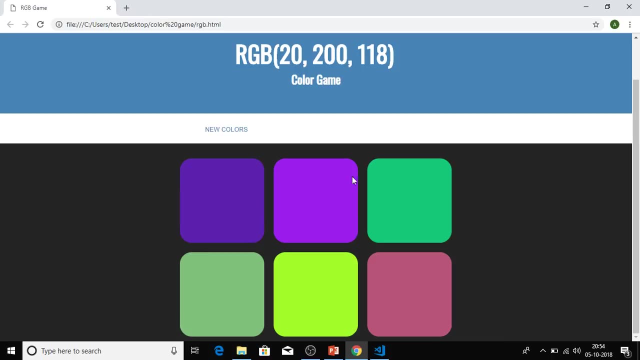 simple it's. if you just read it, it's like you can totally understand what is happening. okay, now the next. what i'm going to do is: um, we also need to set the winning color at random. we can't just randomly have the winning color to be this every time, okay, okay, so that was the fluke, and that. 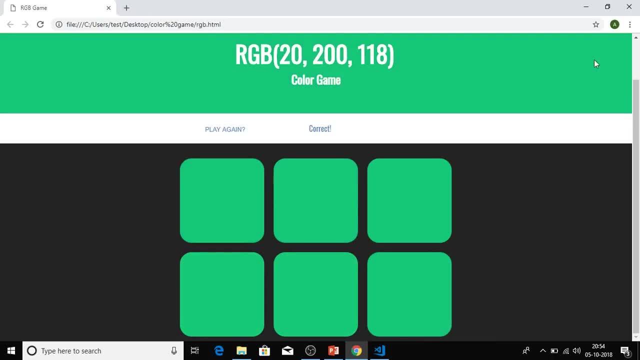 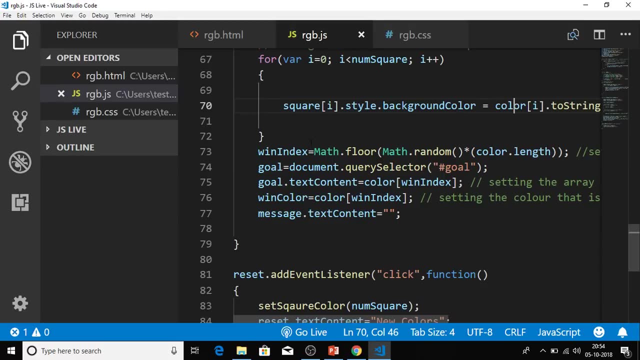 won't happen again. but uh see, we can't have the winning color to be set to one particular square, so we also have to make sure that the winning color is um set at random. so what we do is we do random random generator function, matrandom to generate the winning color, okay, and we store the. 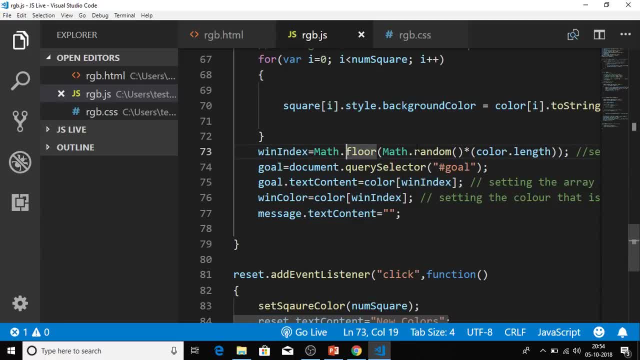 we create a winning index where we store the value of that. okay, now, within this goal is going to be stored the value of the winning color. so you're basically here: you're setting the array index, win index, and then, within this win color variable, you're going to store the value rgb value of the.